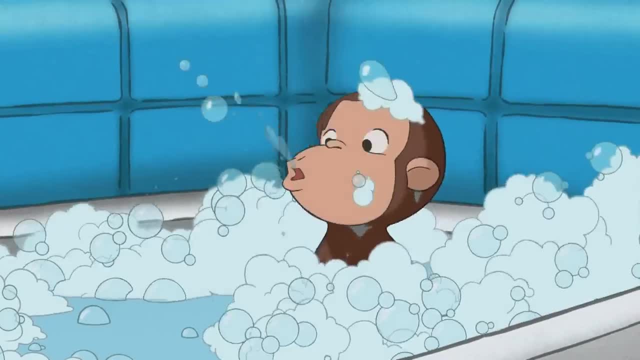 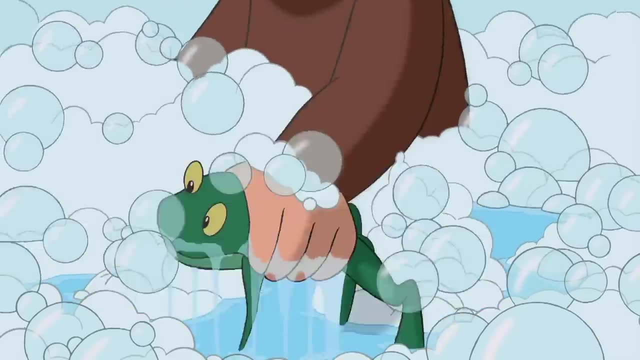 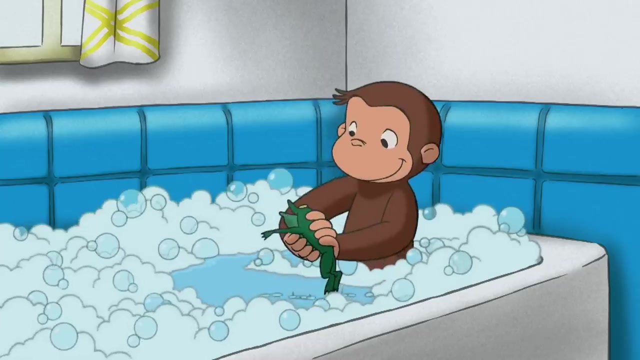 There were only two things that could get George to take a bath: Bubbles and Sproingy, the most awe-inspiring toy frog that ever lived and the best bubble maker George ever met. A bath just wouldn't be a bath without them. 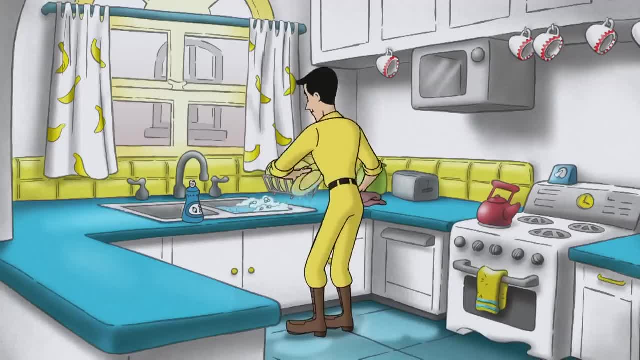 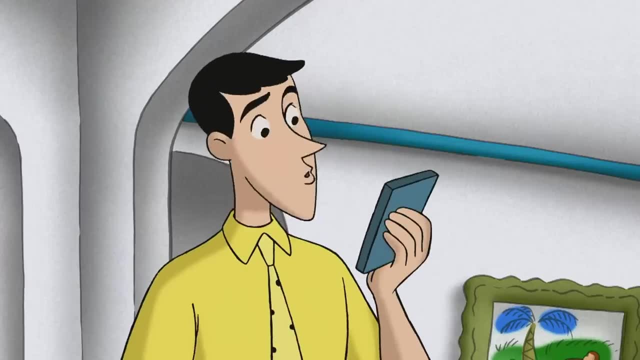 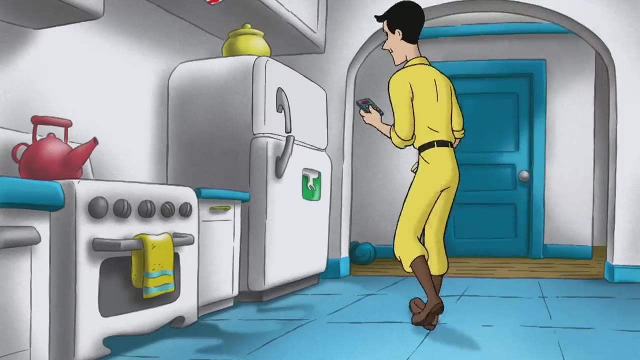 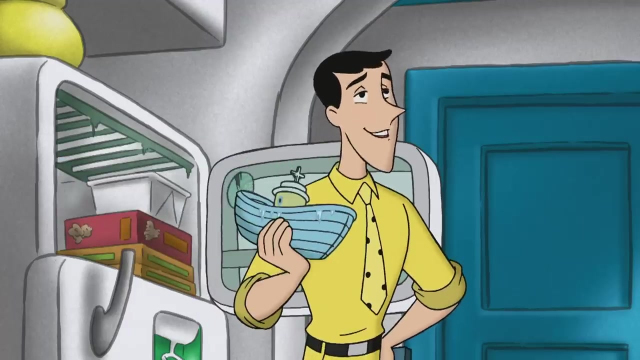 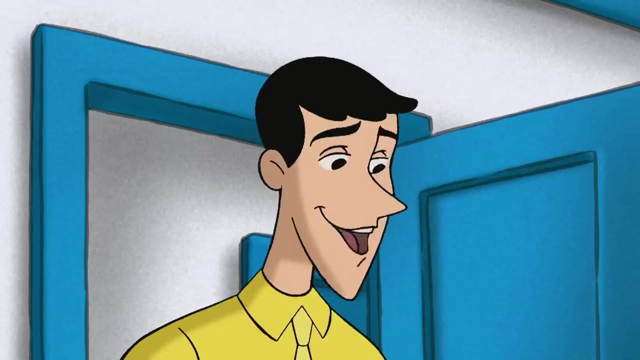 I wonder what this belongs to. Oh, George, I found your lost boat, Woo Ha ha ha, In the freezer. Ah, You know, George, if you were a little more careful with your toys, you wouldn't lose so many of them. 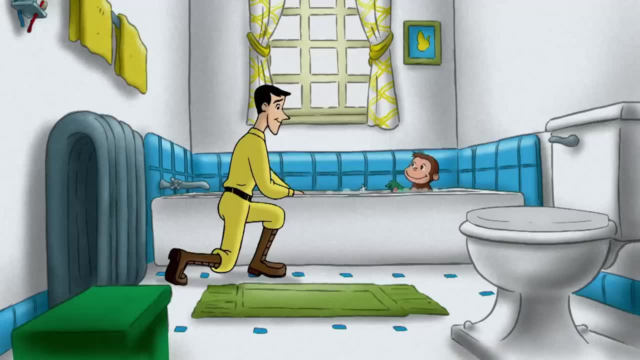 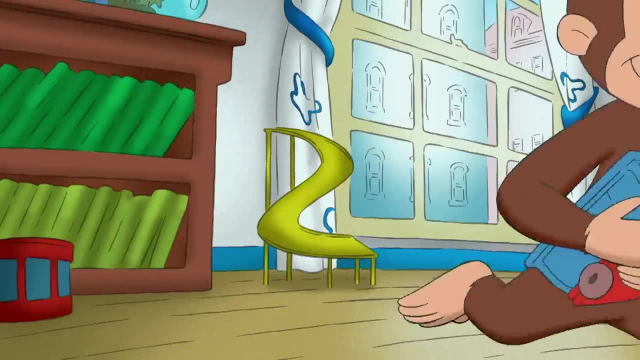 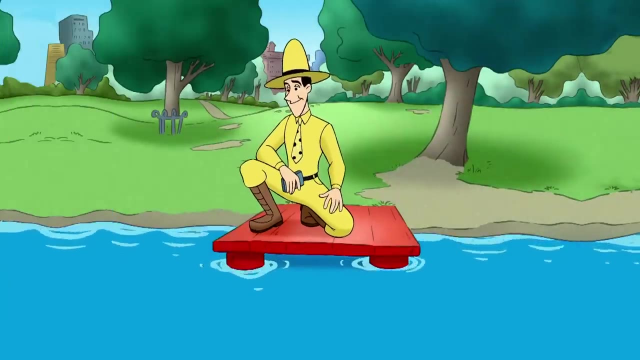 Woo-ha, Woo-ha. You almost ready to go to the park. Ha ha ha, Woo-ha, Woo-ha, Woo-ha, Ah, Hey, aren't you glad we found your boat, George Ge. 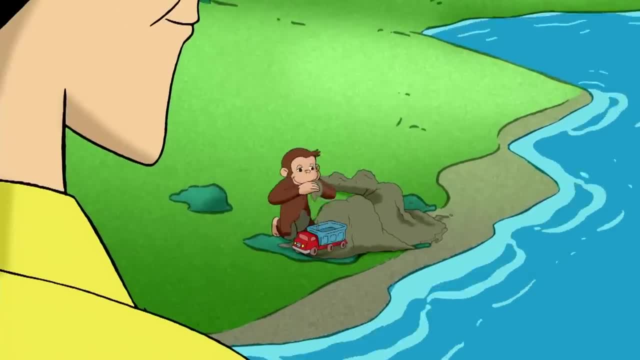 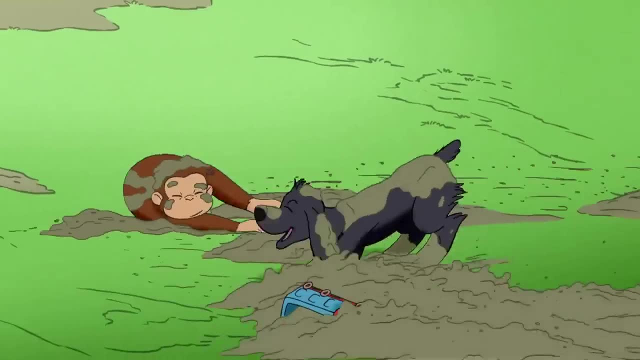 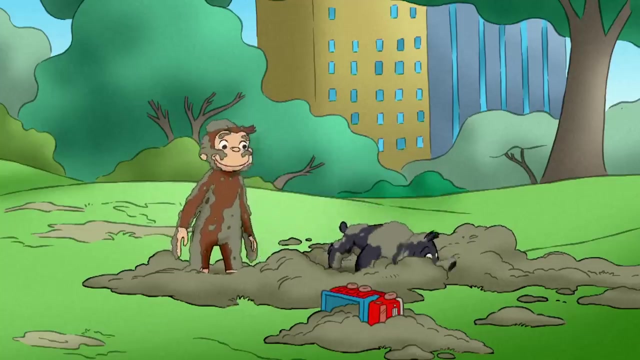 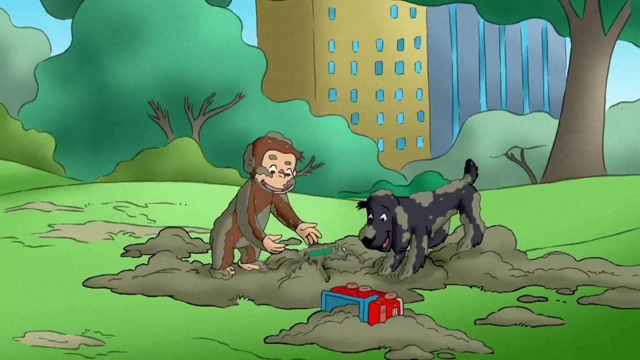 George. Yeah, Charky wanted to play in the mud too. Woo-ha, Woo-ha-ha, Woo-ha, Woo-ha, Woo-ha, Woo-hoo-woo, Woo-ho. Hey, George. 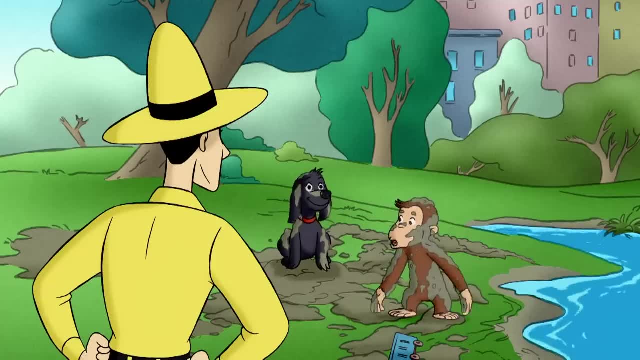 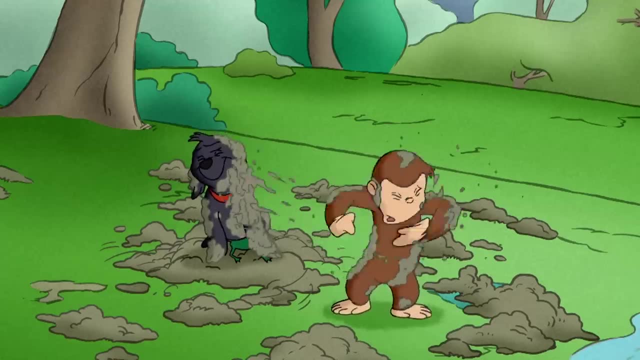 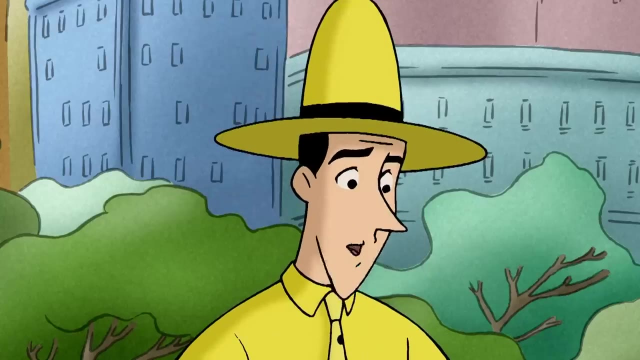 What do you say? we go home and grab some lunch. Ha ha, ha ha. Maybe you should try and clean up a little bit before we go. Ha ha, We could be here all day doing this. You can clean up at home, George. 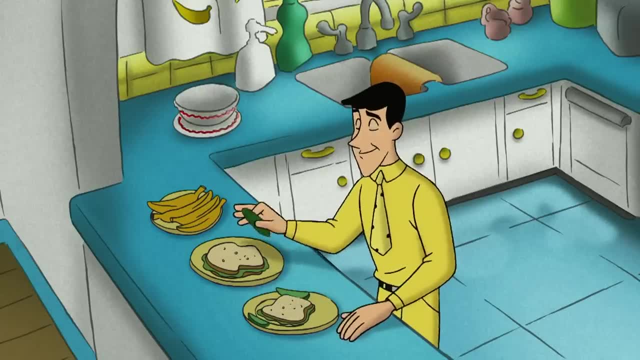 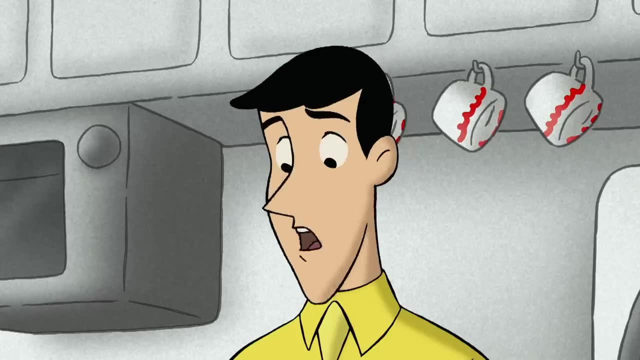 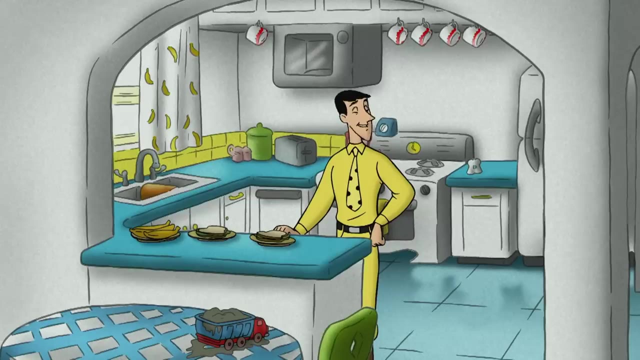 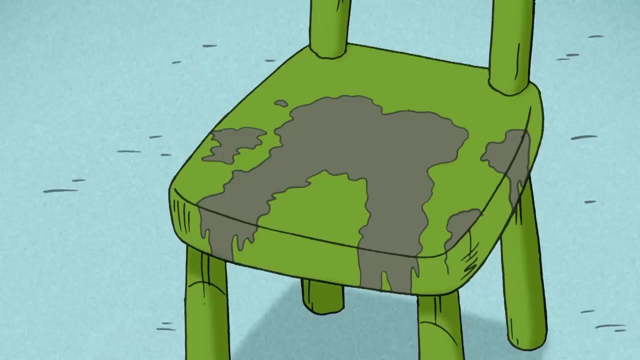 Okay, George, lunch is Ha ha ha ha Ready. Ha ha ha ha. George, you have to get cleaned up before you can eat. Just take a quick bath, I'll wait. Ha ha Ah. There were only two things. 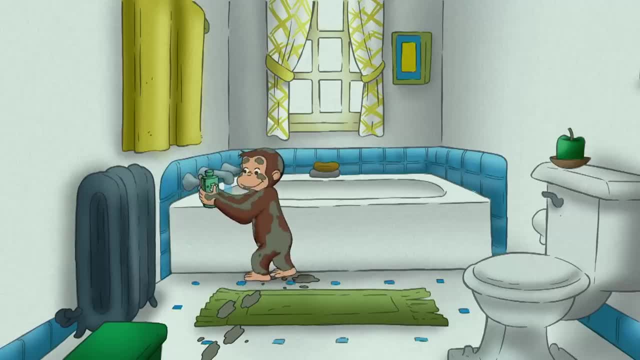 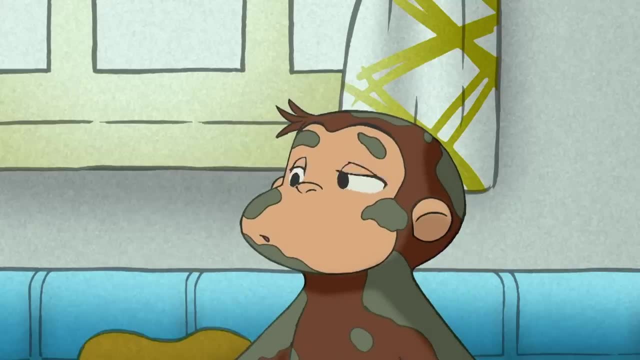 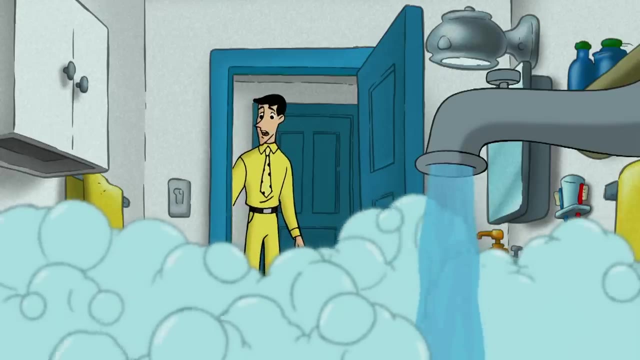 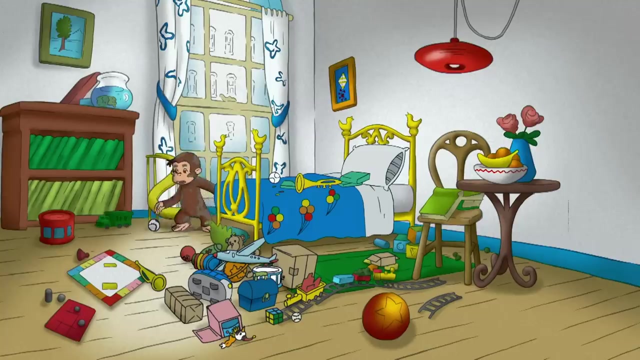 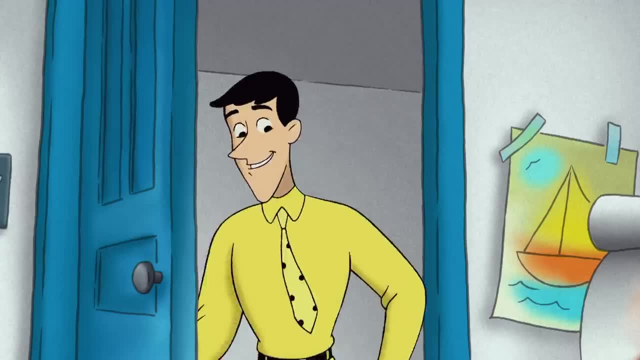 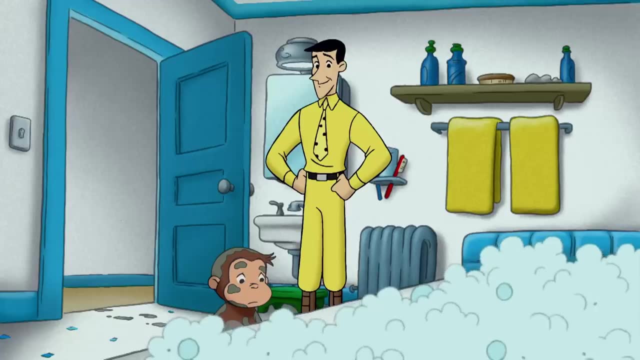 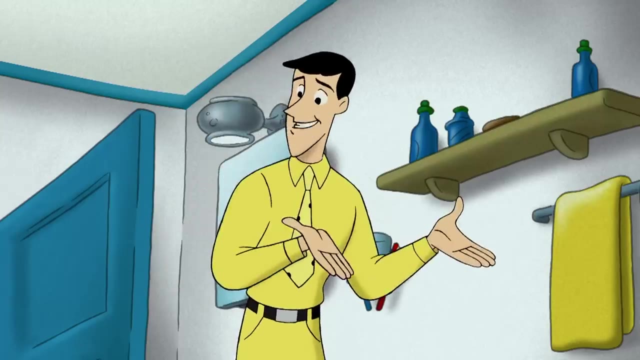 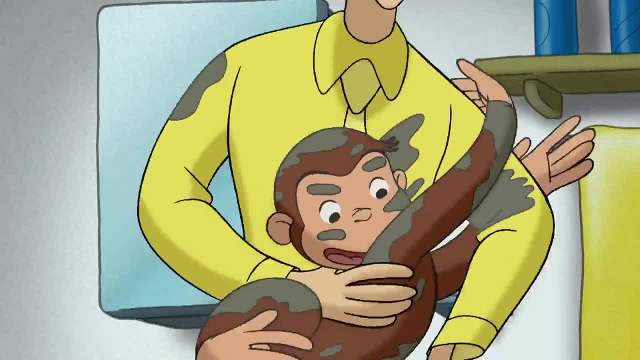 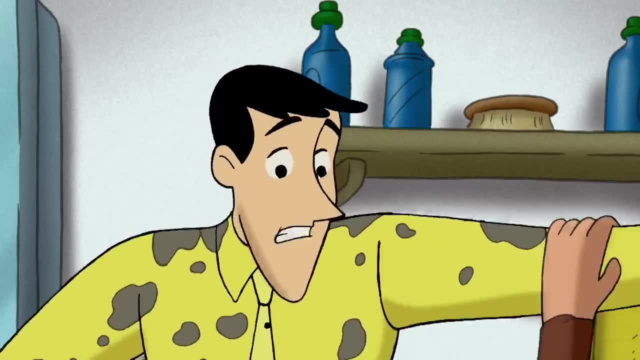 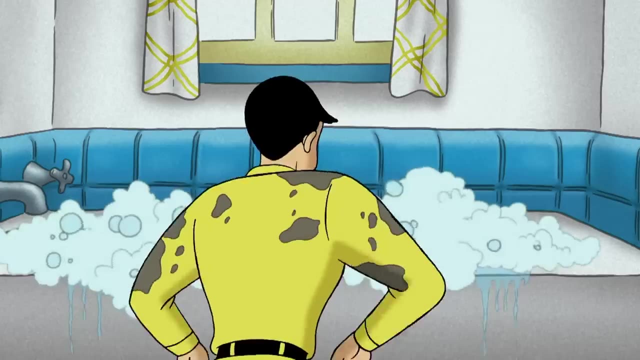 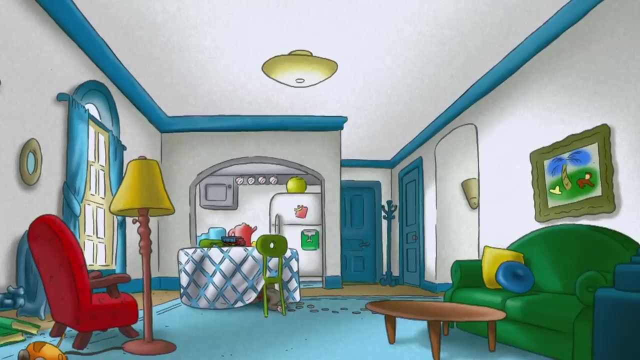 Alright, here we go Into the sea. Hey, You're tickling me, Look. I know you took a bath already this morning, but you're muddy, George. There was no way George could take a bath without Sproingy, who had to be around here. 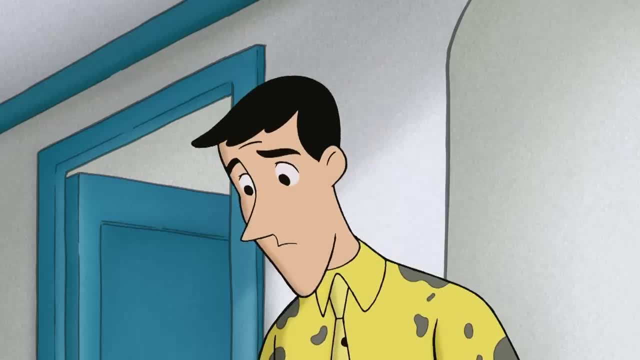 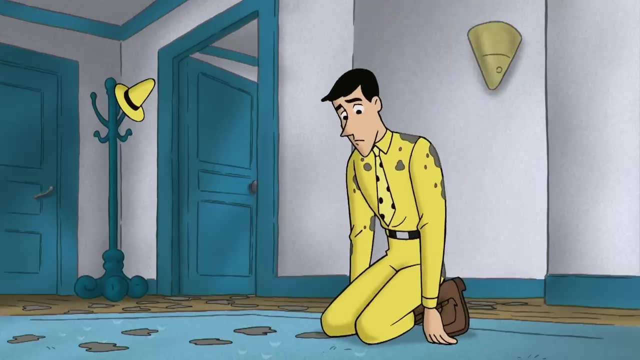 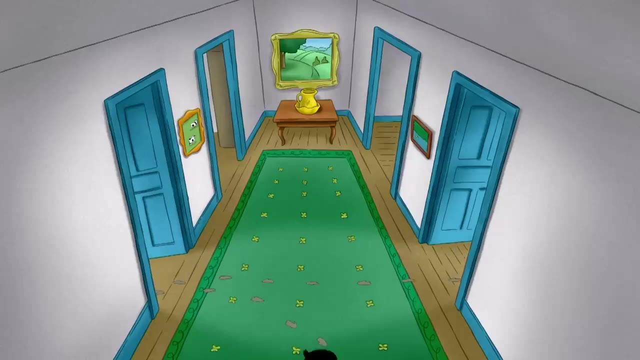 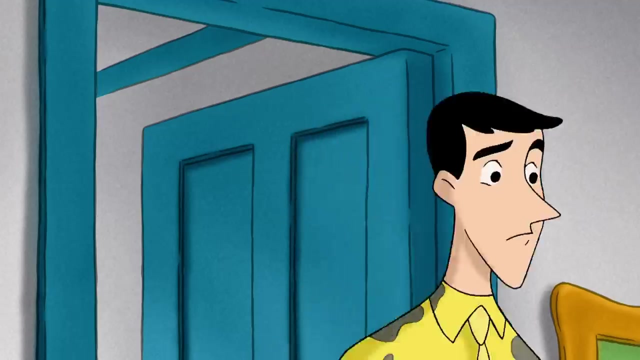 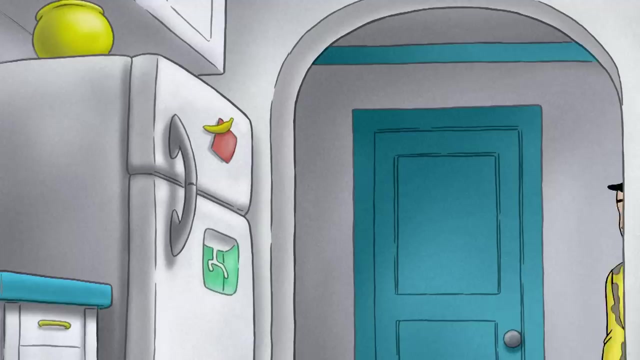 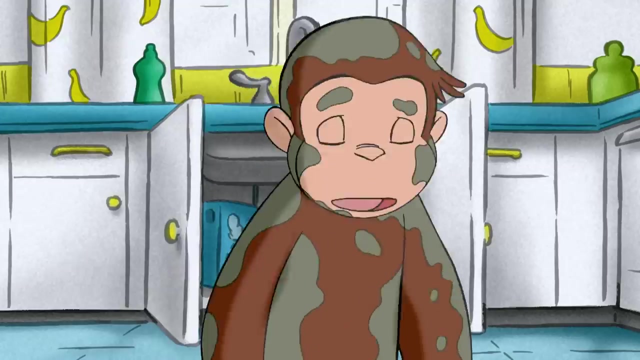 somewhere and there was no way George was going to admit he lost another toy who had to be here somewhere. George, George, George, Aren't you going to take a bath? Are you going to take a bath tonight? You don't know. 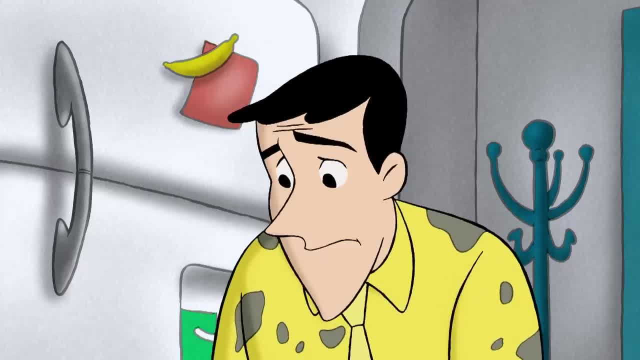 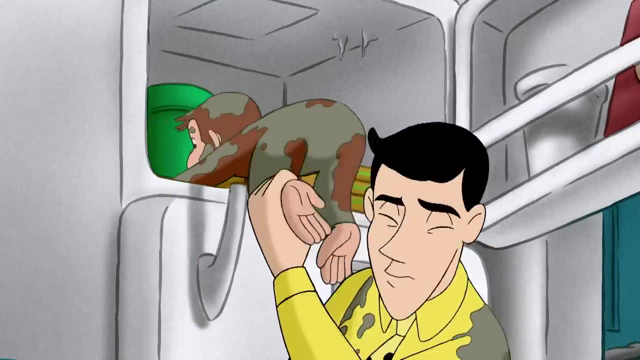 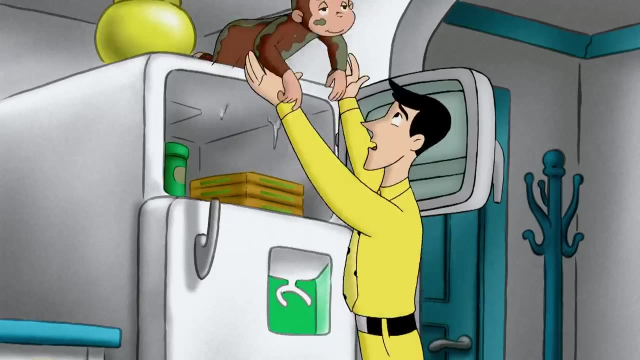 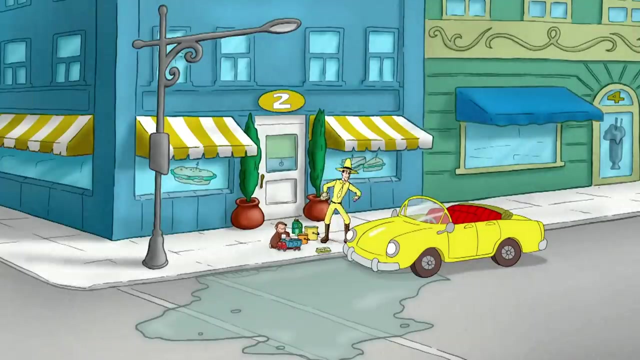 You don't know Tomorrow Ever. Oh well, I can't have a muddy monkey messing up the apartment. Okay, George, forget about giving yourself a bath. How about we give your truck a bath? You don't mind if I wash my car while you wash your truck, do you? 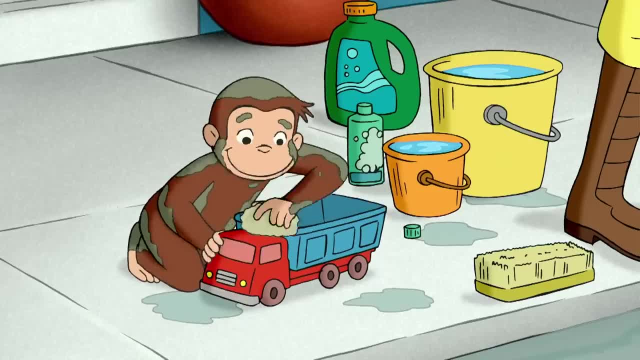 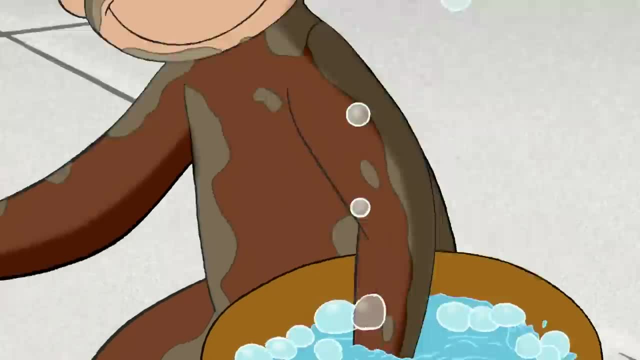 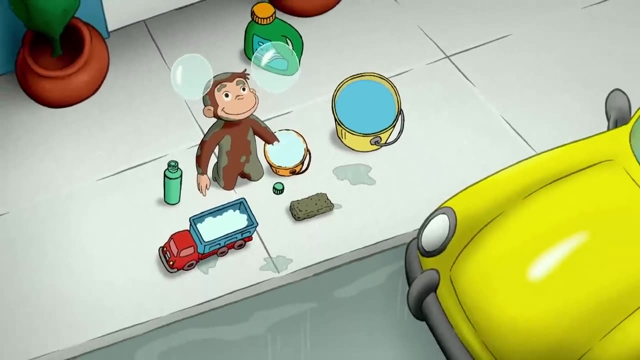 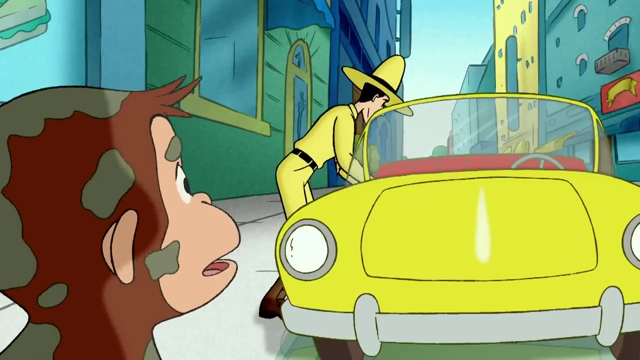 George loved making bubbles anywhere. He didn't need a tub, a bucket of water and a little soap. work too. They were so light and shining and filled with air. But making bubbles reminded him of Sprungy There. all clean, Good job. 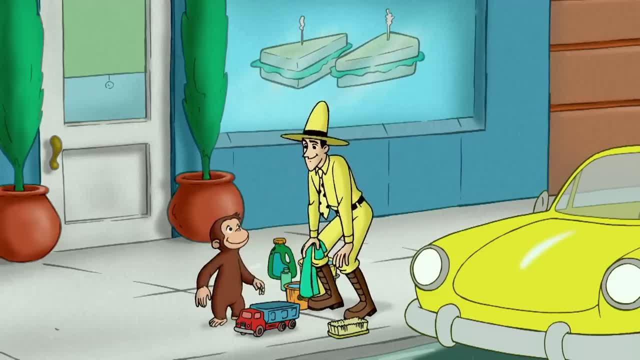 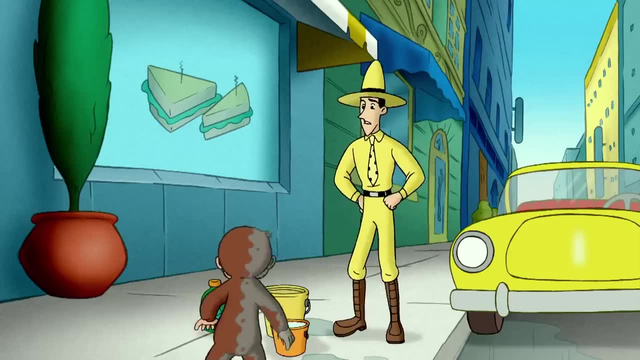 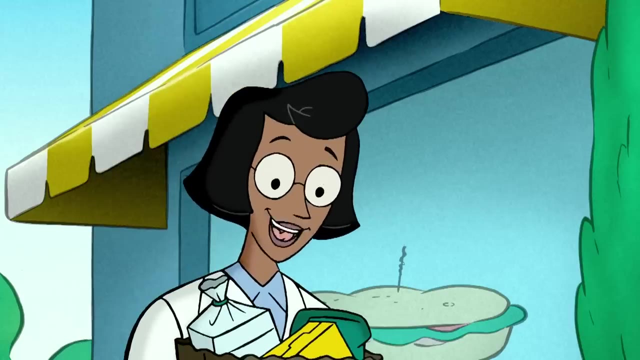 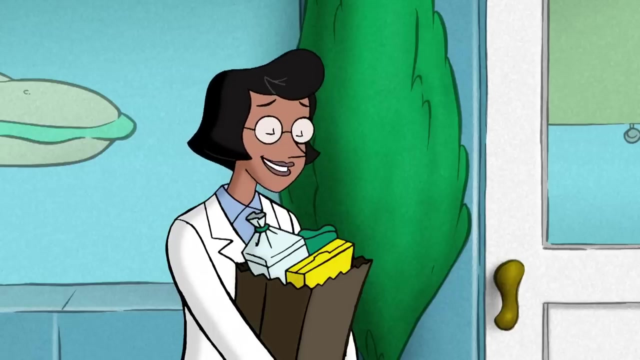 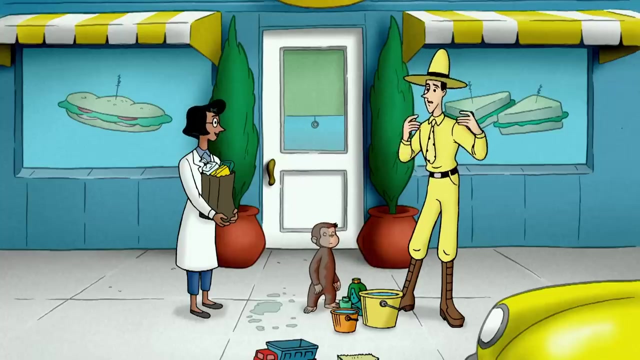 Oh well, at least the right half of you is. I guess someone's due for half a bath. I wish, but George won't take a bath anymore. I don't get it. Maybe George feels he's getting too old for a bath. 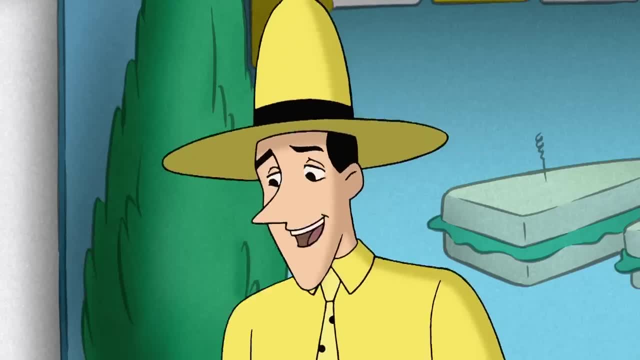 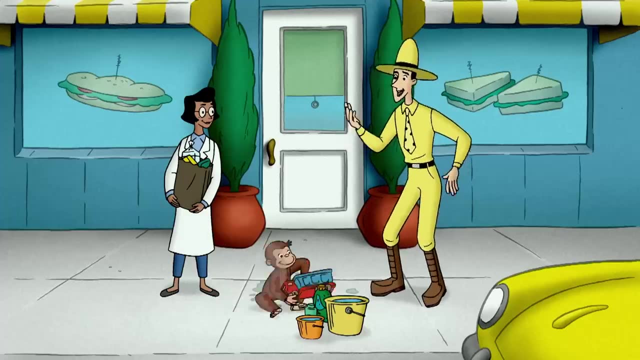 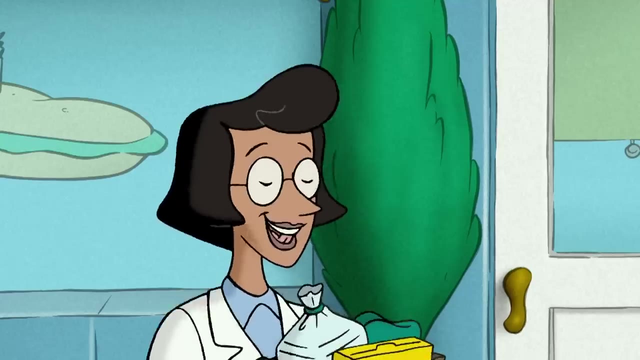 Of course, that's it. My little monkey is growing up. Now I know exactly what to do. Come on, George, we're going in. Oh thanks, Professor Wiseman, You're a genius. Well, yeah, I understand. 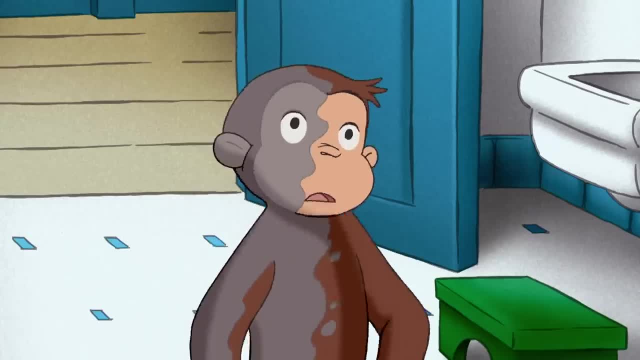 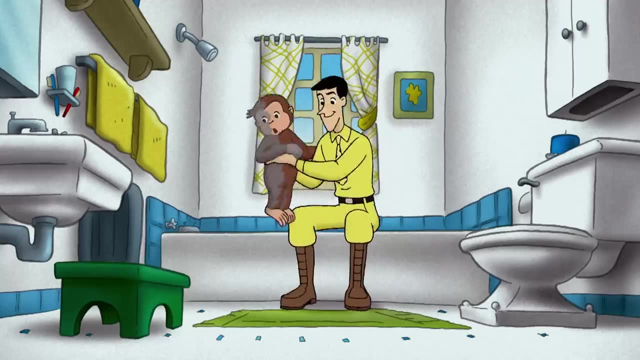 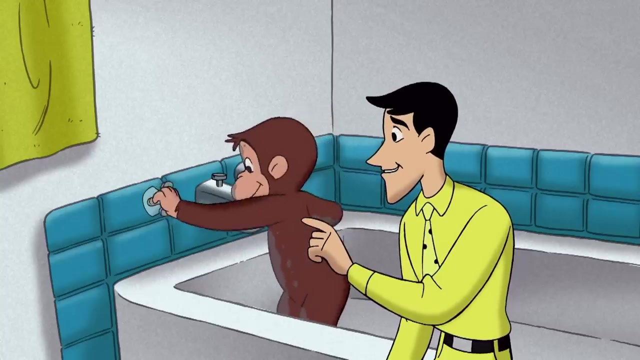 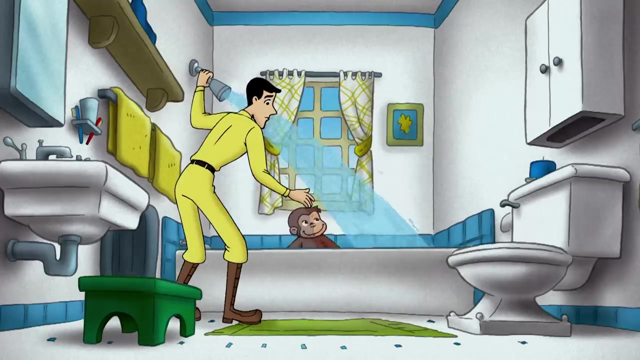 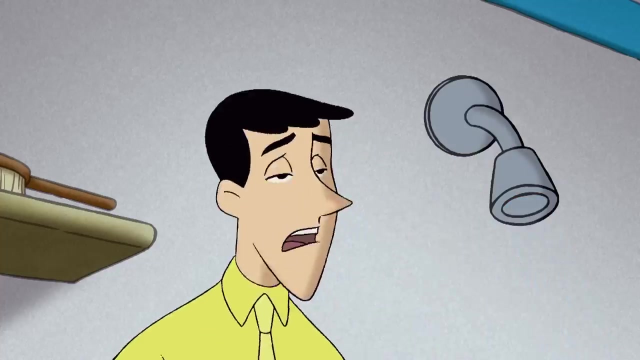 I understand your problem with baths now, George, And I agree It's time for you to start taking showers. Turn on the water, George, and see what happens. Oh, George, George, Okay, Won't take baths, won't take showers. 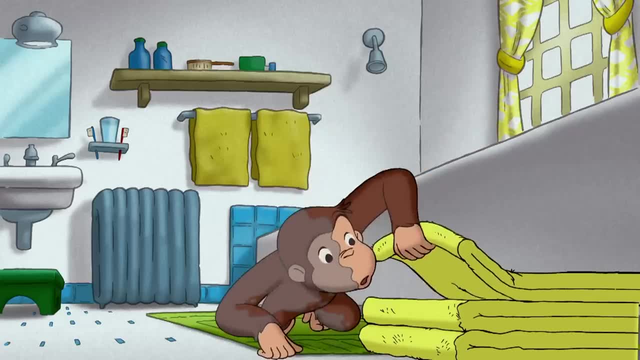 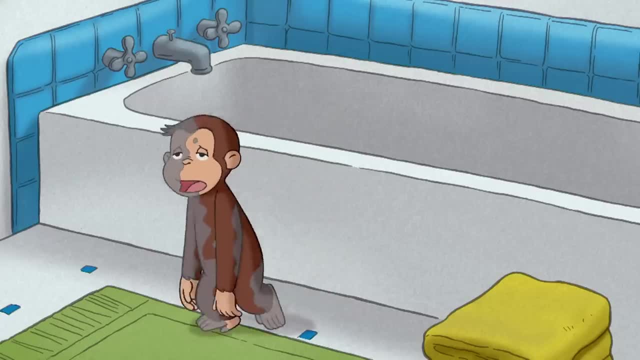 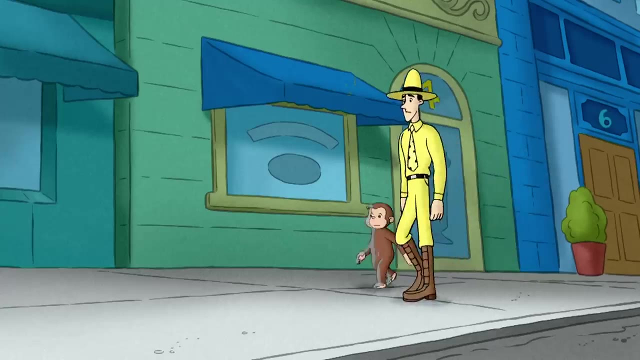 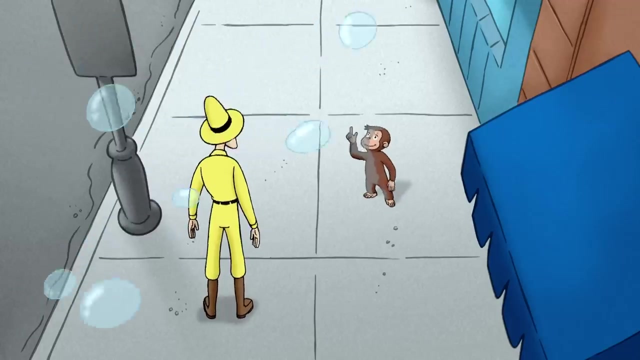 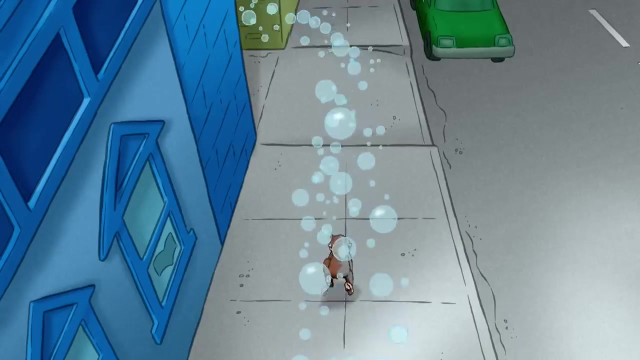 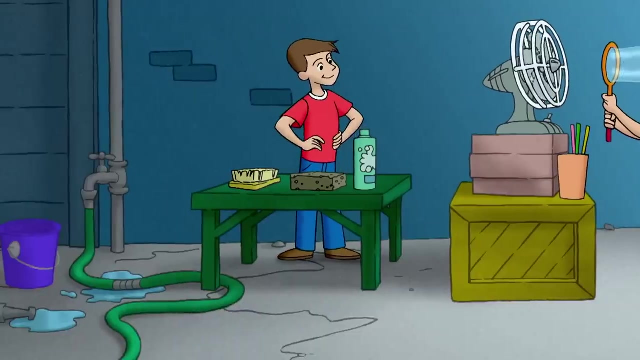 I need to take a walk and not think about any problems for a while. But sometimes not thinking about something is harder than you think. Bubbles, Maybe, somehow. Springy was nearby. Hi Betsy, Hi Steve, Hello. 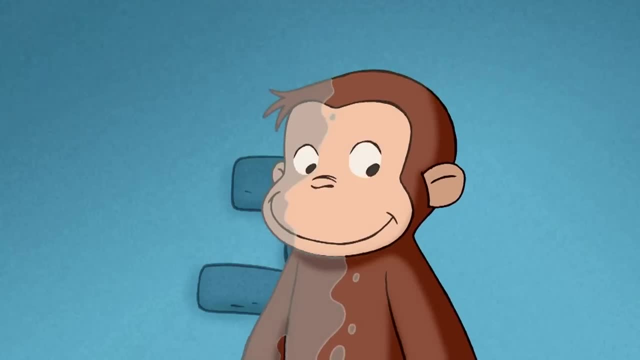 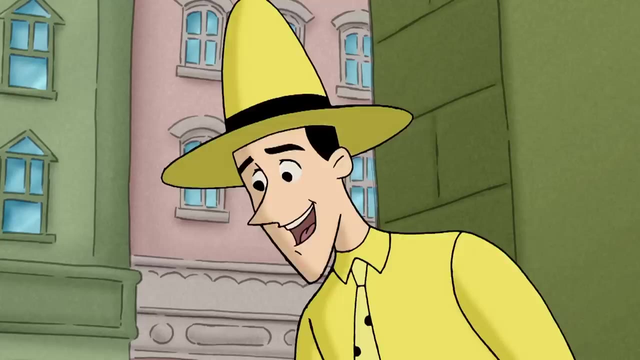 Betsy made pretty good bubbles, But she was no plastic frog. Hey, George, We're washing dogs to make money. Want to help? Uh-huh, Yeah George, Why don't you help? There's soap and water and bubbles andsoap. 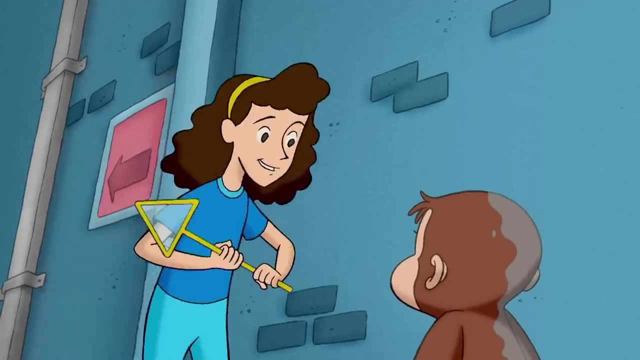 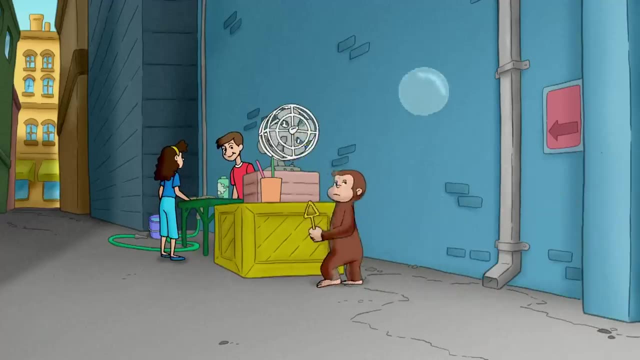 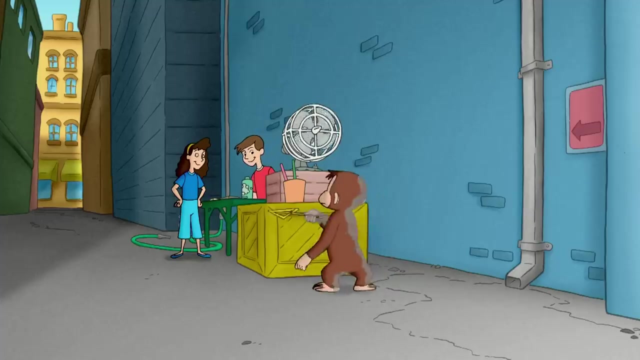 Great George can help me make bubbles to attract dirty customers. George figured the triangle bubble maker was broken, But a square bubble would be just as good. Huh, They fooled me the first time. I tried them too. It doesn't matter what shape bubble maker you use. 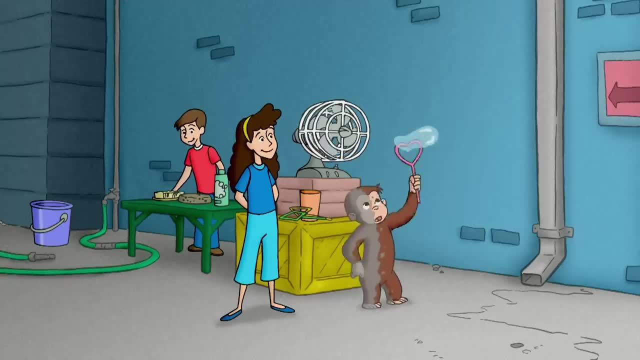 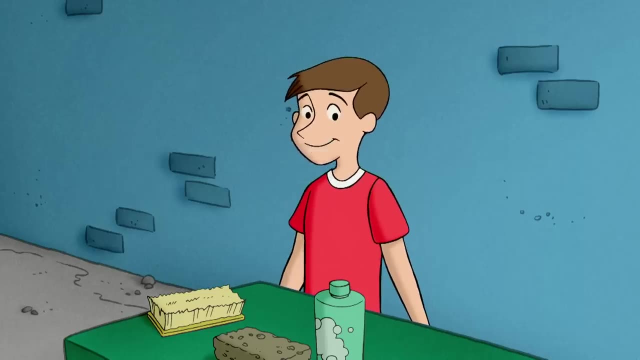 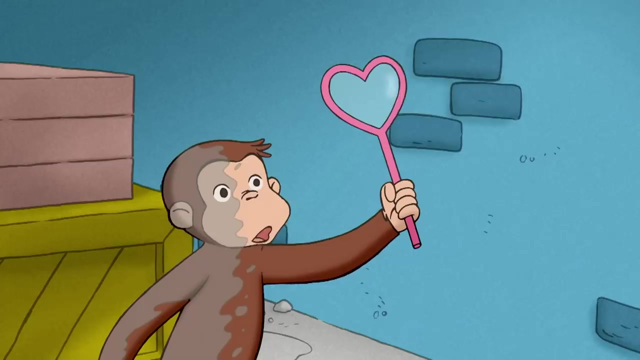 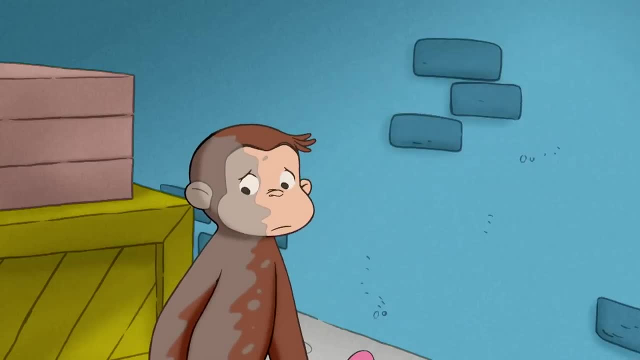 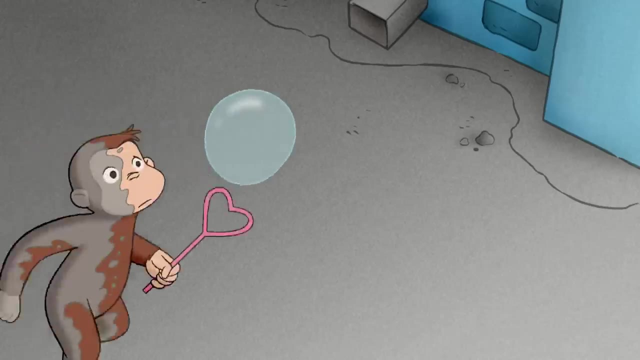 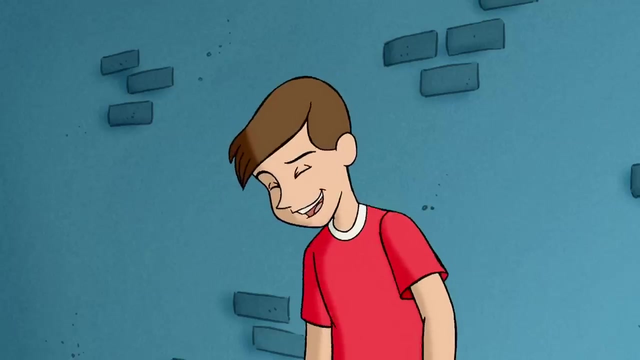 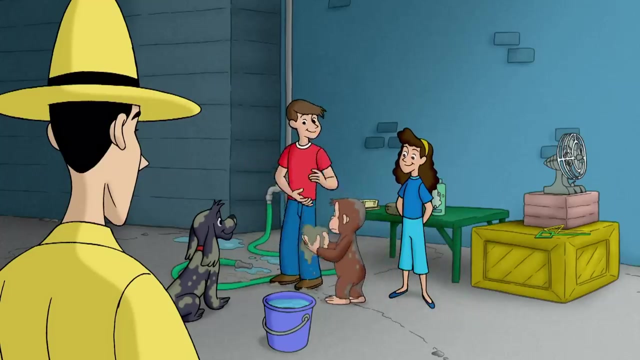 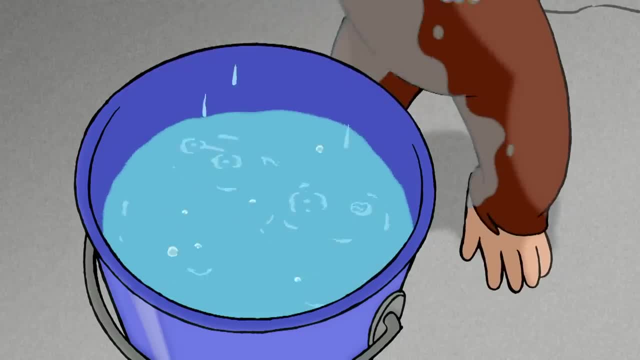 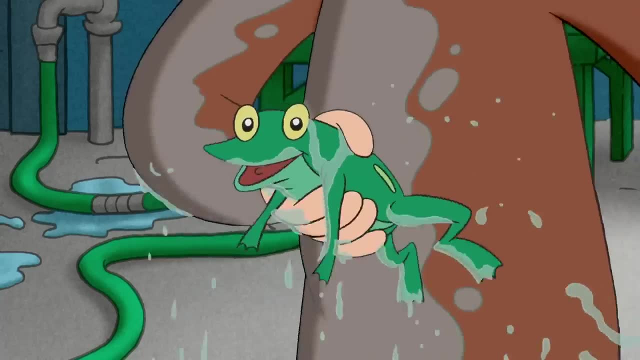 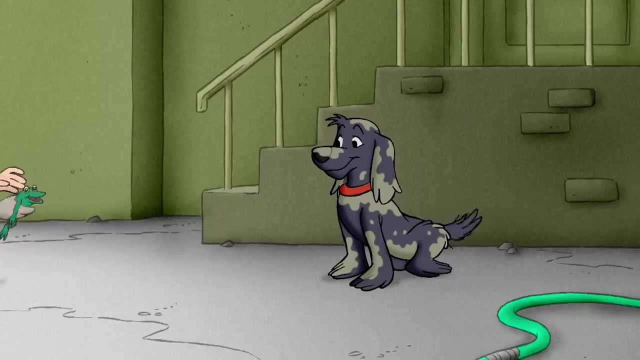 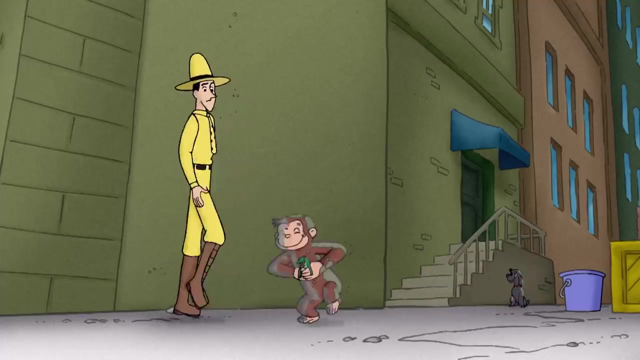 Hey, George, would you help me? Could you wash Charkey's ball? Yeah, Happy Sisters' Of course, the park, the mud, Charky. No, no, no, no, you're getting dirtier, George, slow down. 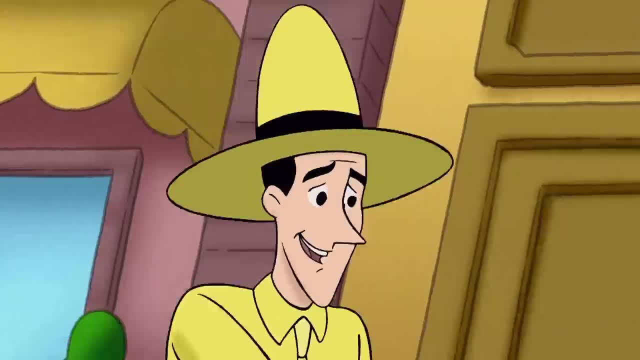 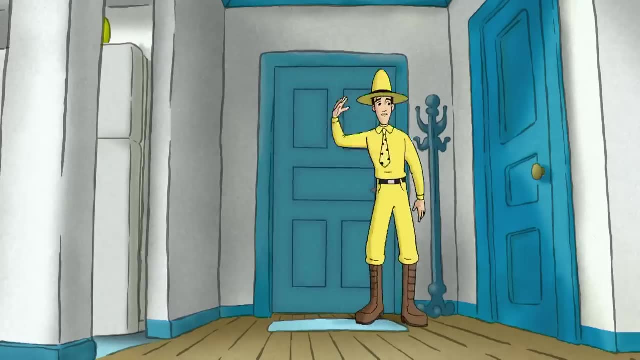 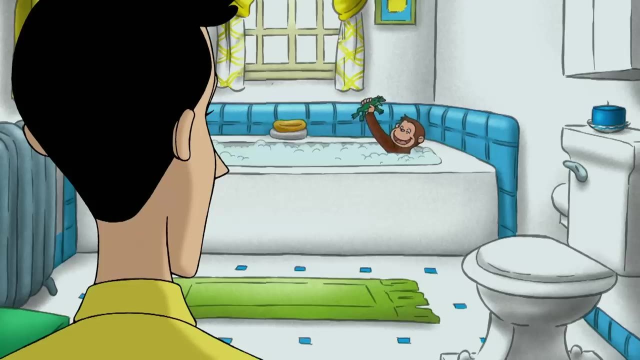 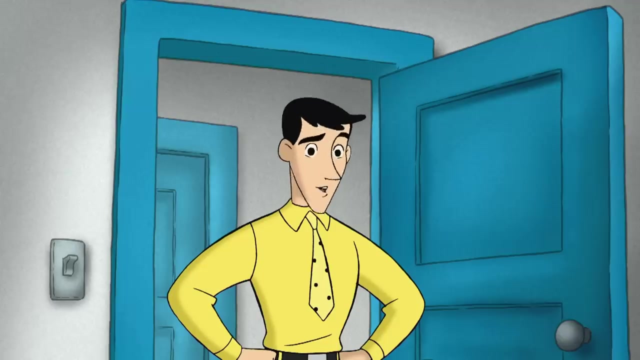 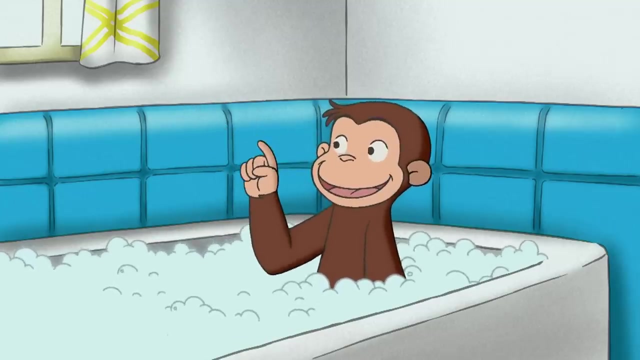 Okay, I'll meet you back home. You beat me home. Why were we racing? George, you're taking a bath. Okay, then enjoy. I, um, wow, I wonder what that was all about. A bath, A bath just wouldn't be a bath without bubbles and sprungy. 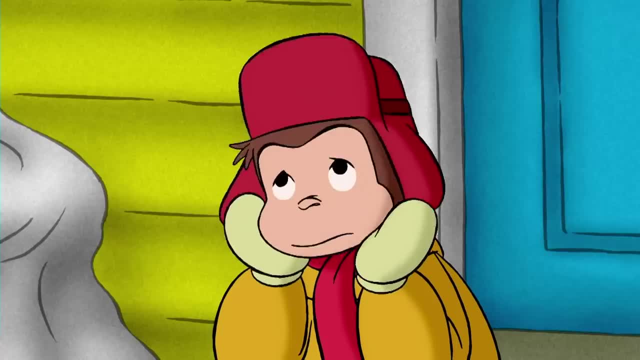 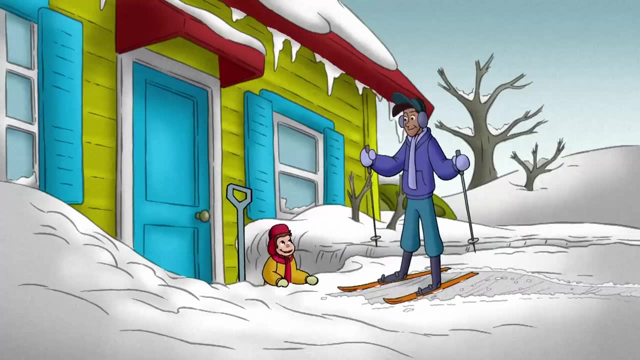 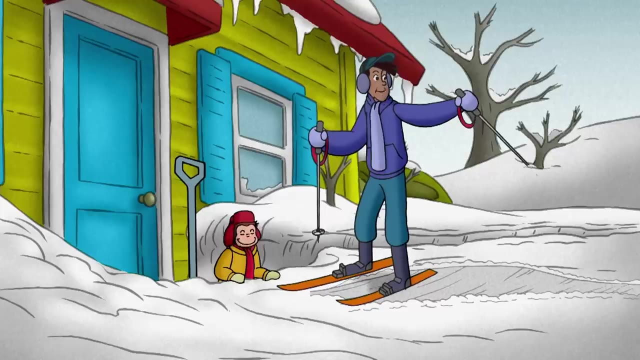 Here was all this fresh snow just itching to be played with, but it was too deep for George. Hey, George, Hey, Hey, George, Hey. I guess a city kid wouldn't have seen cross-country skis before. It's the most fun way to travel on deep snow. 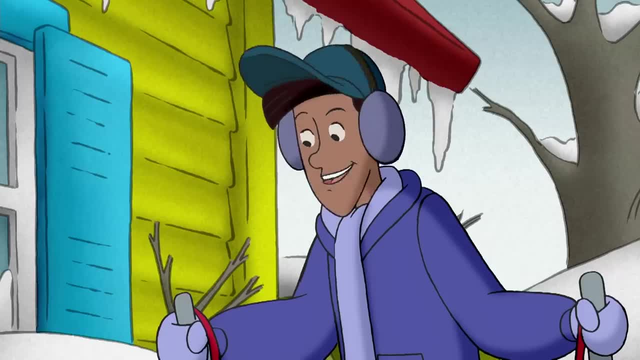 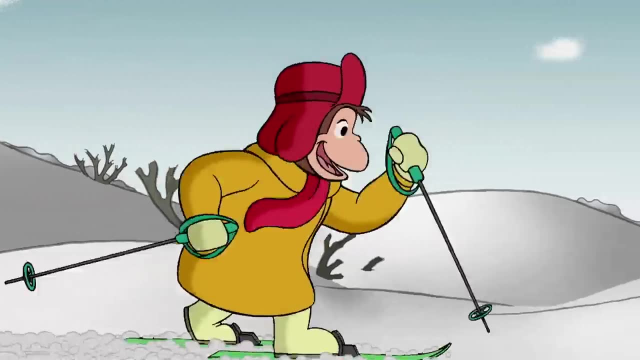 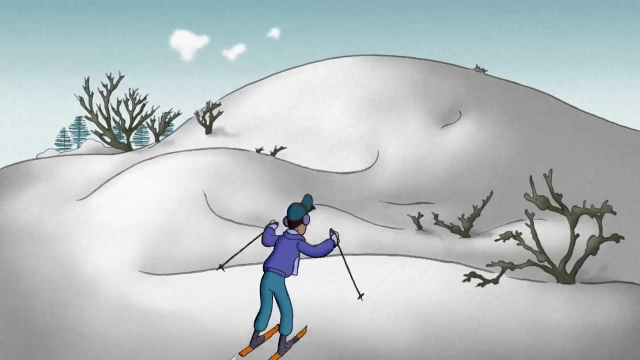 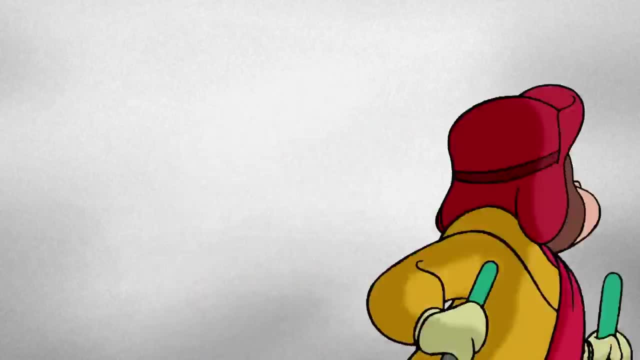 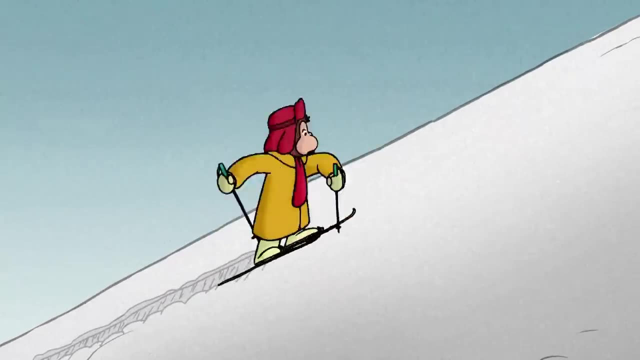 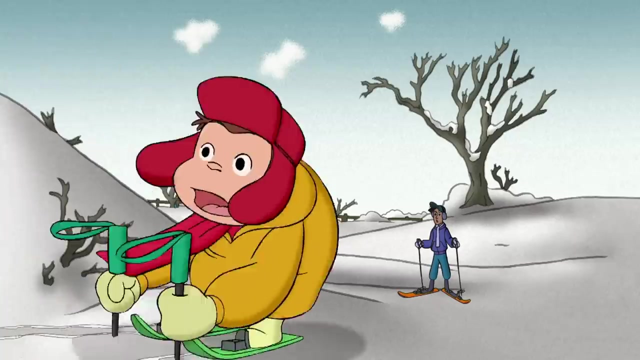 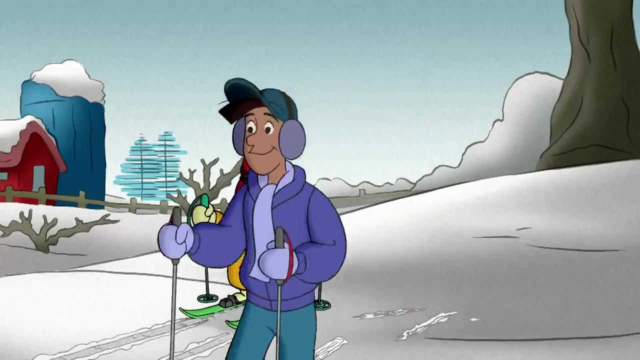 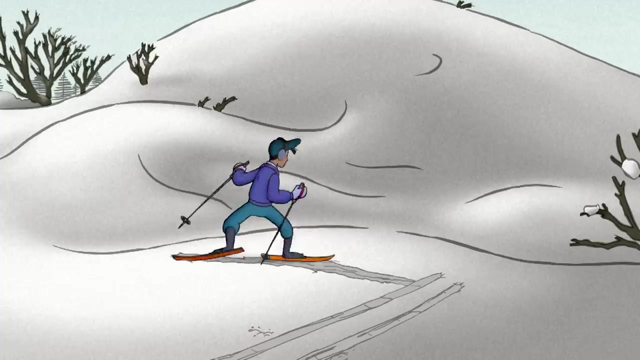 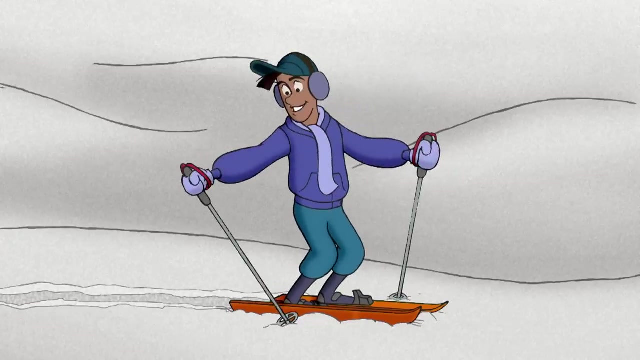 I can't handle that big hill With skis on. George could go anywhere. there was snow, Or so he thought. You can't attack a steep hill straight on like that, George. You gotta zigzag it When you stop, angle your skis like this so you don't slide back down. 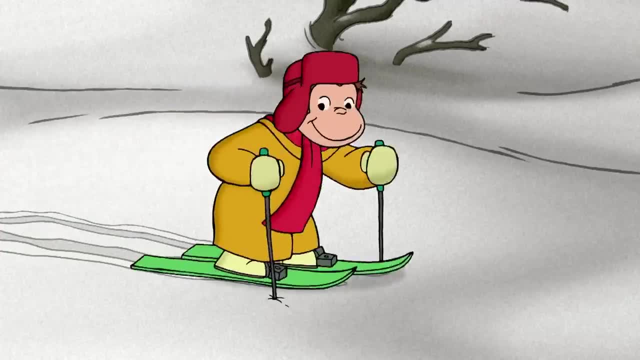 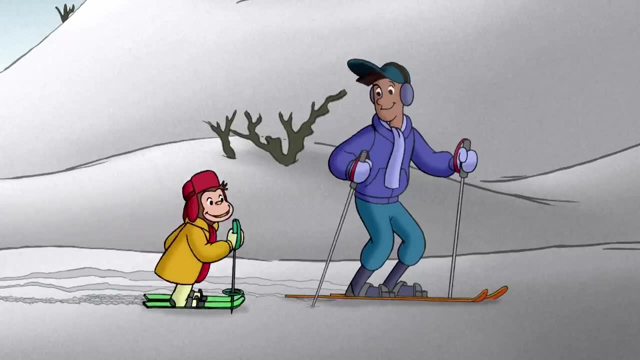 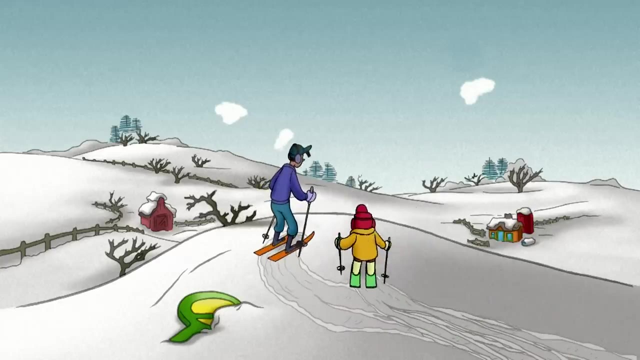 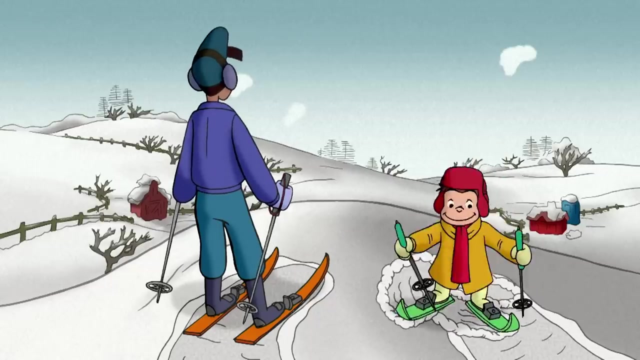 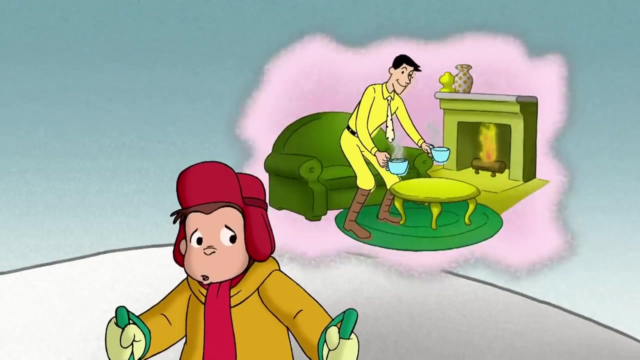 Yeah, that's it. There you go, George. That's the way to do it. George had a great view up here. He could see houses and farms And there was his house, And then he thought he'd better head home right now because the man was making the last of the cocoa. 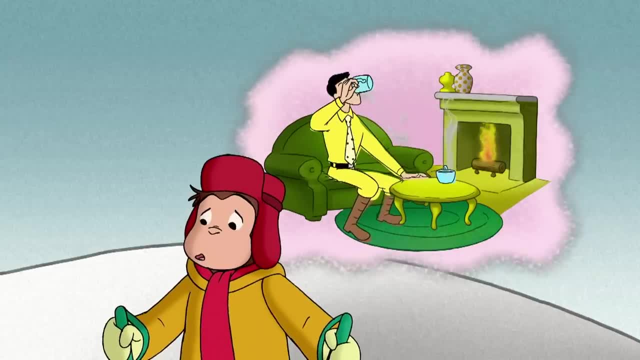 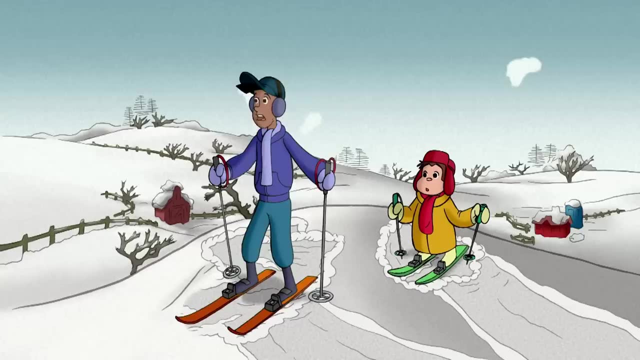 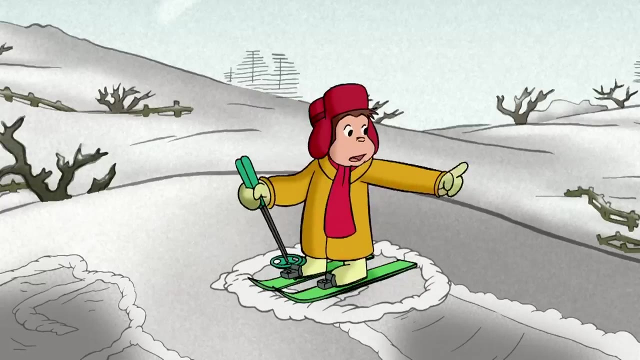 And no one can resist the drink-me-now power of cocoa, Not even the man with the yellow hat. I wonder what that could be. I'm gonna go take a quick look around You wait here. Ah, Ah, Ah, Ah. 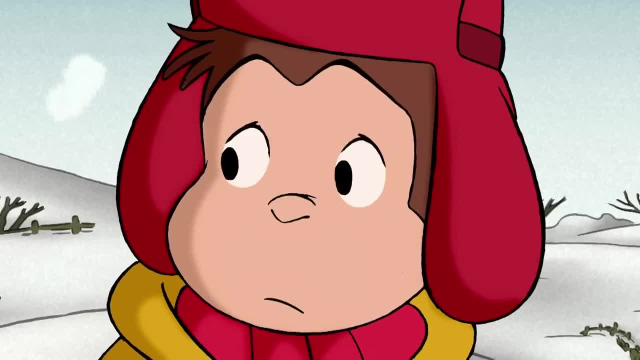 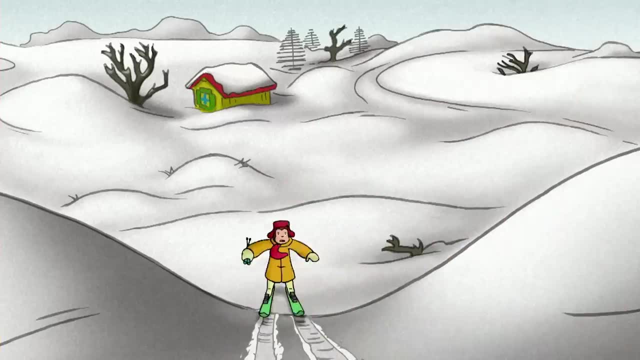 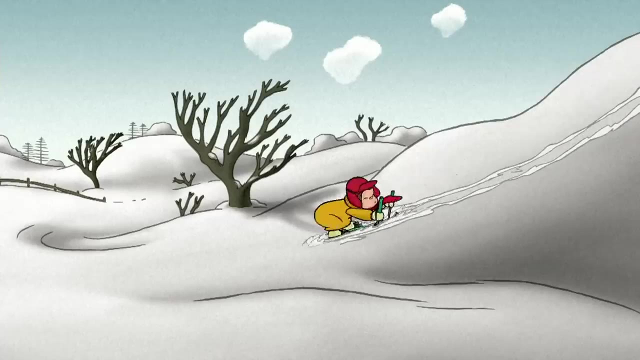 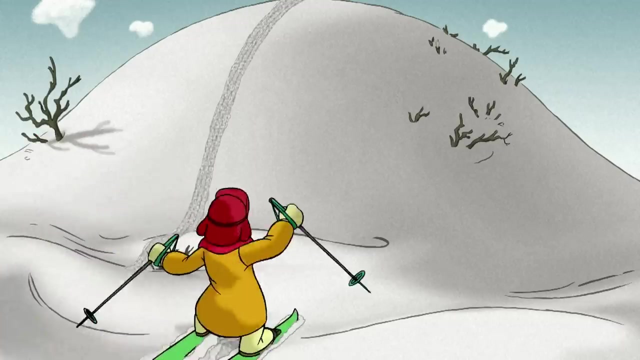 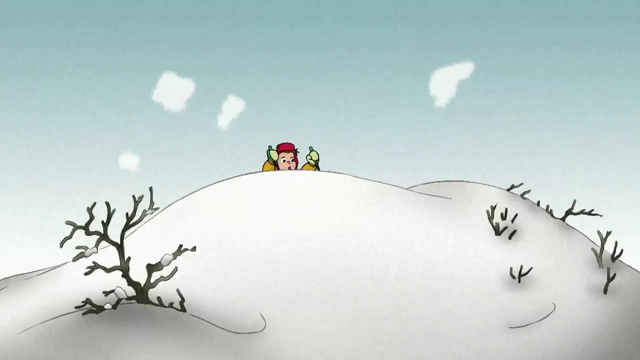 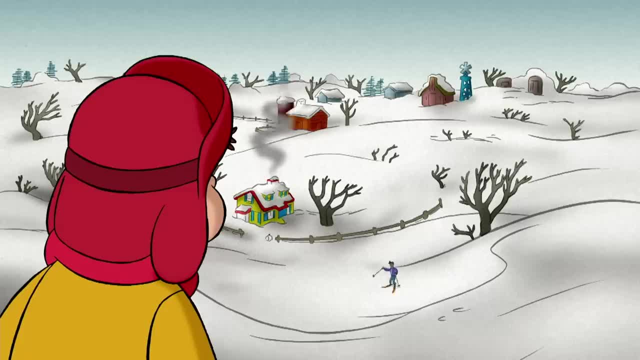 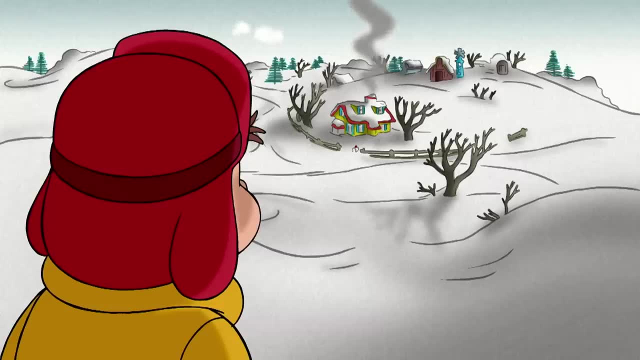 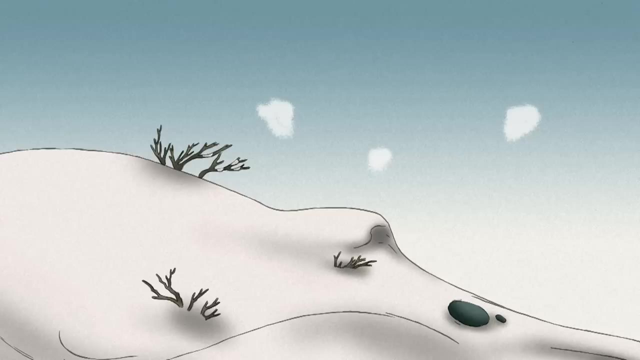 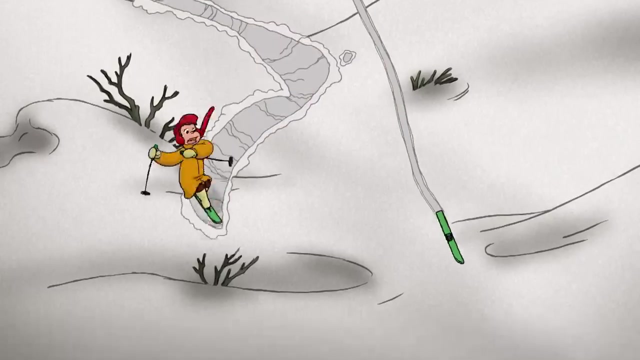 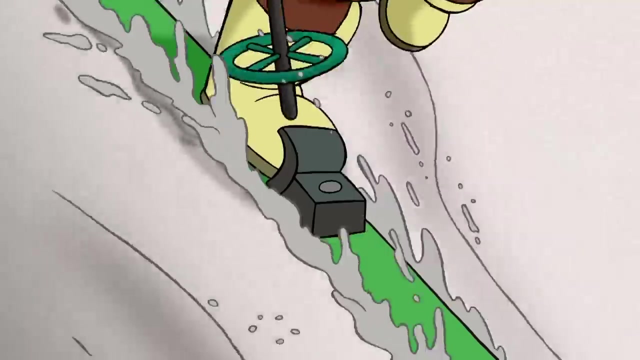 I couldn't find what made that sound. I'm heading home now. Have fun. At least it was all downhill from here. Who figured he'd be home in seconds? There had to be a way to get that ski. Huh, There I was. 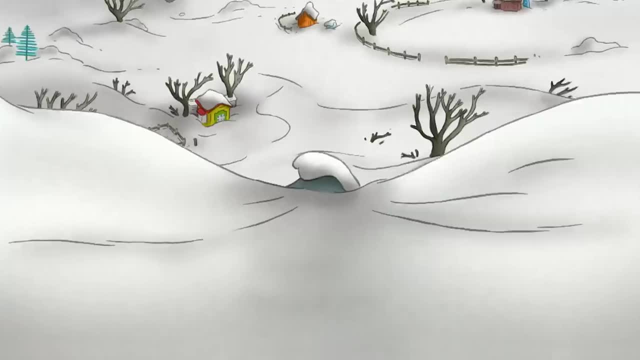 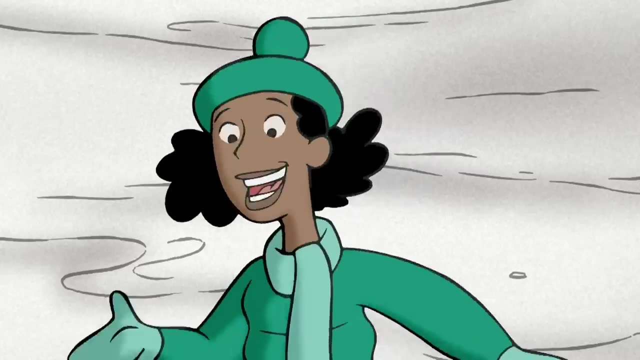 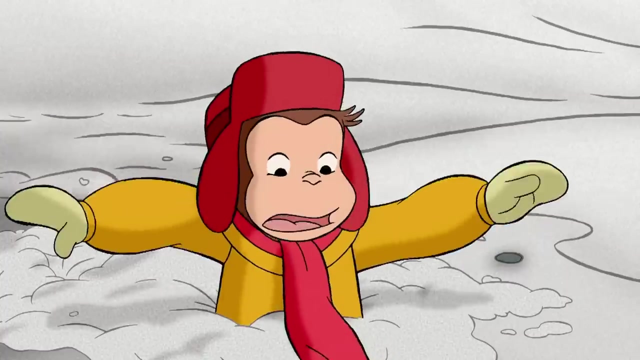 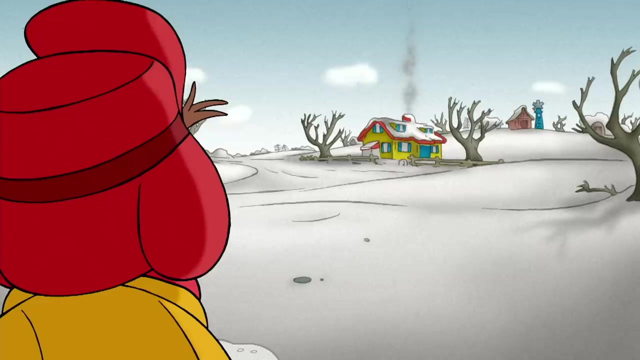 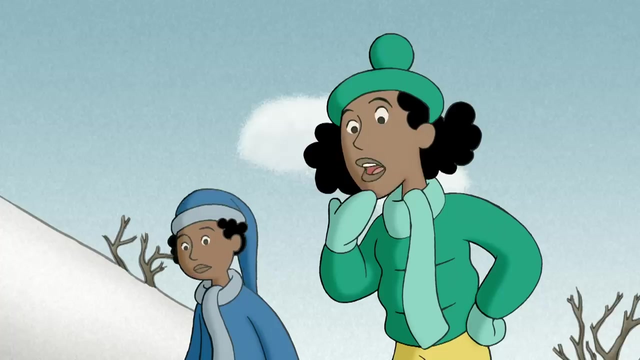 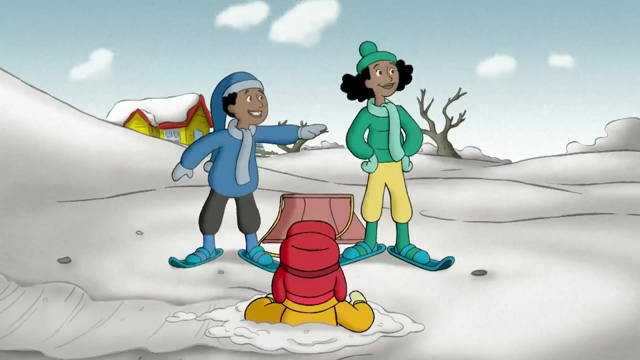 Well, one ski was better than none. That was awesome. There was no way George could walk home in deep snow without skis. I think he likes our snowshoes. I think he wants to borrow our snowshoes to get to that house. He probably lives there. 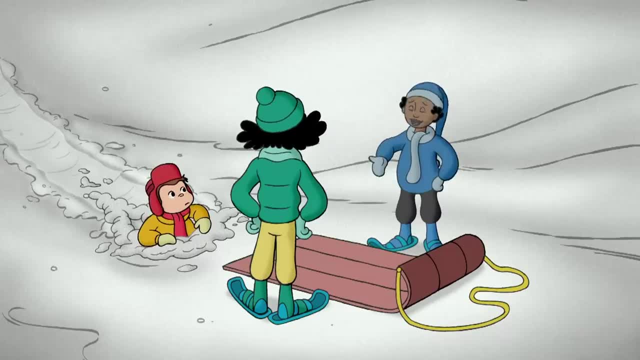 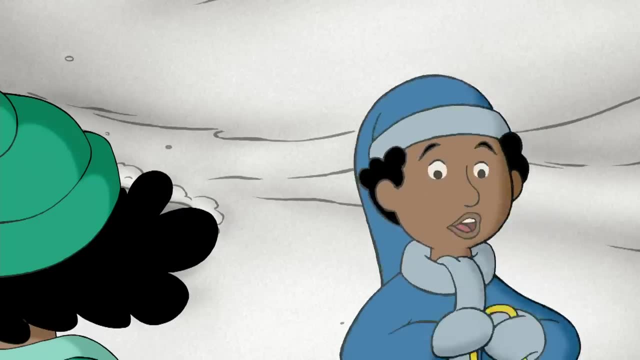 I'll give him mine. Then how do you get home? You can't walk on the snow without them. Let's pull him home on our sled. Kent, we're already late. Mom's going to get worried. We can't just leave him here. How about we get ourselves home first? 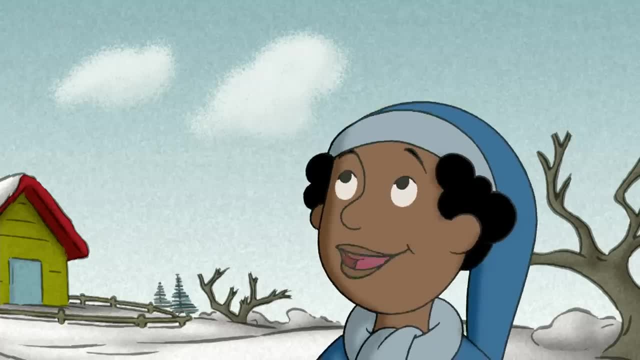 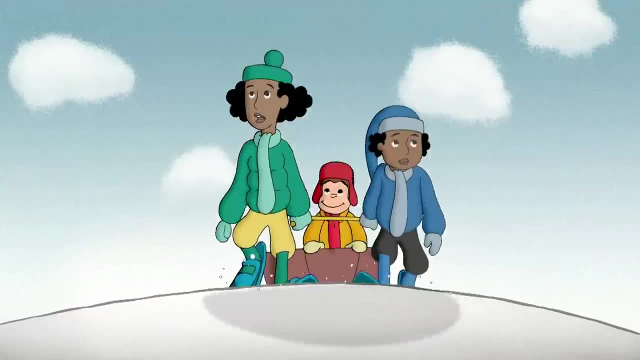 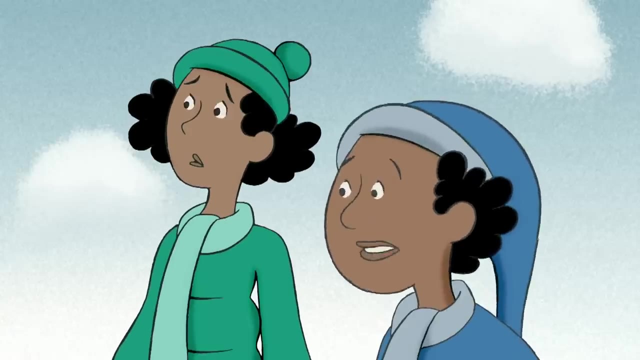 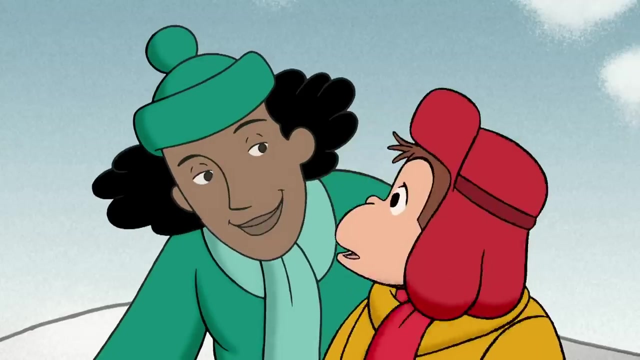 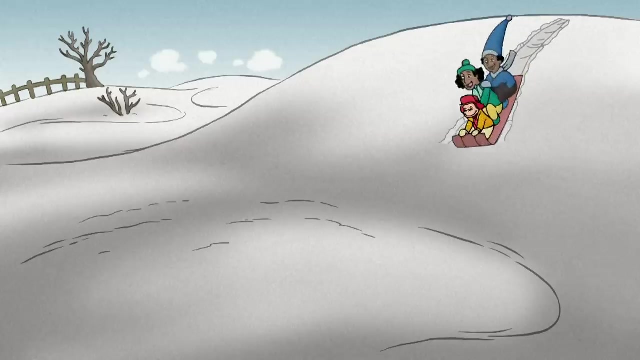 and then we'll give the monkey your snowshoes. We live on the other side of the hill. Climb aboard. There's that weird noise again. It's probably kids like us riding sleds a hill or two away. On your marks, Get set, Go. Why didn't we give the monkey? 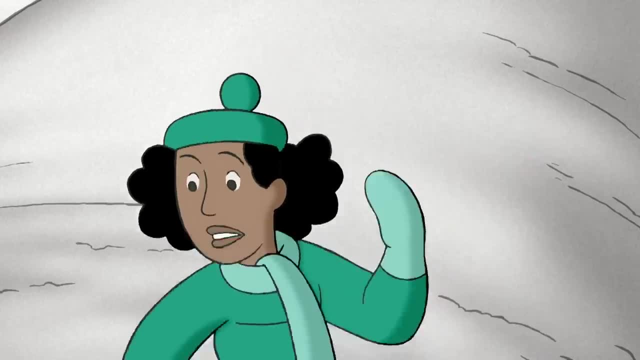 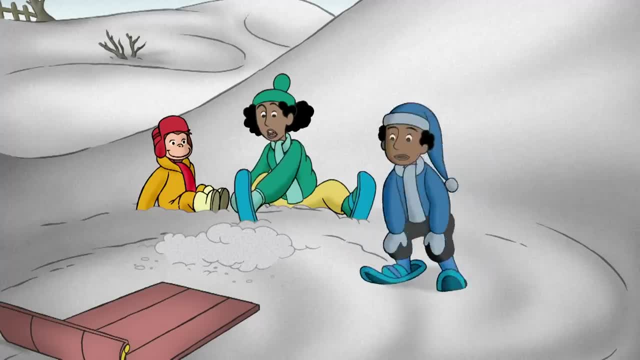 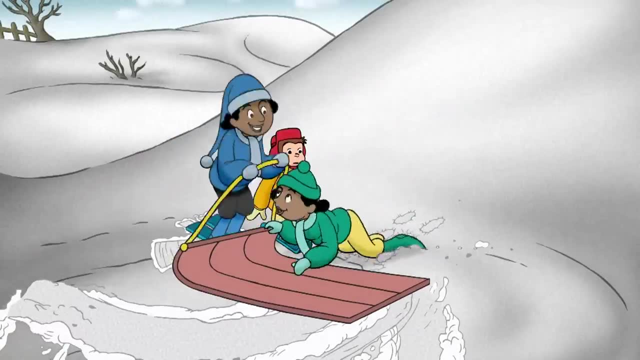 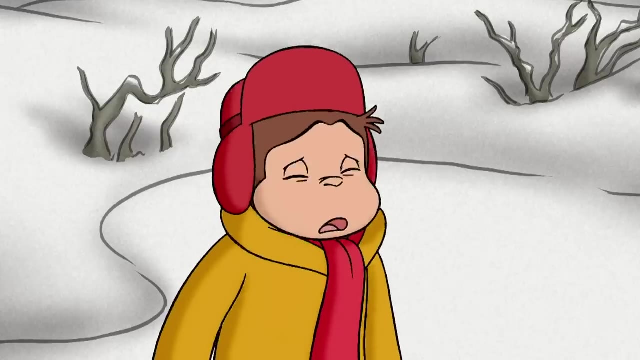 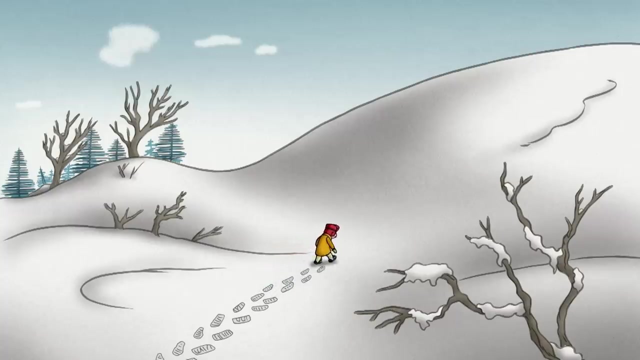 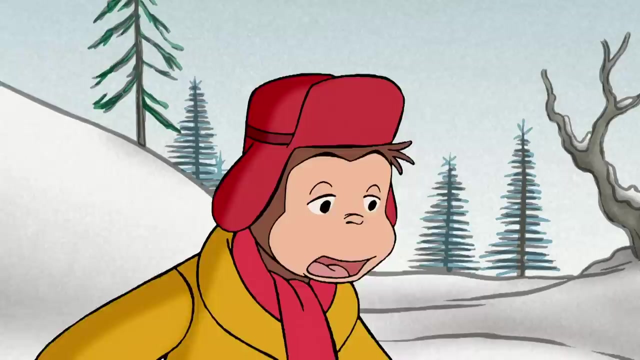 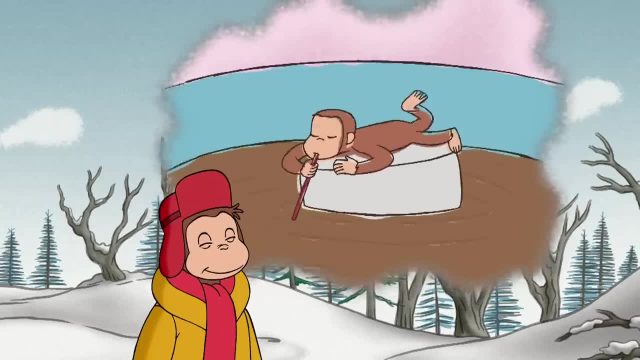 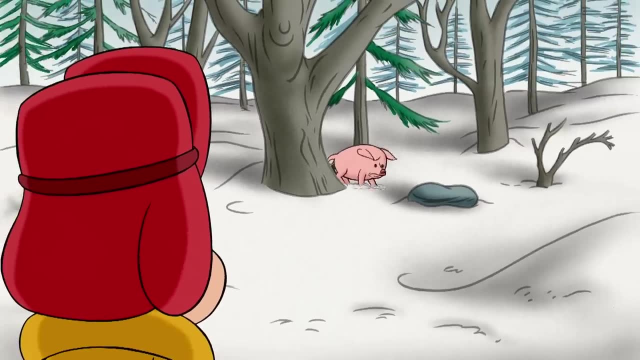 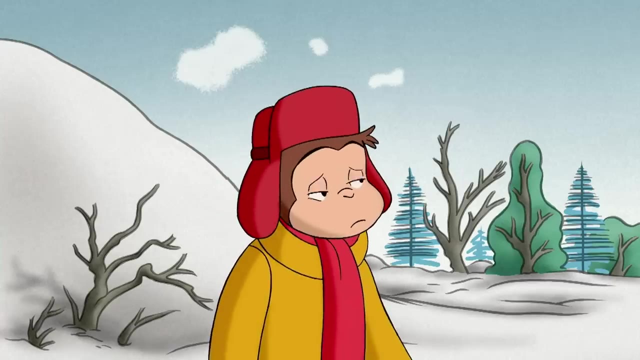 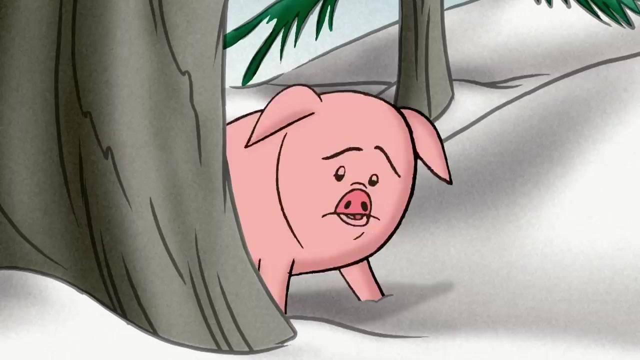 was the joyous hope of Coco. Now George could see what made that sound: a cold, lost pig. George was almost at the top. The pig was way over there. He didn't even know if he could help. We can't just leave him here. The pig was way over there. 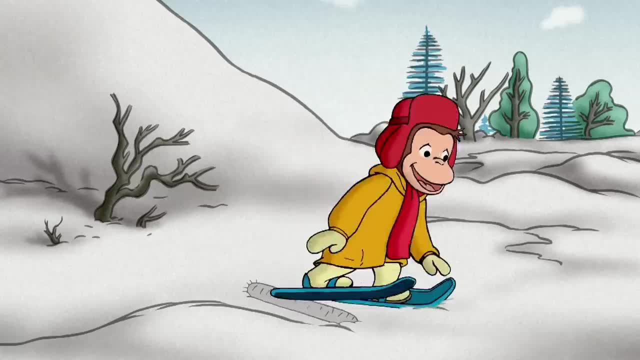 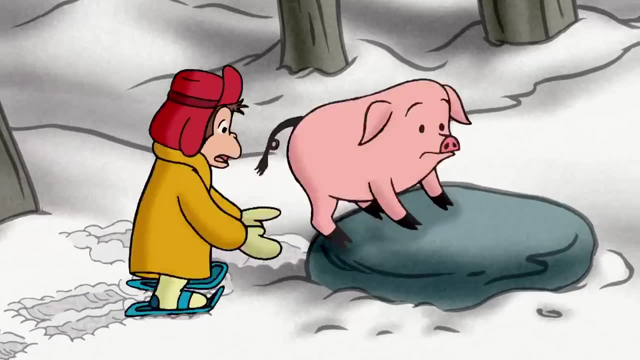 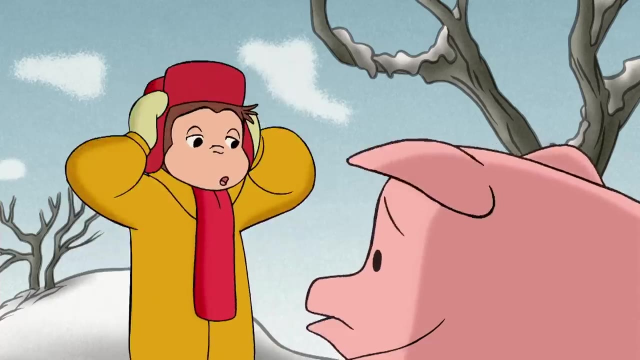 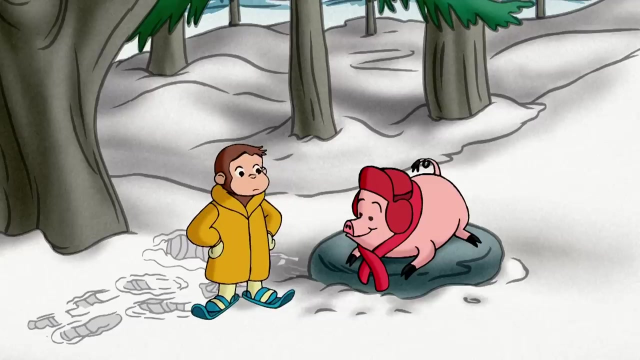 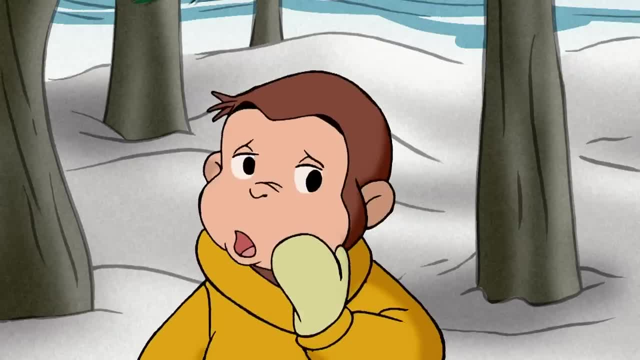 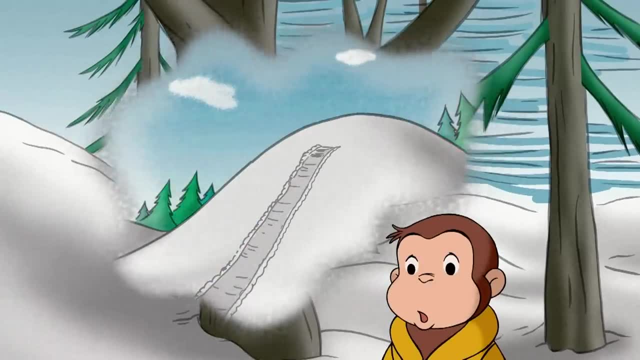 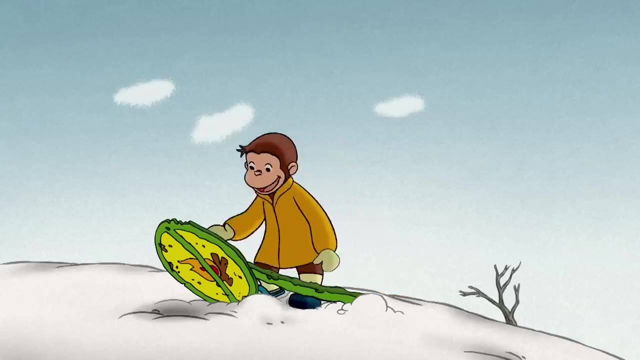 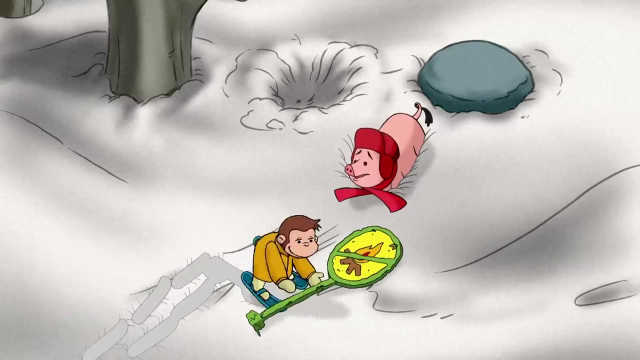 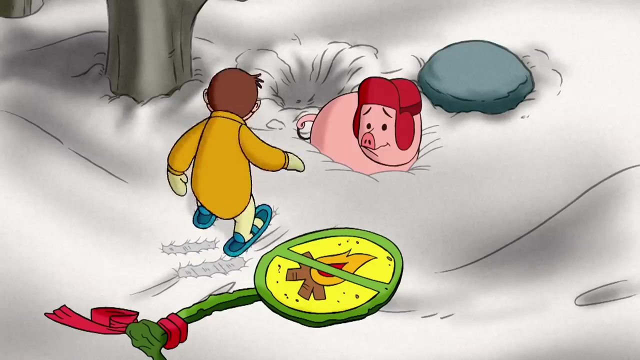 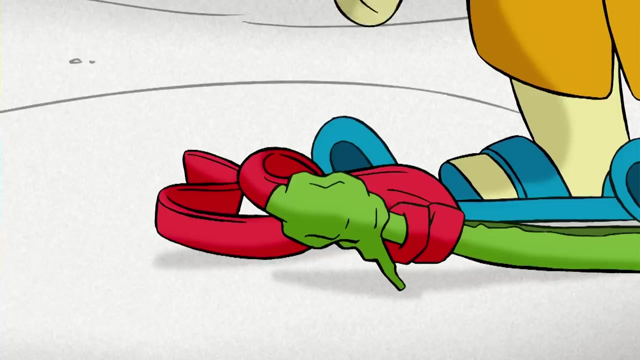 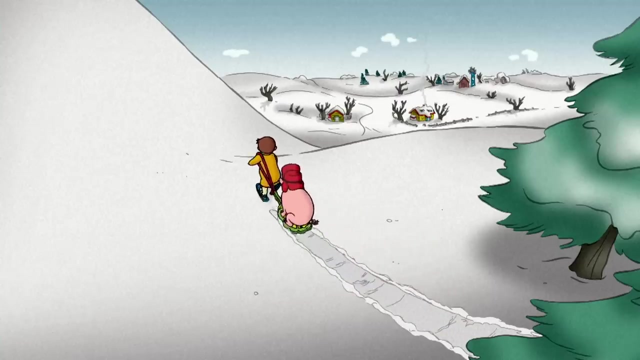 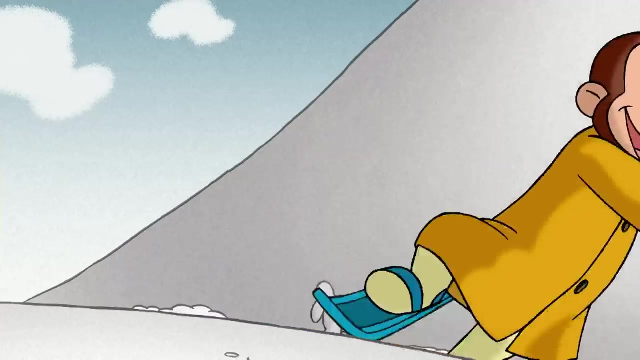 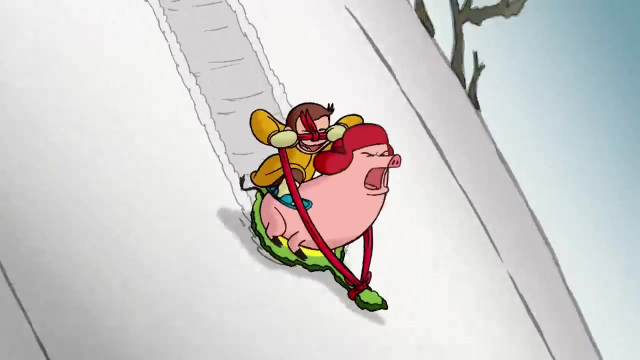 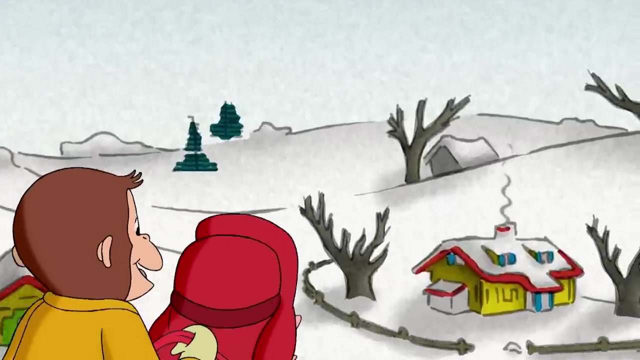 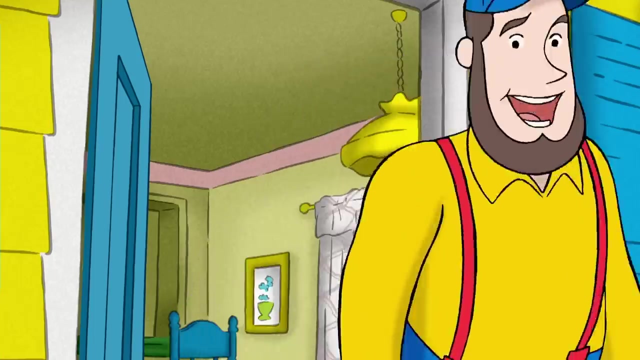 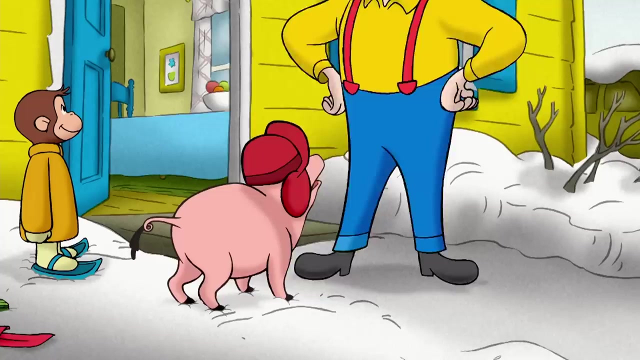 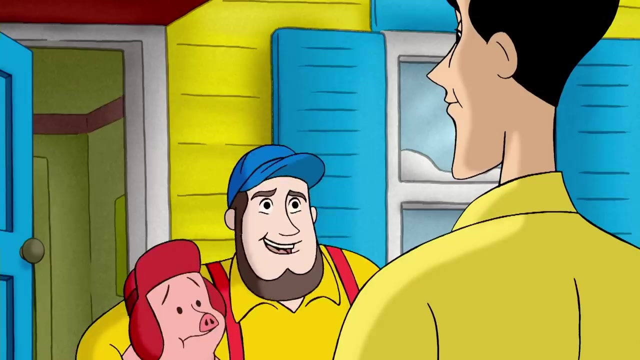 What did you do? Howie was going to get it down. What they needed was a sled. What they needed was a sled. I'd know that squeal anywhere. It's Little Mike. He got out last night before it snowed. He's never even seen snow before. 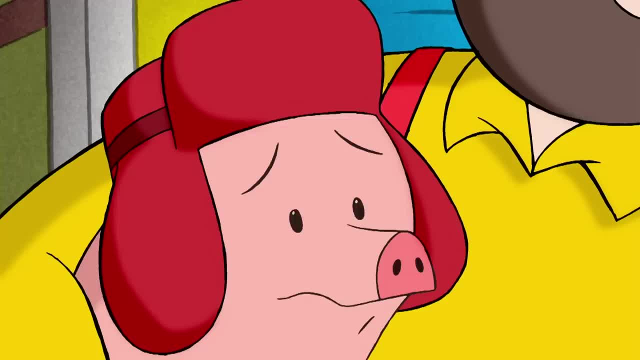 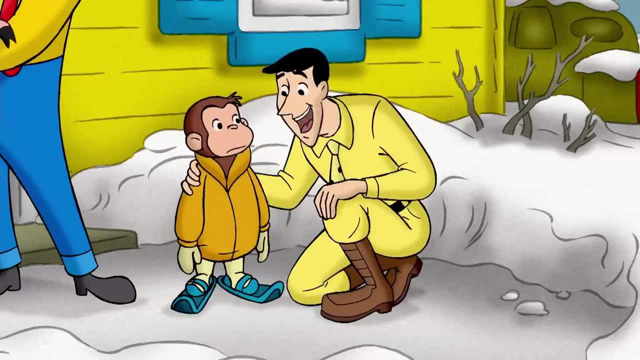 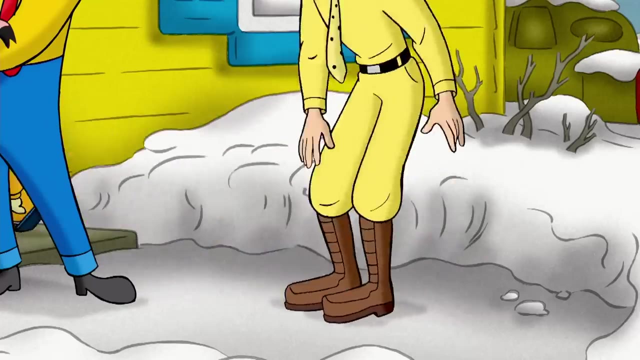 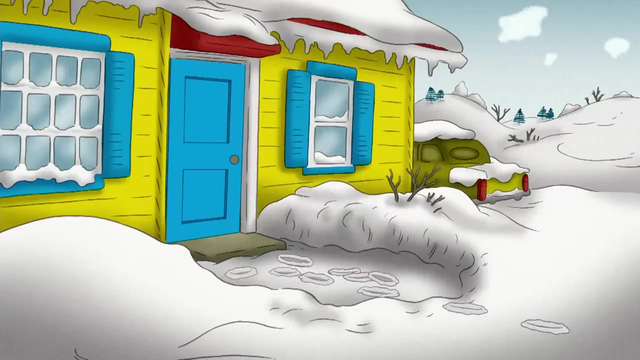 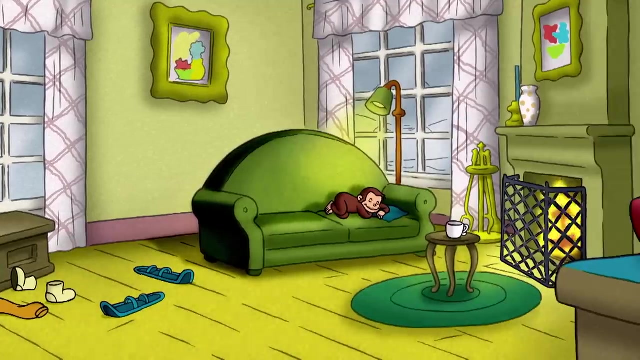 Must have been completely mystified by it. Thank you, George. I was wondering what took you so long. There's a cup of cocoa inside waiting for you. Well, see you later. Okay, take care. Skiing, sledding, boarding, bringing a pig home. 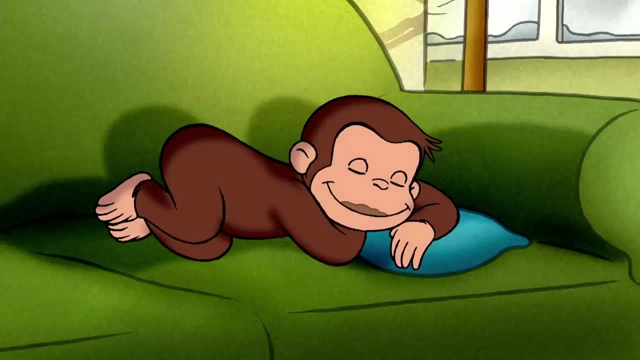 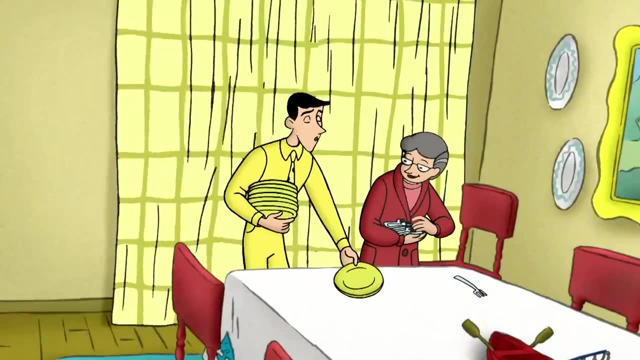 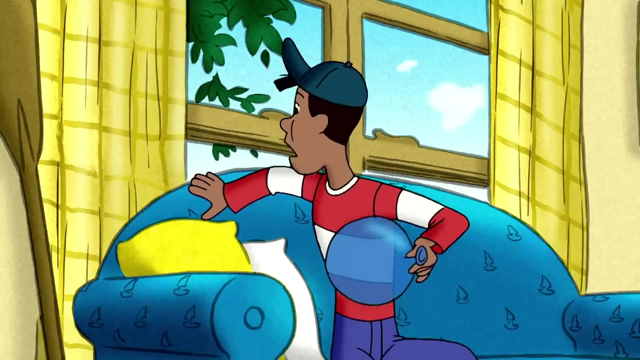 then cocoa, This was a perfect day to be a monkey. You ever thrown a surprise party for Mr Quint before? Well, it's the only way to give him a party, Because they're such a big family. Exactly, I'm watching for Mr Quint's boat. 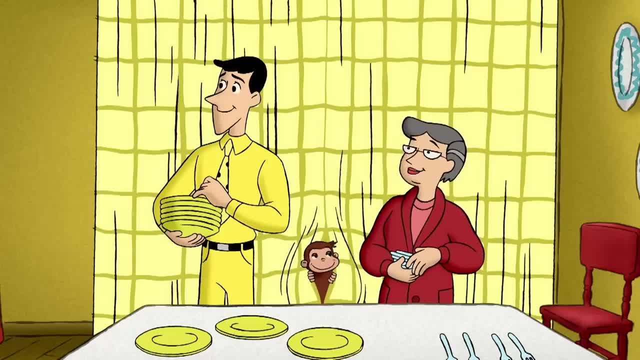 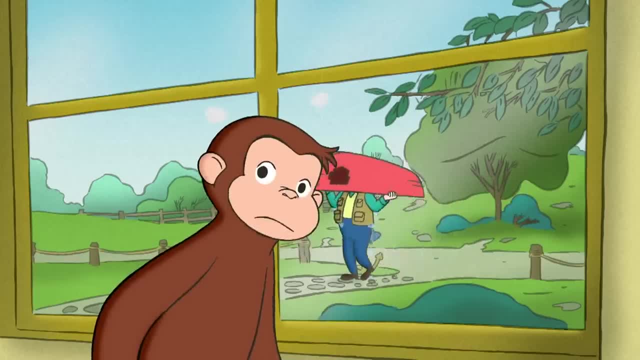 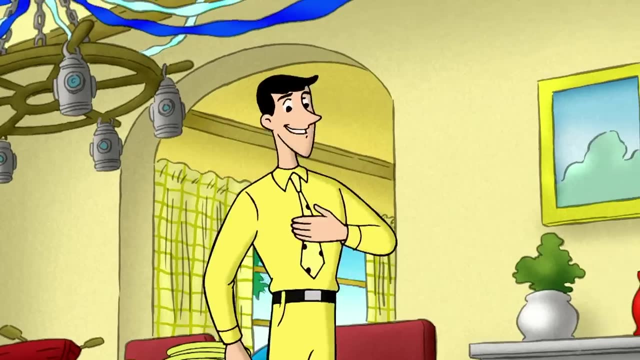 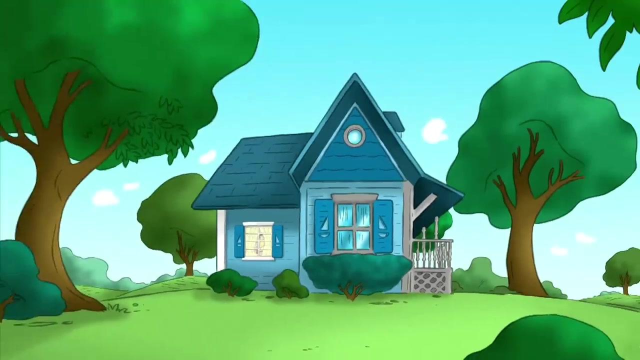 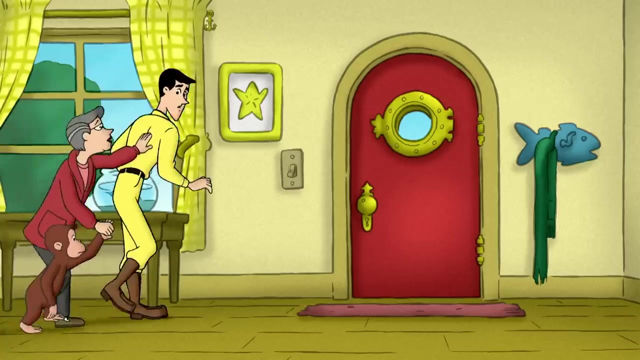 No sign of him. Oh, you don't have to watch yet, Bill. He won't be back for at least two hours. Oh, you don't have to watch yet, Bill. You can't be a badass if you don't make a crap. Oh, it's not my birthday, George. 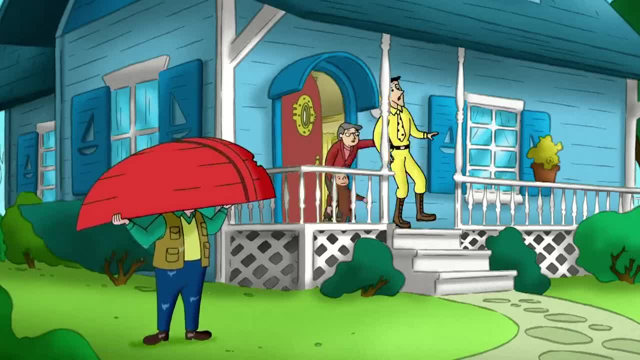 I'm not supposed to get surprised. He's home early. What do we do? Take him to your house and keep him there until party time. Drill, drill, Drill, drill, drill, drill. Now we go. Drill, Drill, drill drill. 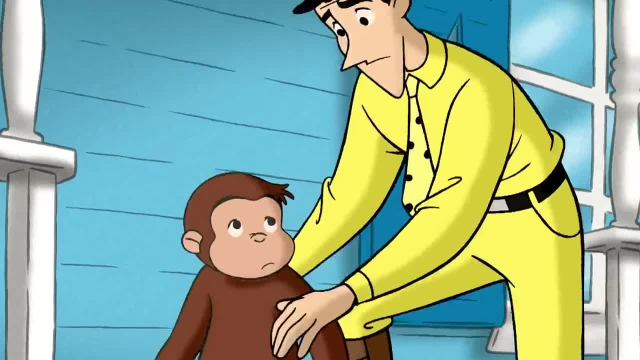 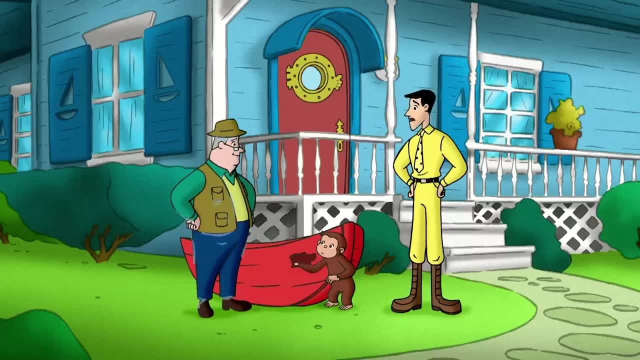 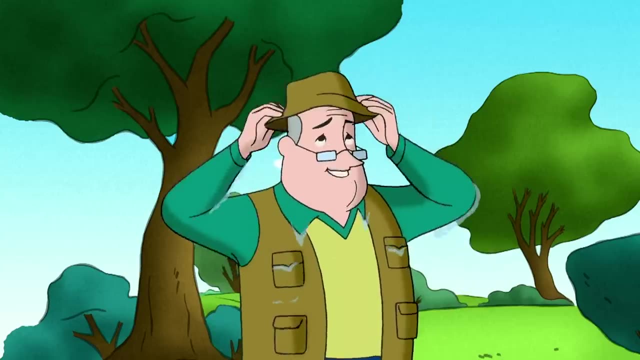 Not yet, George. Well, hey there, young fellas. Ooh, looks like you sprung a leak. Bad luck today, huh, Eh, not all bad. Got to see part of the river I never saw before- The bottom. Well, I gotta change my soggy socks. 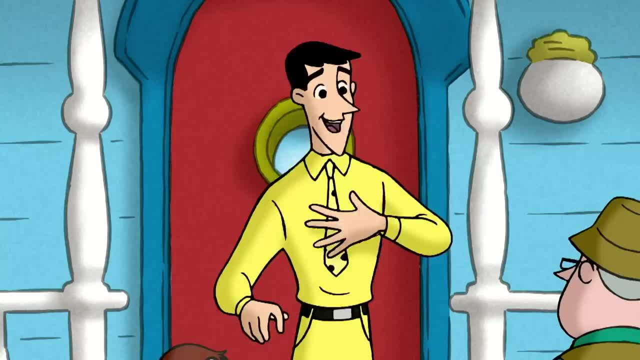 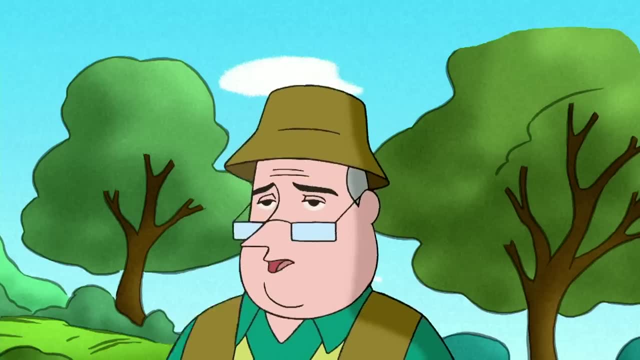 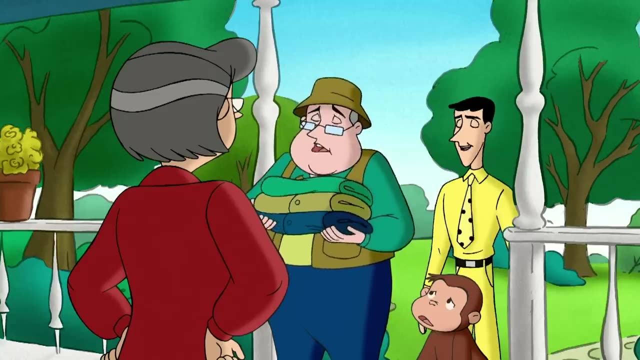 Don't? I mean, come to our house. We want to build a fish pond and need expert advice About fish. Well, sure, Let me just get some dry clothes Here. dry clothes Go help him. All right, Mother, if you say so. 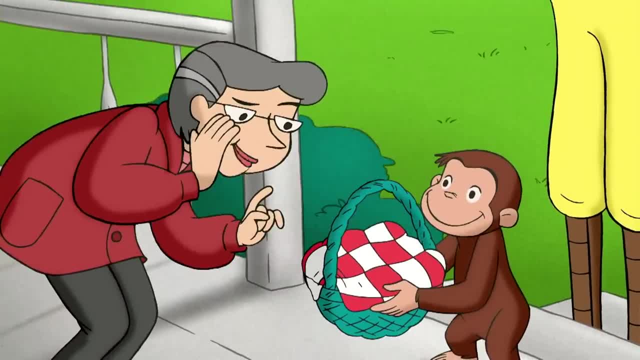 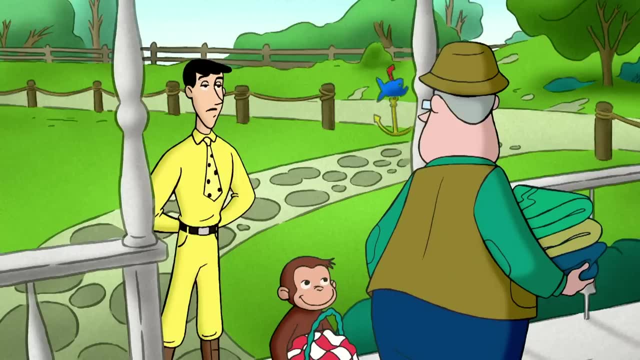 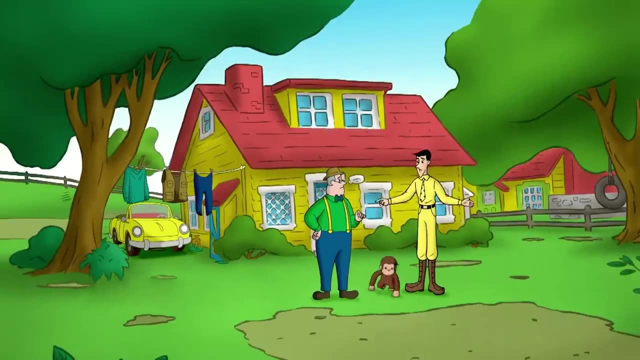 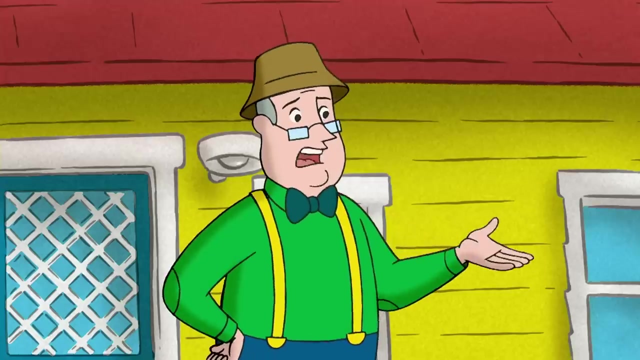 No quit can resist fish crackers. They may come in handy. Okay, goodbye, Have fun. So George and the man with the yellow hat kept Mr Quint busy with lots of questions. What do you think? Well, if you make a pond that big, you can have almost any size fish. 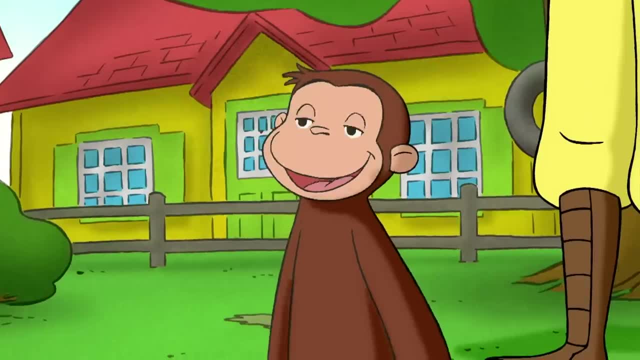 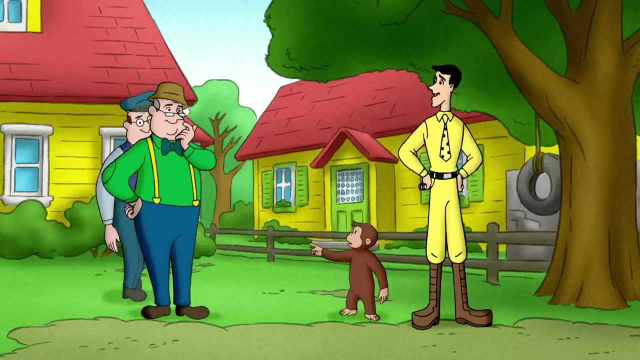 As George was about to ask exactly how many whales he could have, Mr Quint's brother, Flint Quint, showed up. Hoo, hoo, hoo, hoo hoo, Hmm, Oh, uh, hi, George, it's Mr Quint's brother, the train station master. 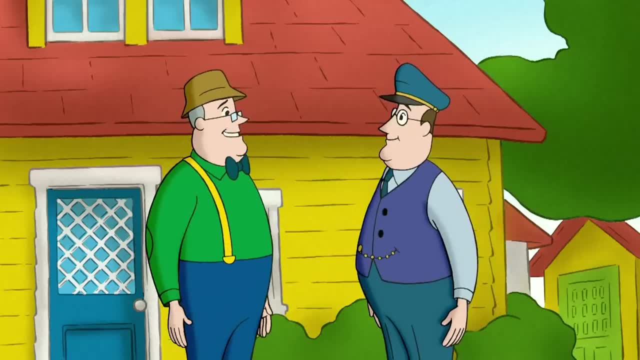 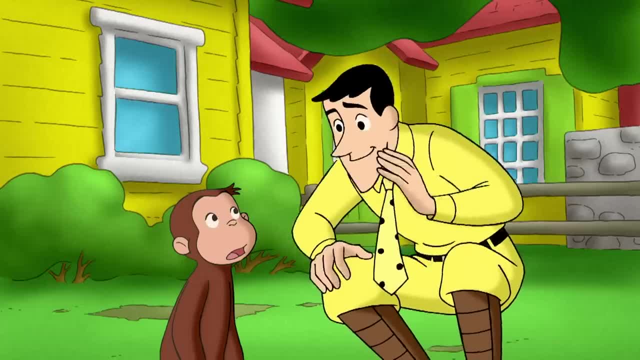 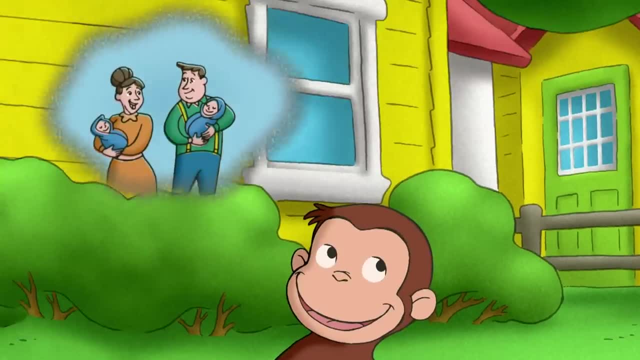 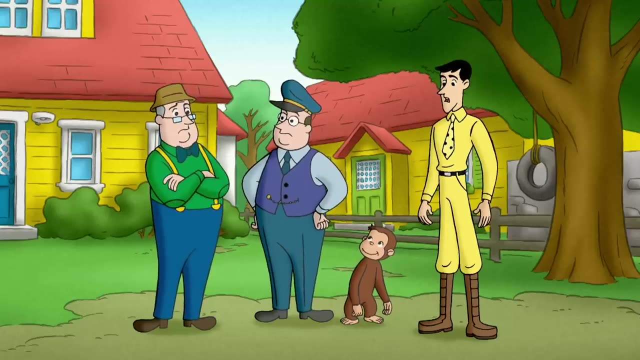 So Flint can't know about the party either. okay, The Quints were twins. Now George had two people to yell surprise at. It couldn't get any better. Yo, I said you needed help, so I came right over. Well, this here's fish business, not trains, so you can weigh anchor. 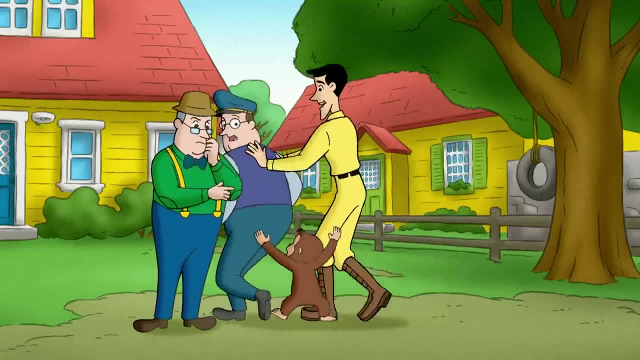 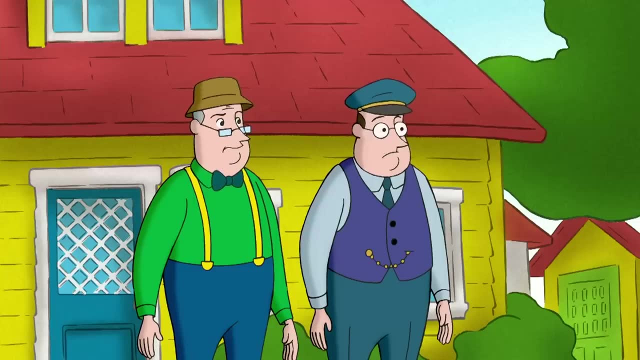 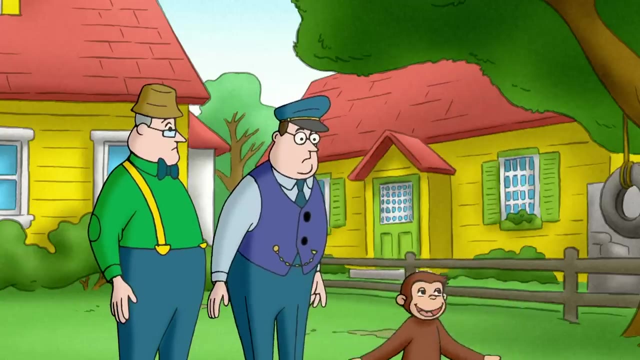 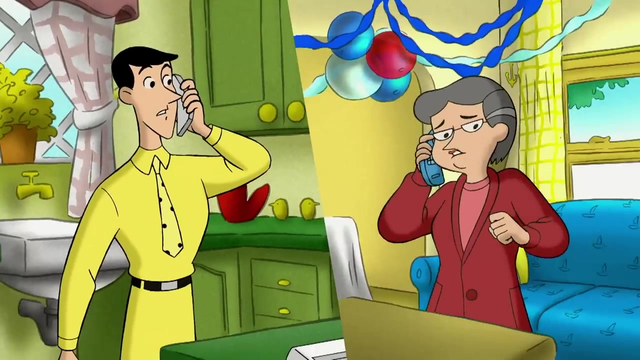 I'll meet you back at my house. Don't go. We want to know about running a train around the pond. we're planning, I'll be right back. Hello, Oh, it's Mrs Quint. Disaster: The bakery truck broke down so they can't deliver the birthday cake. 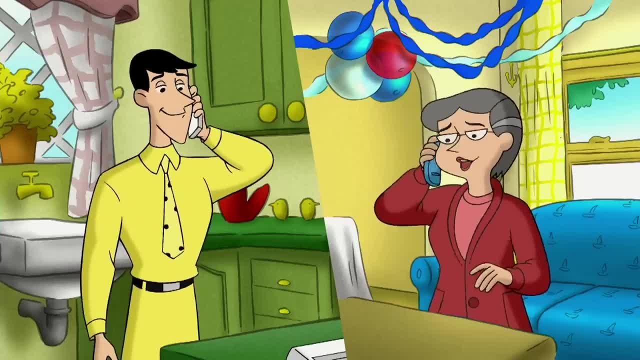 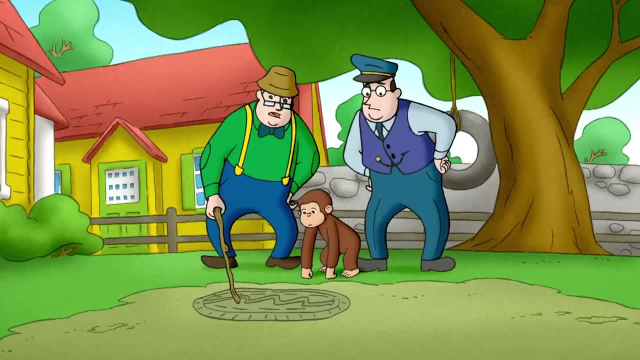 Don't worry, I can go pick it up. Oh, thank you, It's at Mr Piscato's Bakery over in Franklin Square. You can't run tracks across the pond, It'll scare the fish. Well then, we'll just have to tunnel. 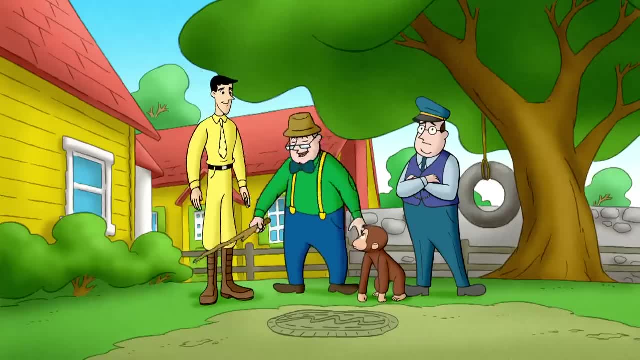 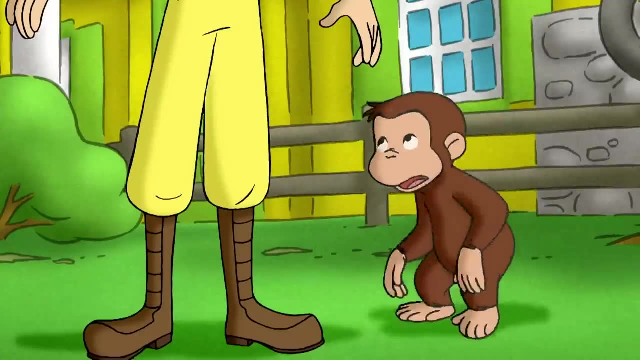 Guys, could you, monkey, sit for me while I run an errand? Sure, We'll just figure out the pond while you're gone. Hoo hoo, ha, ha. ha ha, George, it's your job to keep the Quints here, so the surprise isn't wrecked, okay. 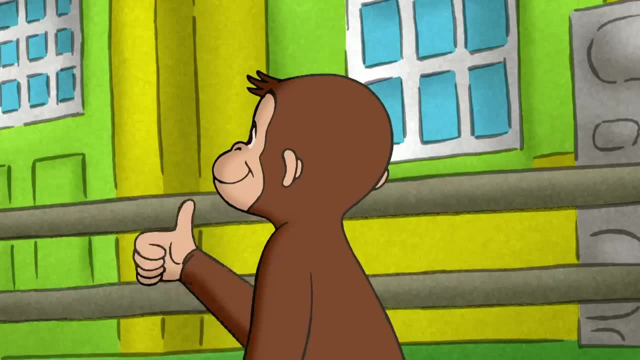 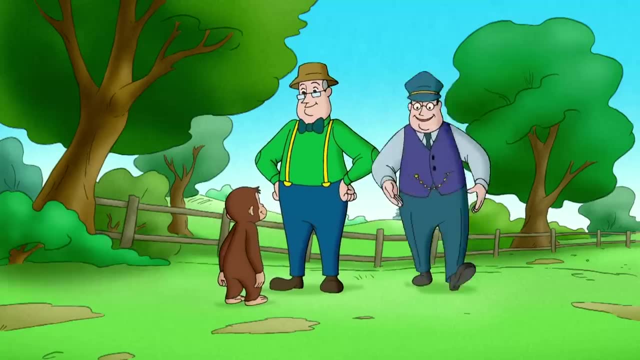 Ah, Ha, ha, ha, ha ha ha. George knew this would be easy, because the Quint brothers would probably argue about the pond for hours. Well, we've got it all worked out: The perfect pond and train. Oh, ha, ha, ha, ha ha. 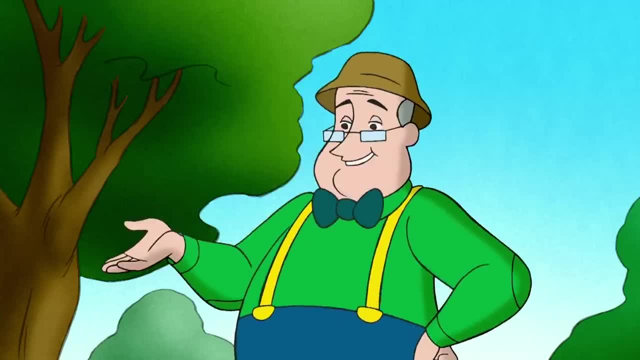 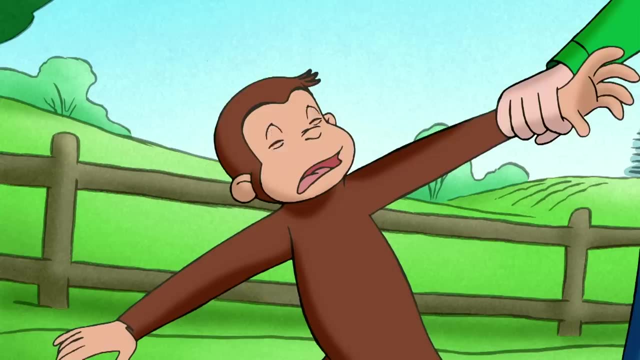 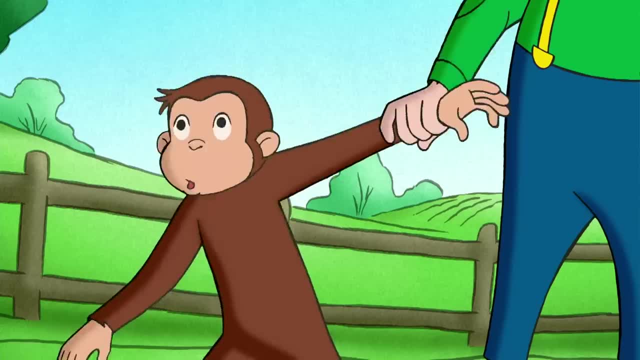 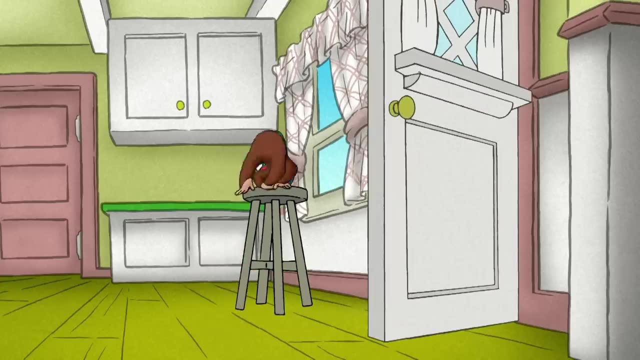 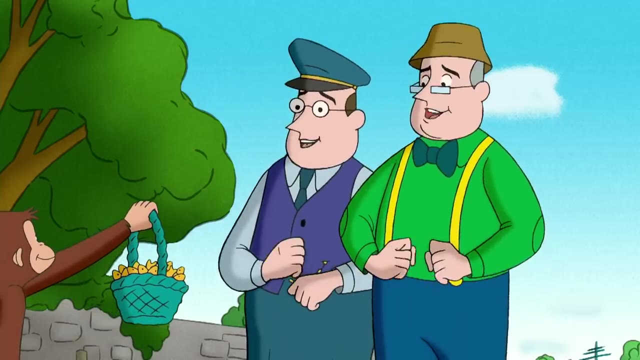 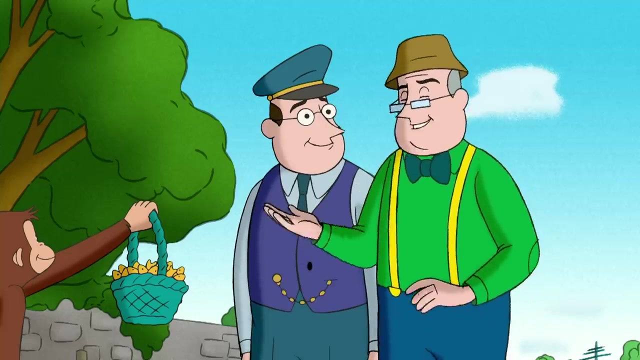 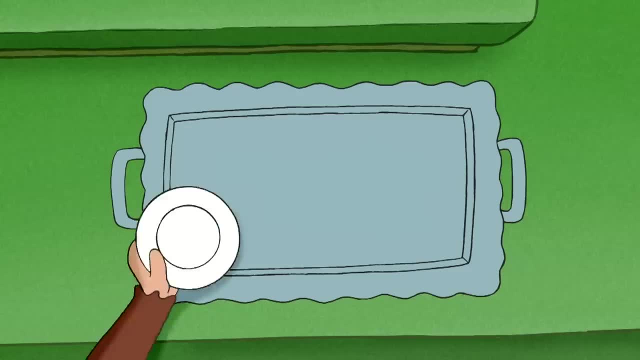 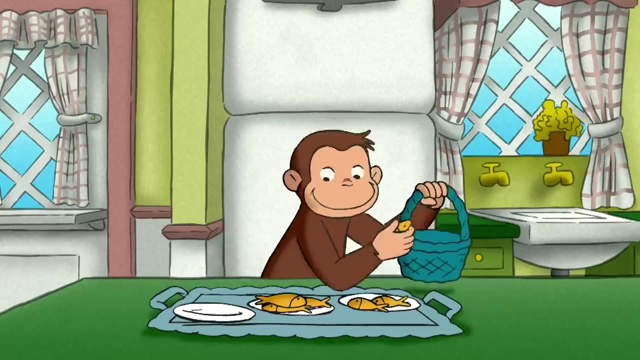 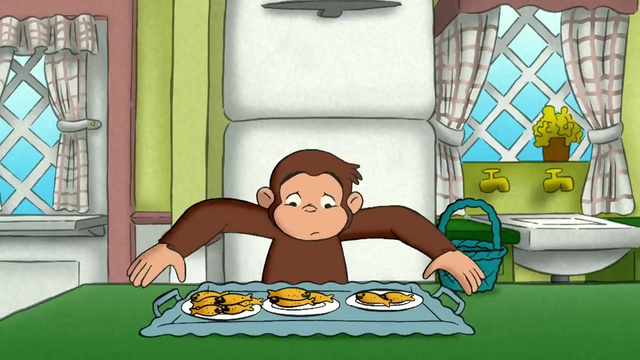 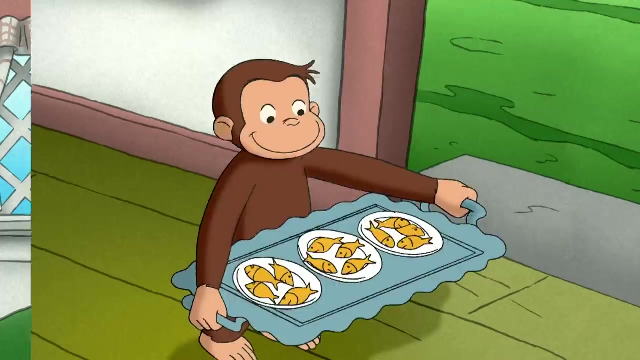 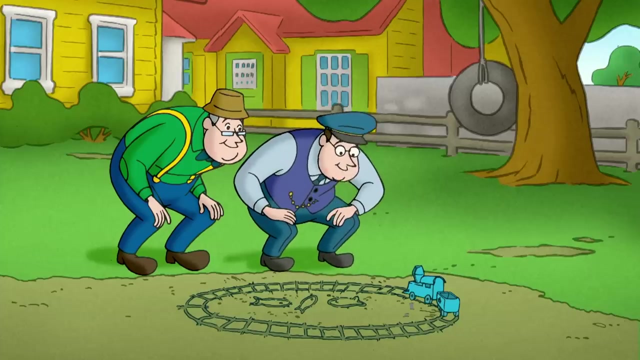 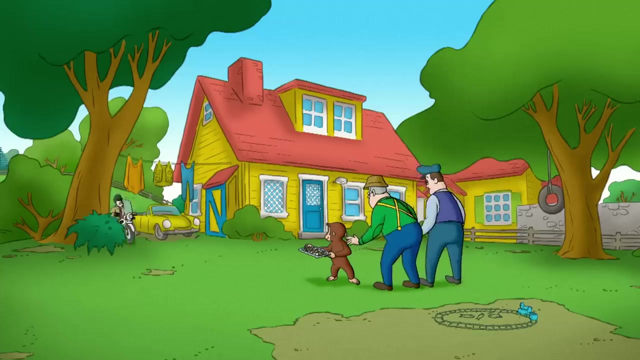 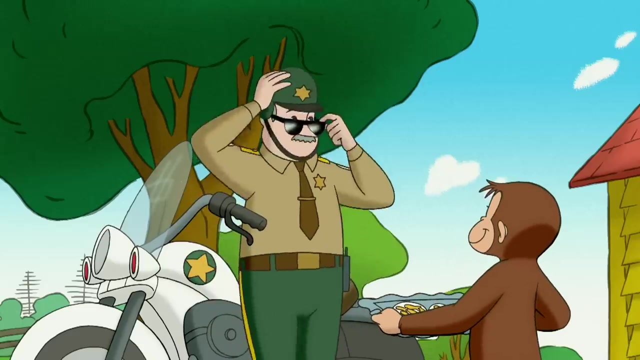 That's a good idea. Eating this many crackers would keep the quince here a long time. Somehow this didn't look fair. Fish food can arrive by train at ten o'clock and three o'clock. Those look delicious. Whee. My brother's wife requested I proceed here to provide backup. 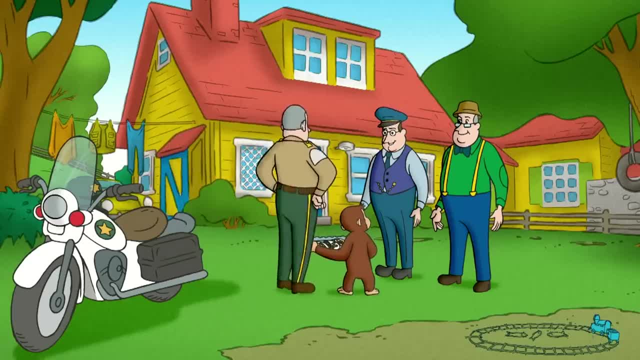 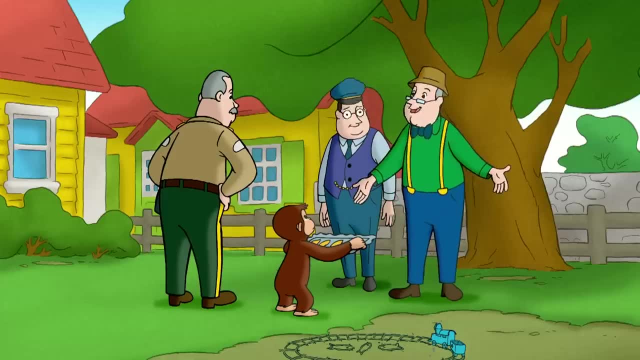 Hey Clint, Happy birthday. Hey Flint, Happy birthday. Hey Wint, Happy birthday. Oh, didn't you know, George, All us quince were born together. Of course, I'm the oldest By two minutes. 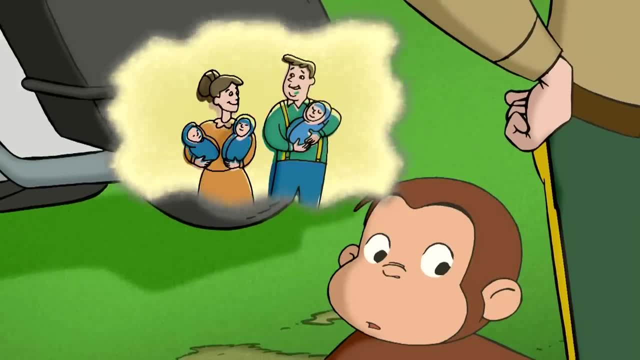 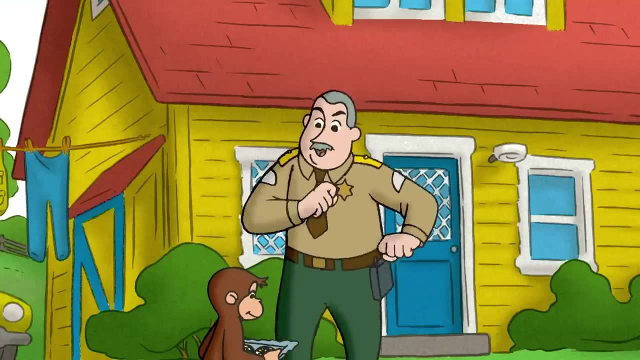 The quince were triplets. Now, George had three people to yell surprise at: Ah, Even better, Fish crackers. Ooh, ooh, ooh. Well then, you hawks, we were here first, Huh. 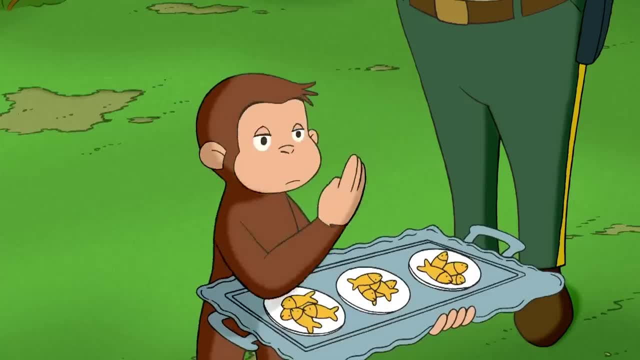 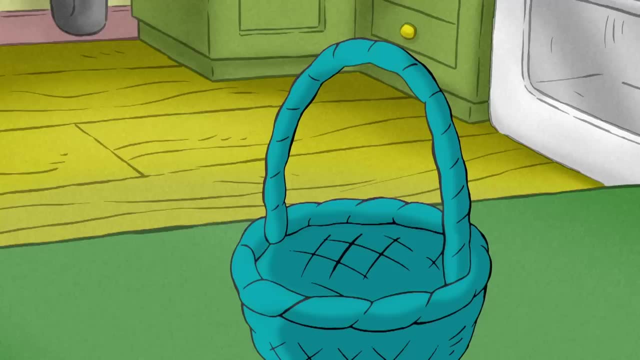 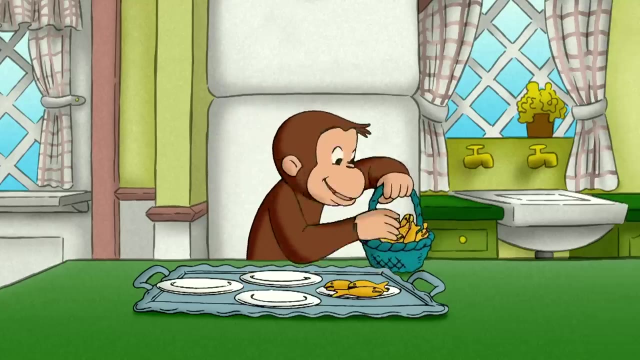 Huh, Huh, Huh. George was gonna need another plate to keep three whole quince here. Ha-ha-ha, Ha-ha-ha, Ha-ha-ha, Ha-ha-ha, Ha-ha-ha. 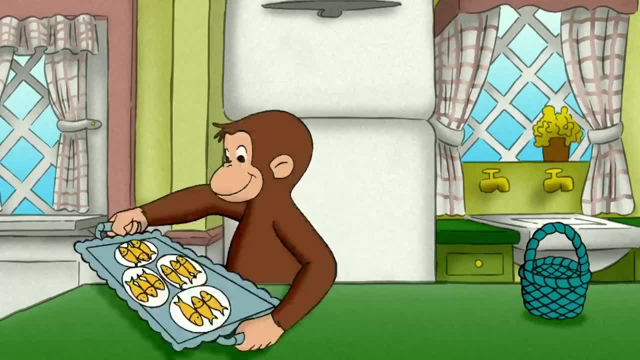 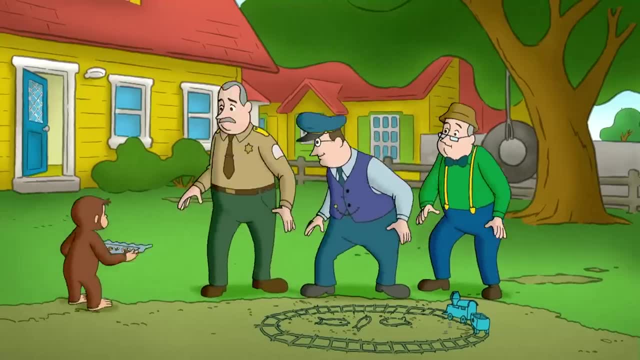 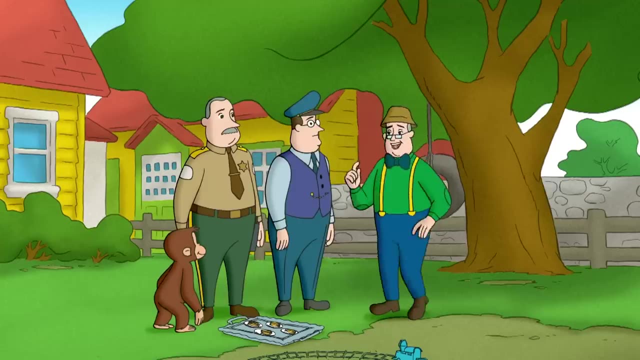 Huh, Huh, Huh. Nice, But where's the police boat? Hoo-hoo, Ha-ha-ha-ha, Ha-ha. Hey, I've got juice at home that goes great with fish crackers. Let's eat these at my house. 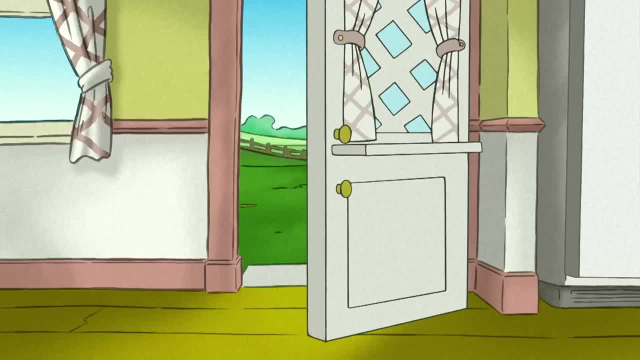 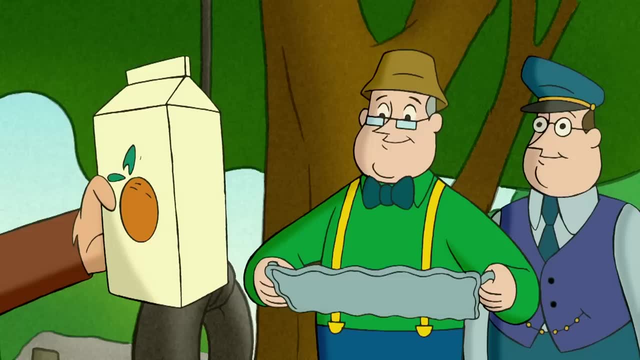 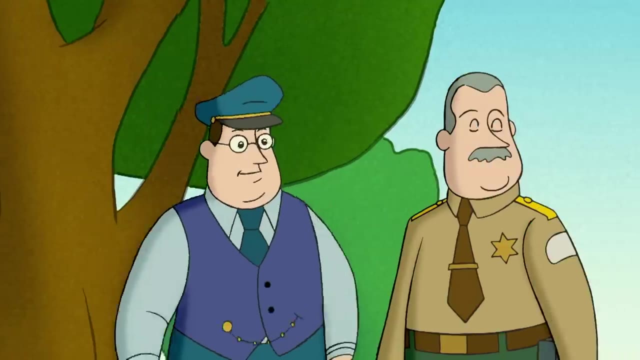 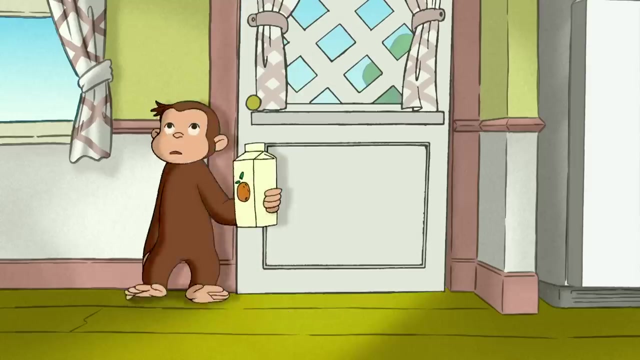 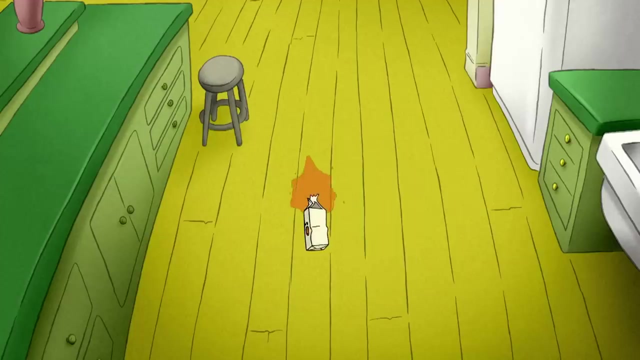 Ha-ha-ha, George. Well, that's the same juice. OK, we'll stay here, so we don't have to wait for fish crackers. Fish crackers, Ooh, ooh, ooh, Phew Yay. 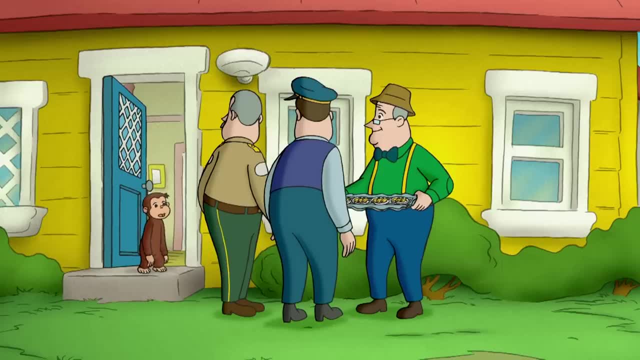 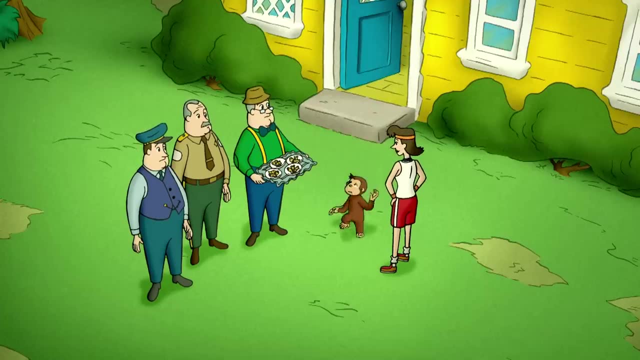 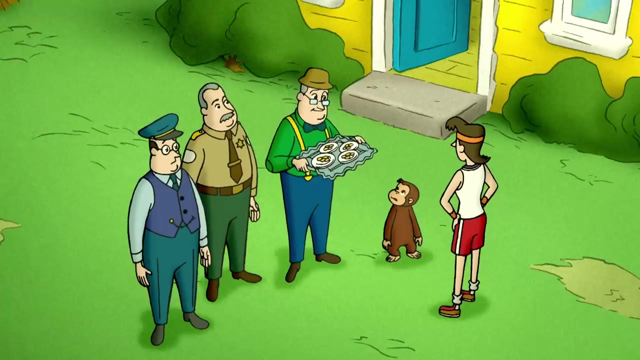 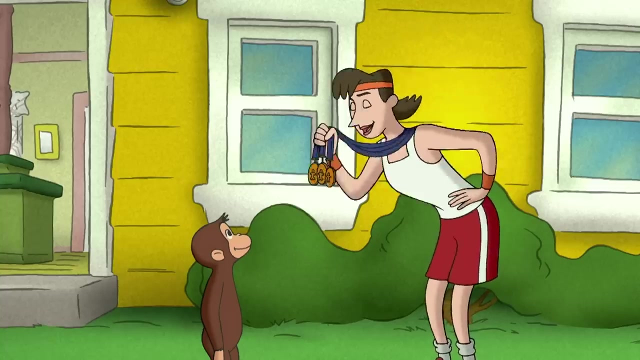 George had to admit he had no juice. Happy birthday boys, Happy birthday George. meet our sister, Sprint Quint, the track star. She won three Olympic gold medals. Aw pshaw, That was long ago. Count them Three. 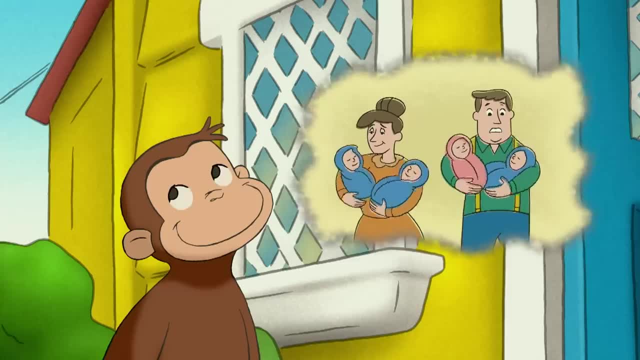 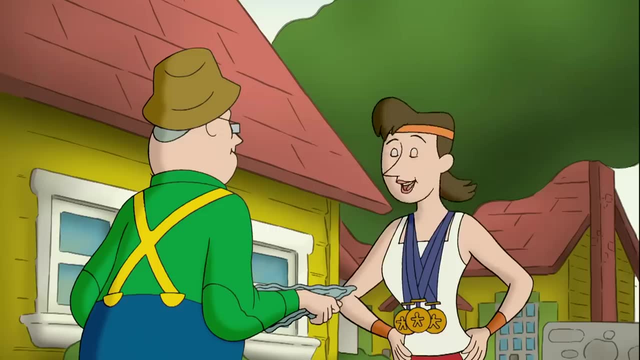 The Quints were quadruplets. Now George had four people to yell surprise at. This was the best. So I hear you need help putting a jogging track around a pump. Are those fish crackers? Ooh, ooh, ooh. 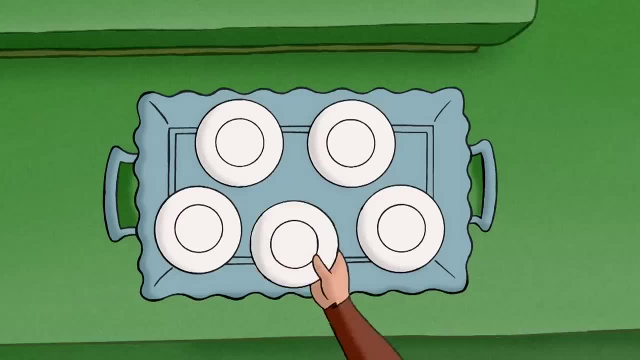 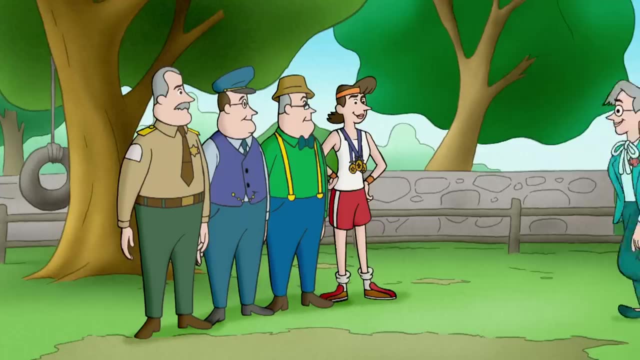 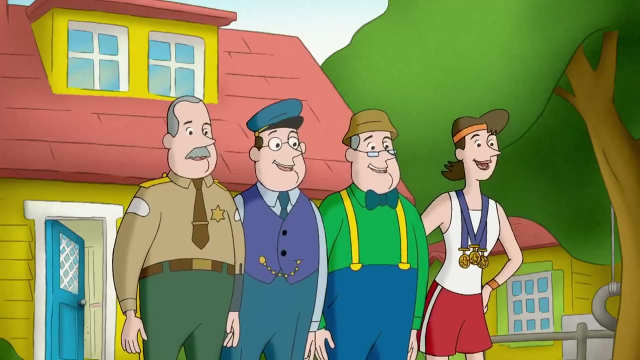 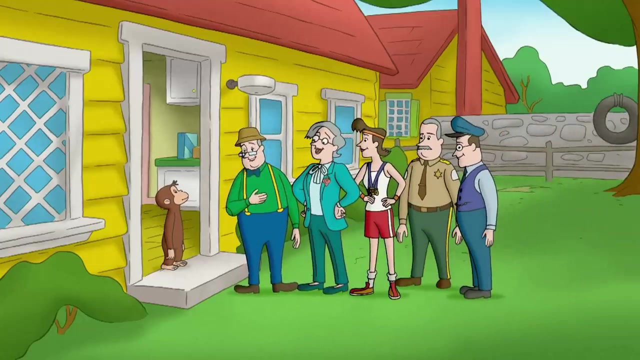 Ha, ha, ha ha. But before he even tried to split twelve crackers onto five plates, another Quint showed up: Flint Clint, Wint, Sprint. happy birthday, Happy birthday George. meet our sister Mint Quint. She prints money for the government. 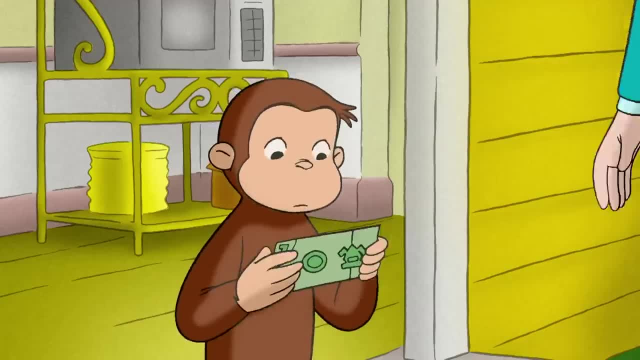 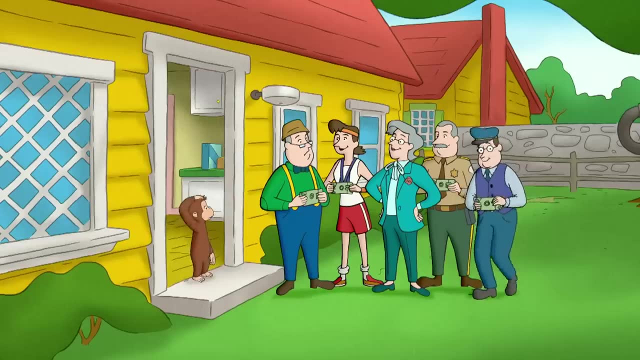 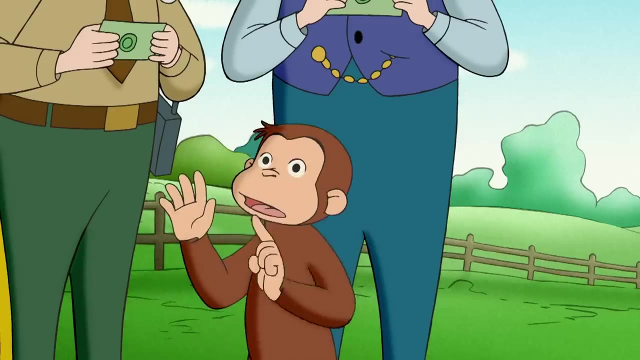 Want samples of my latest work. So I hear you need help figuring out the cost of a pond. Ha ha, ha, ha, Huh, Huh, Huh, Huh, Huh Five. Oh yeah, that's right. 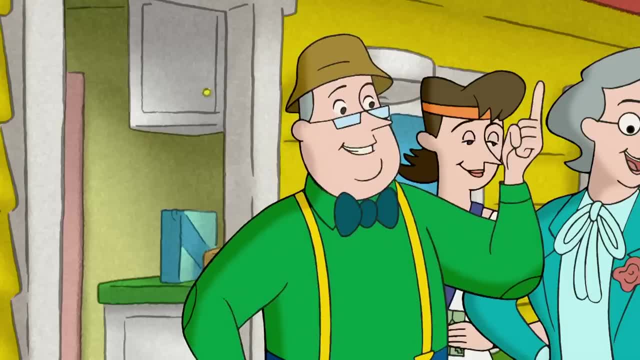 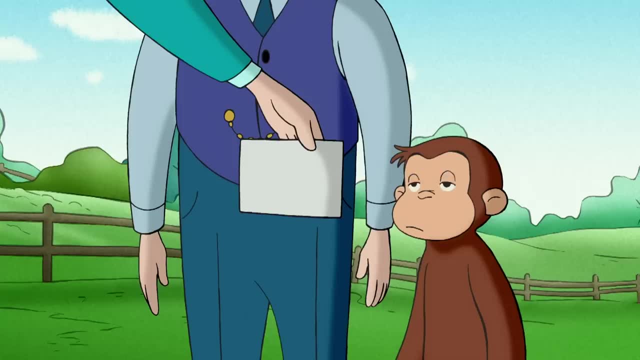 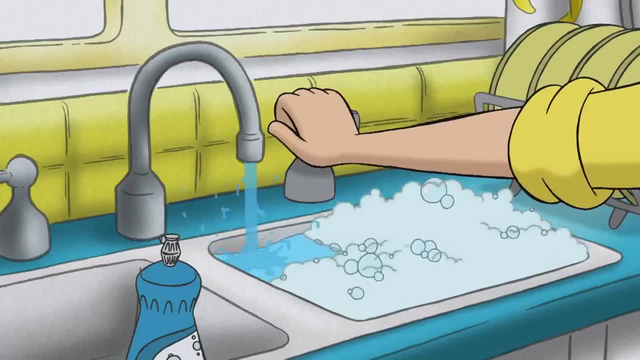 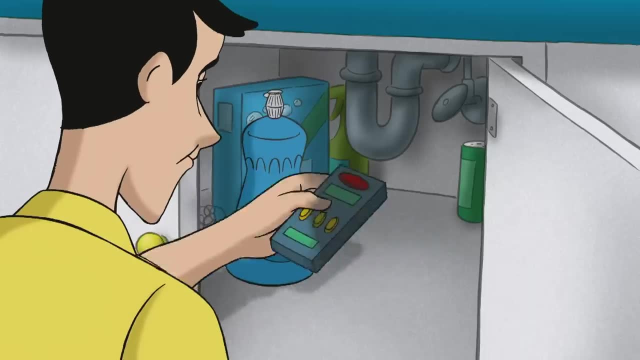 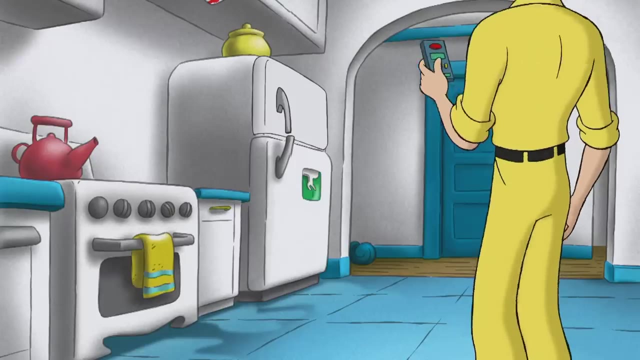 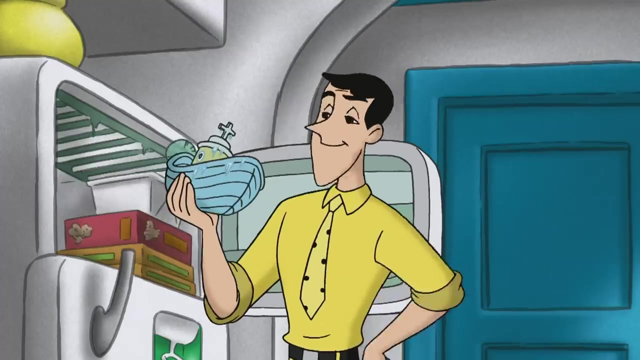 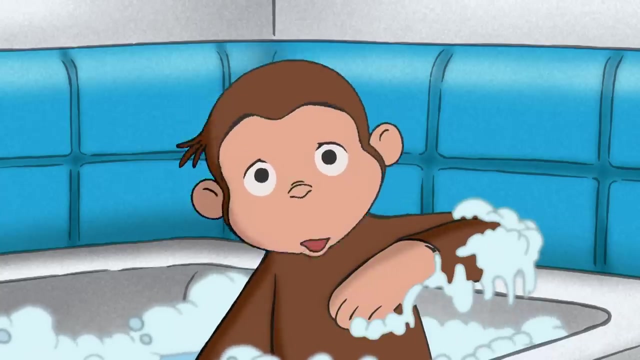 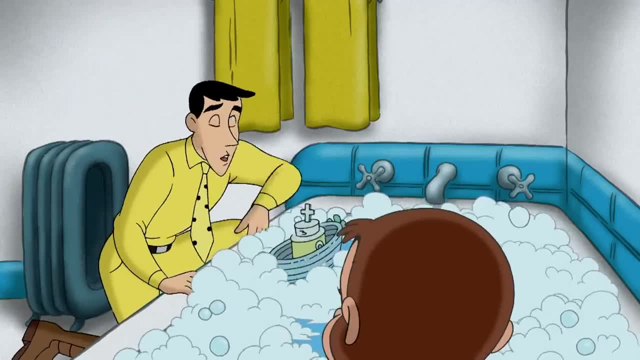 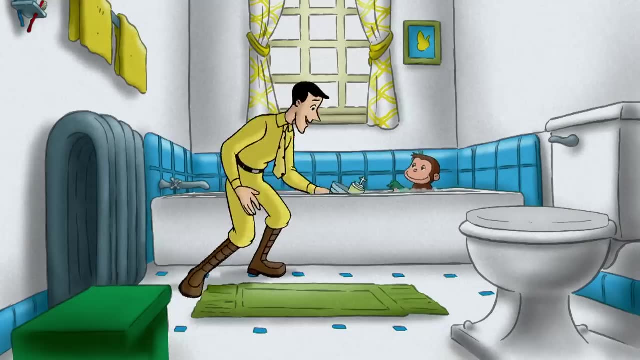 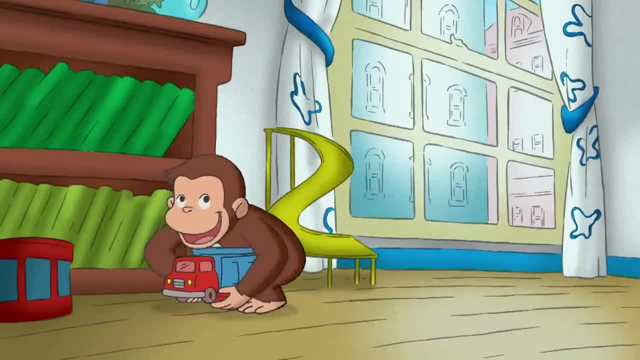 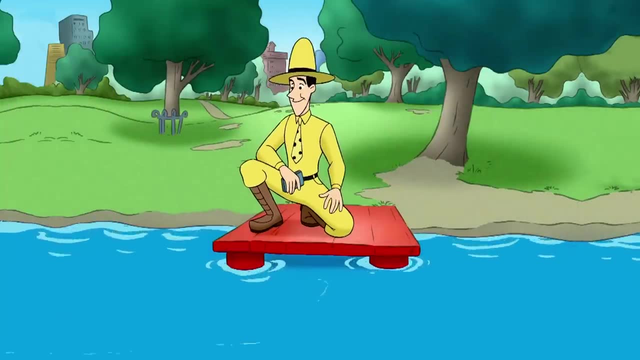 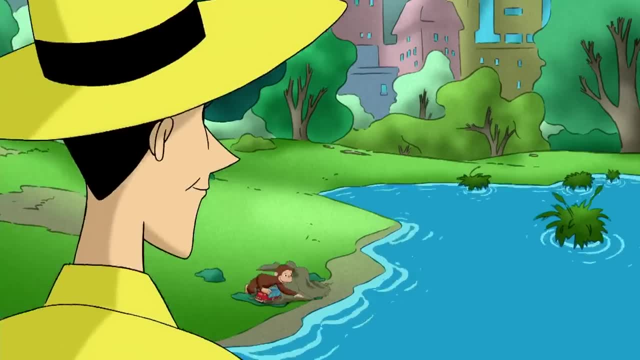 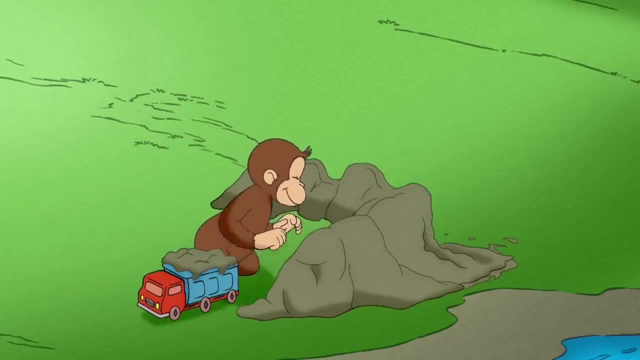 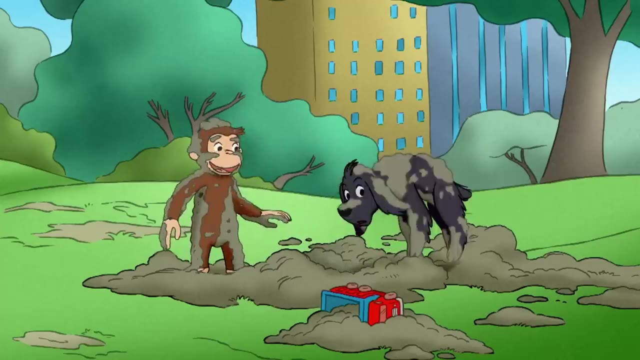 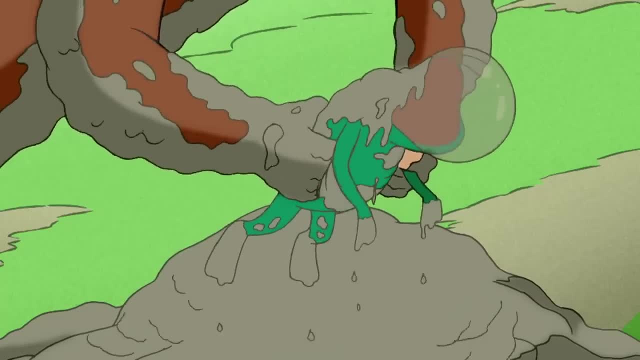 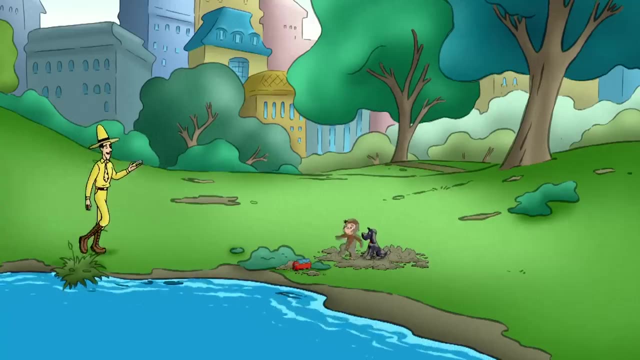 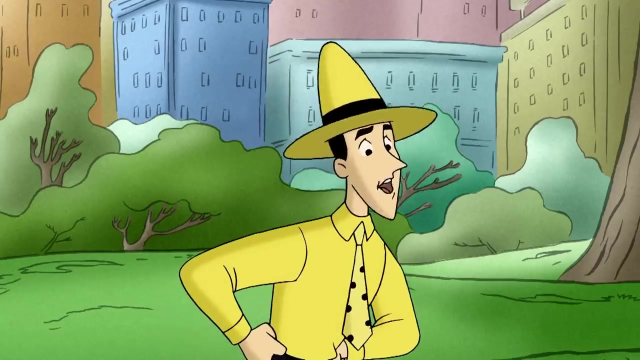 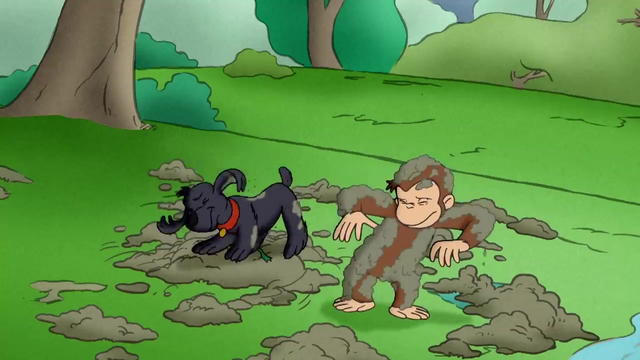 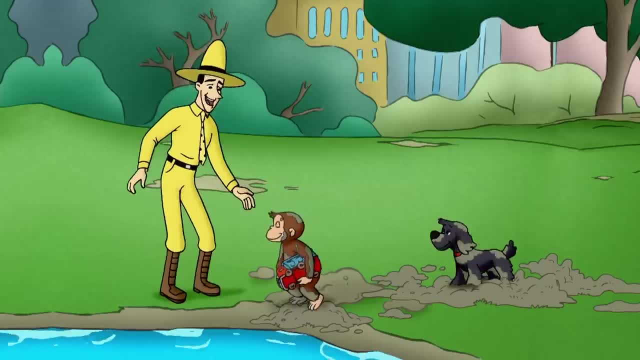 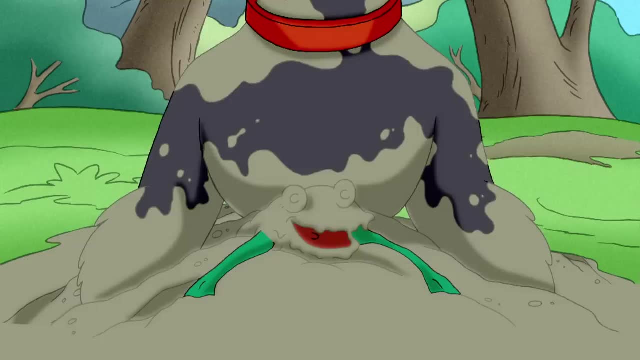 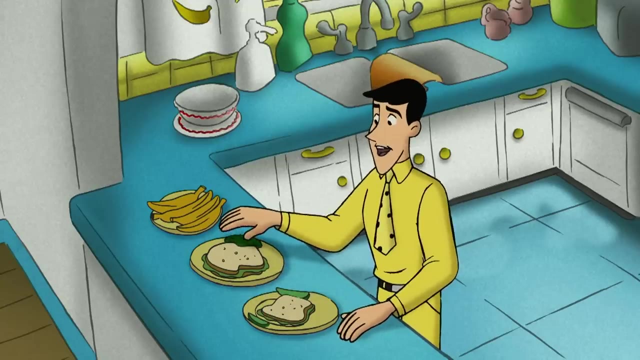 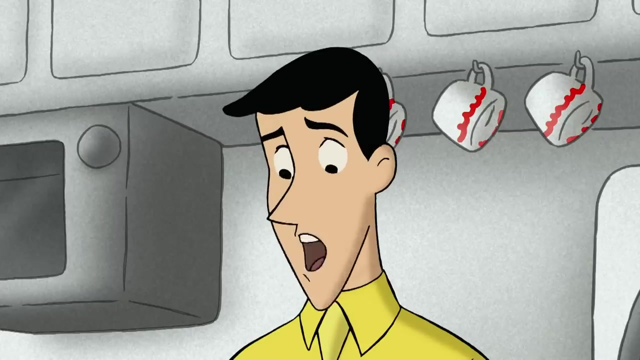 We could be here all day doing this. You can clean up at home, George. Okay, George, lunch is Ready. George, you have to get cleaned up before you can eat. Just take a quick bath, I'll wait, Okay. 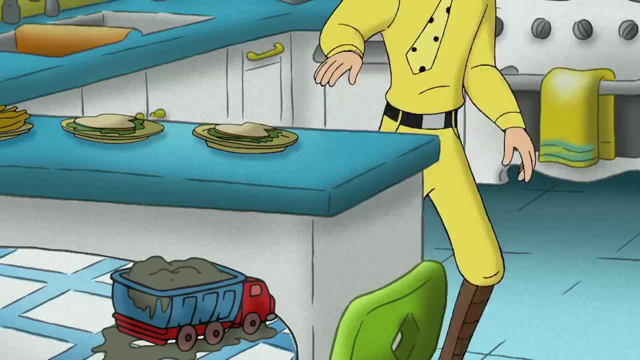 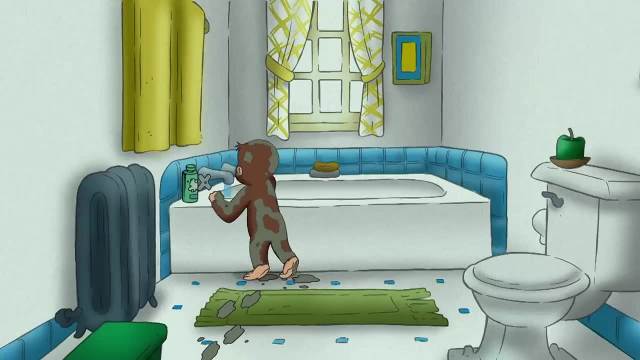 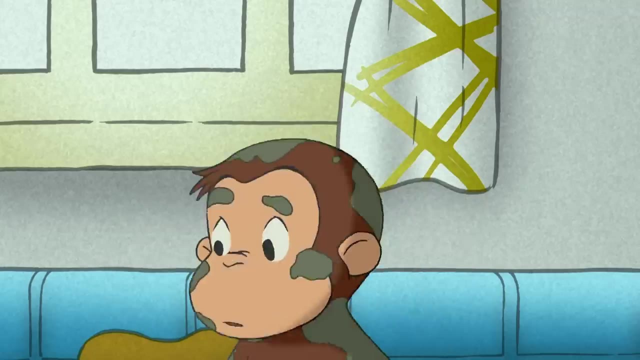 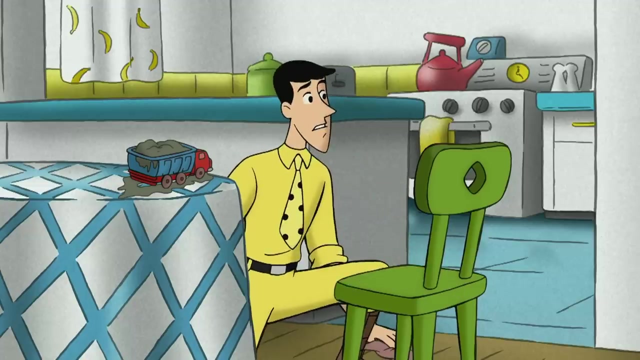 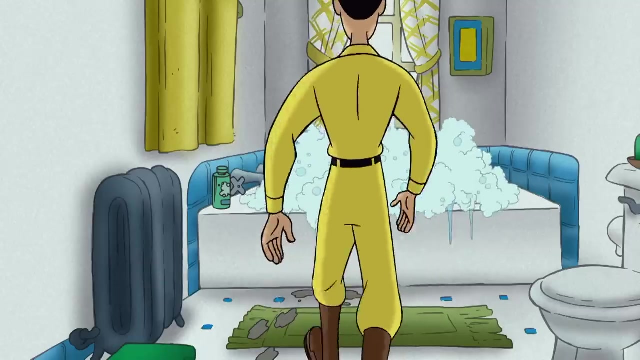 Okay, Okay, Okay, Okay, Okay Okay. There were only two things that could get George to take a bath: Bubbles and And Springy the frog. George wondered where he could be. George, George, what is taking so long? 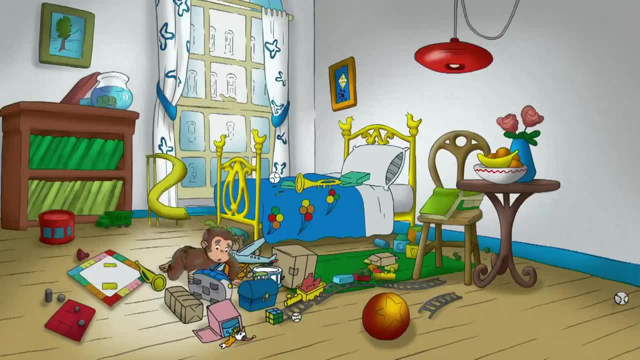 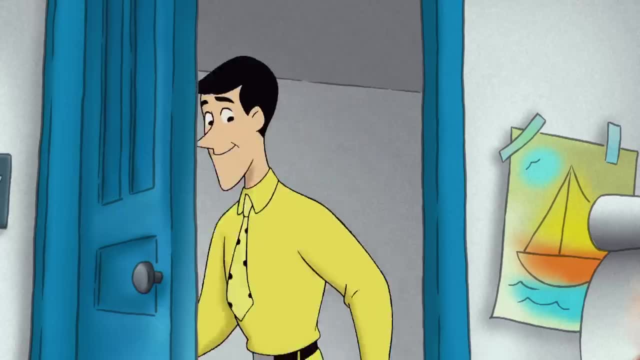 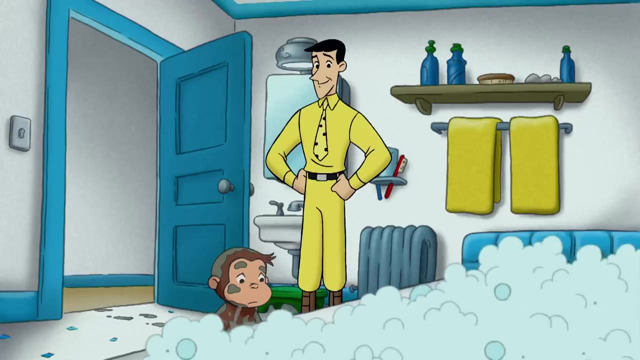 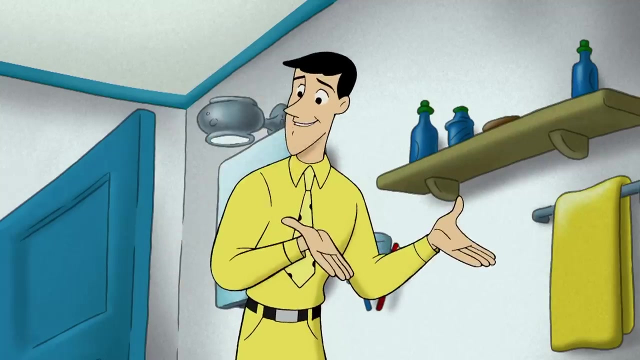 Oh, You can clean your room later. after you clean yourself and after we eat lunch, Hop in. Oh, I get it. You want to be launched like a new ship? huh, All right, here we go Into the sea. 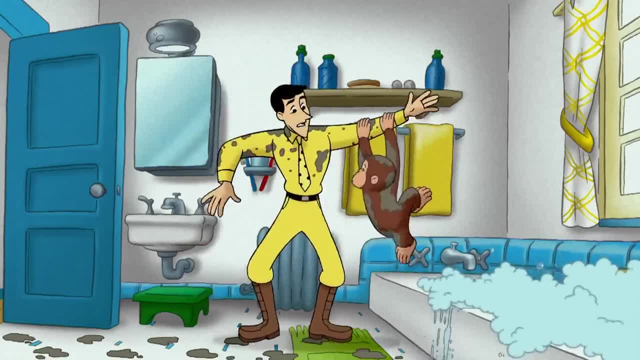 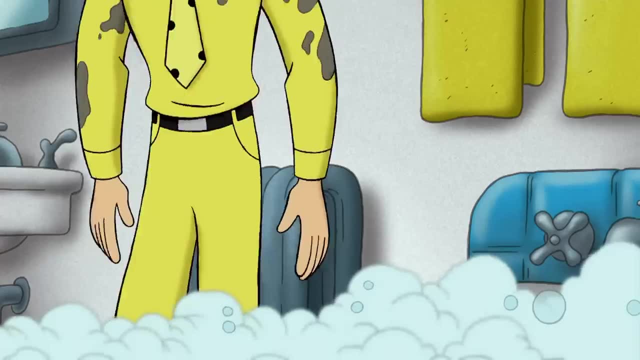 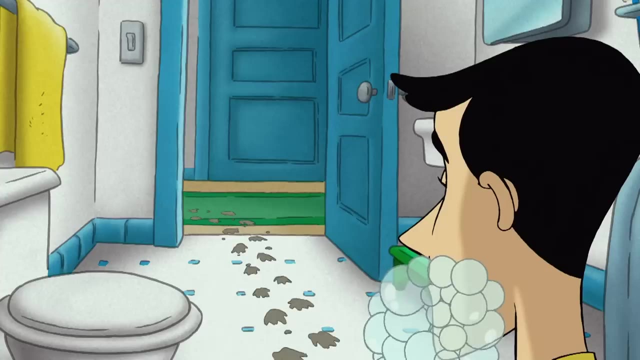 Oh, you're tickling me. Look, I know you took a bath already this morning, but you're muddy, George. Hey, look at all the fun bubbles, See. There was no way George could take a bath without Sproingy, who had to be around here somewhere. 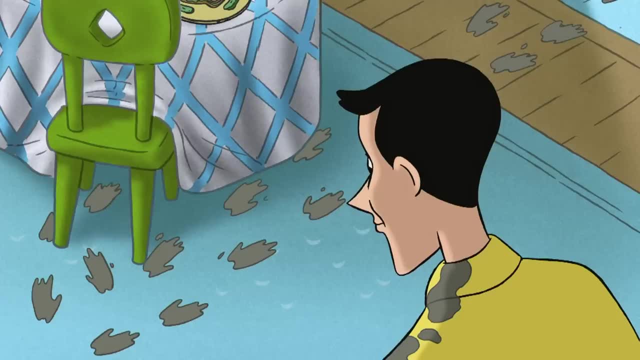 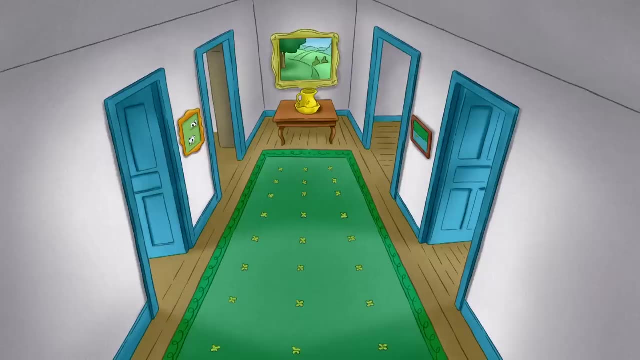 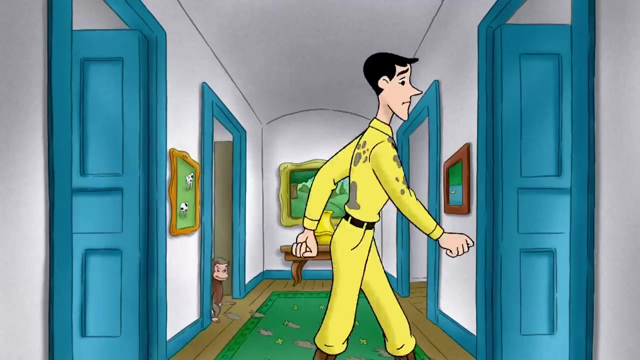 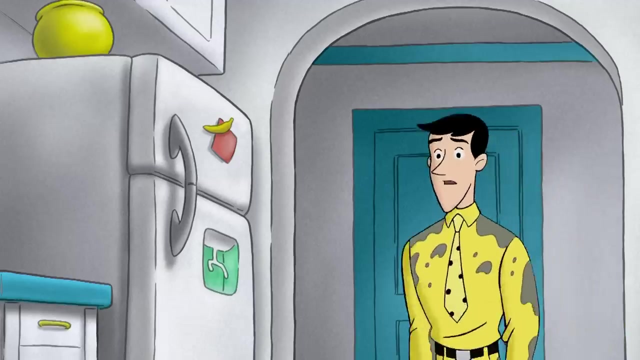 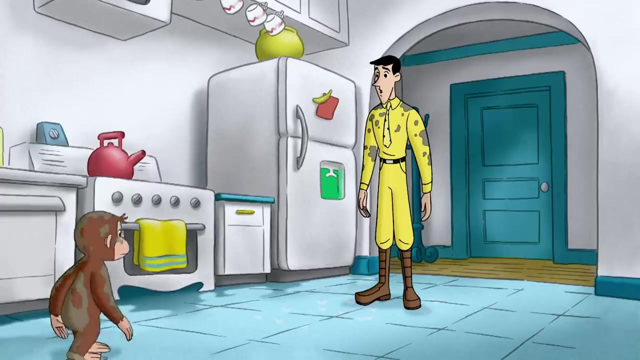 George. Oh, And there was no way George was going to admit he lost another toy who had to be here somewhere. George, George, George, George, Aren't you going to take a bath? Uh-uh, Are you going to take a bath tonight? 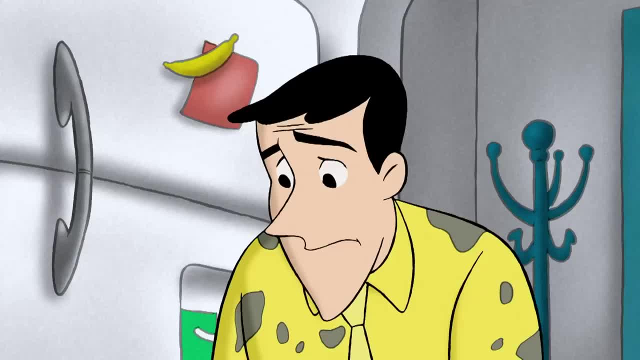 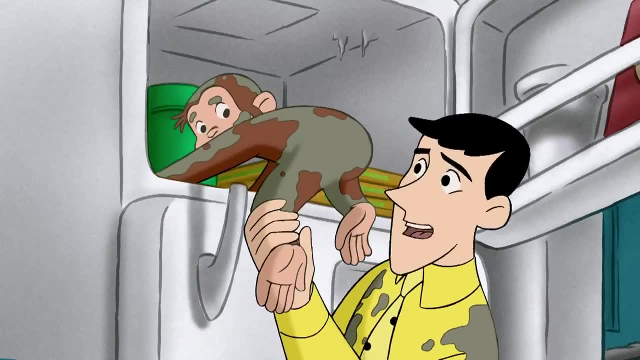 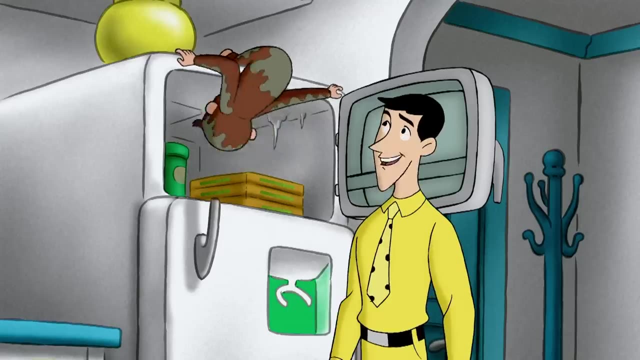 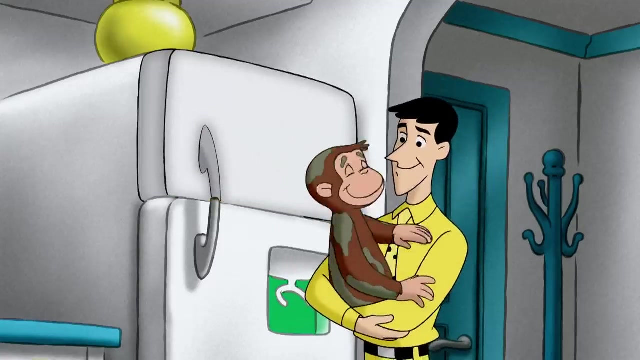 You don't know Tomorrow Ever. Oh well, I can't have a muddy monkey messing up the apartment. Okay, George, forget about giving yourself a bath. How about we give your truck a bath? Huh, You don't mind if I wash my car while you wash your truck, do you? 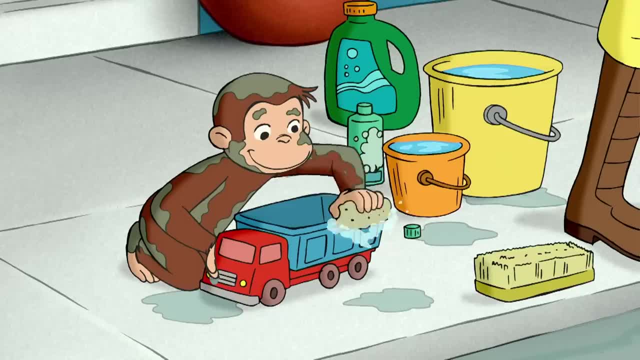 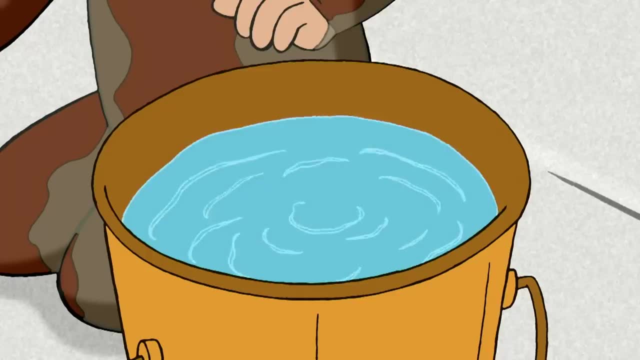 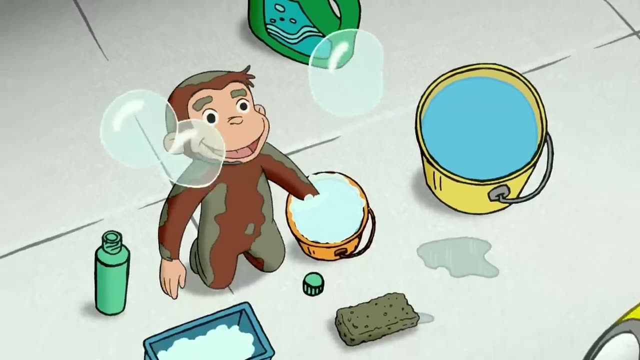 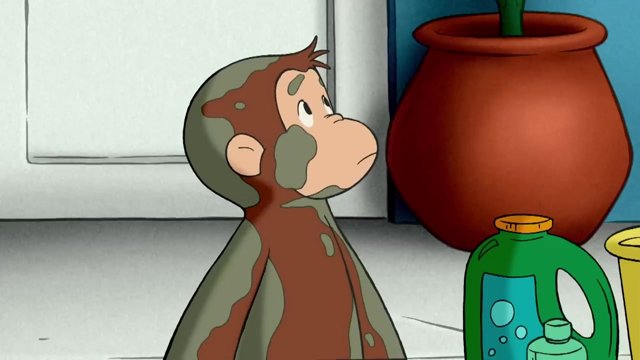 Uh-uh, George loved making bubbles anywhere. He didn't need a tub, A bucket of water and a little soap worked too. They were so light and shining and filled with air. But making bubbles reminded him of the world. It was the time of springy. 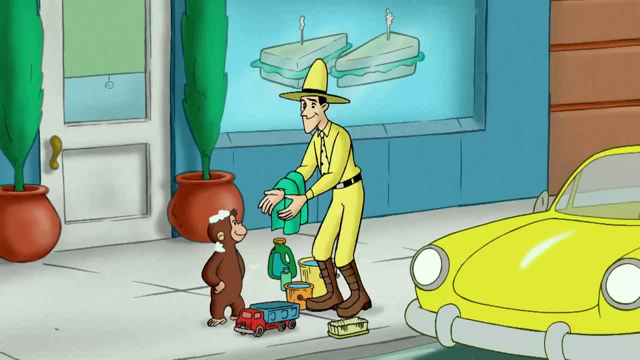 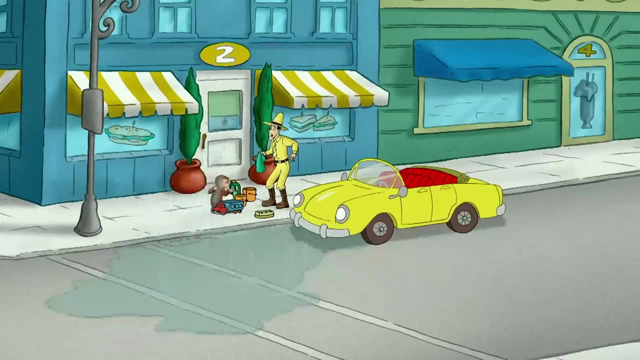 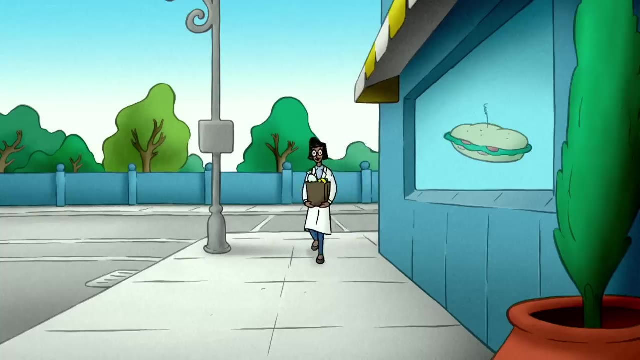 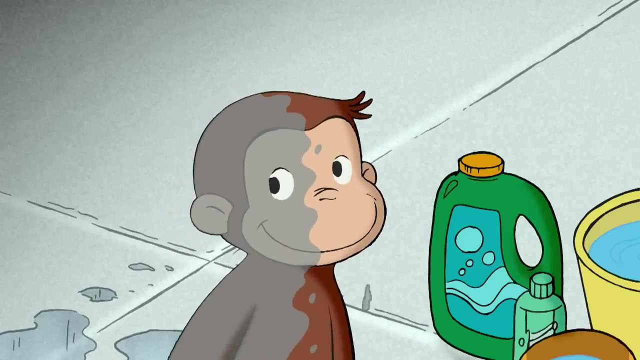 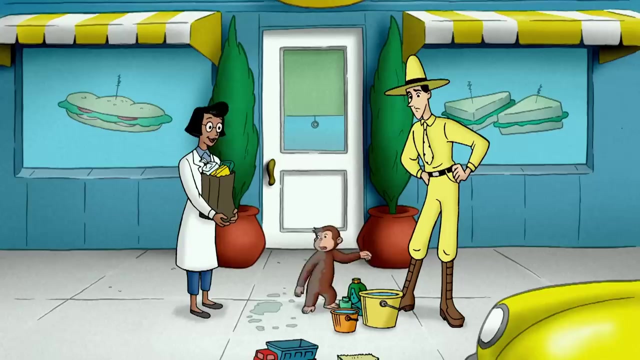 There All clean. Good job, Hi guys. Oh, you're looking good, George, Hmm, Hmm. Well, at least the right half of you is Oh-ho, Ah-ha, I guess someone's due for half a bath. 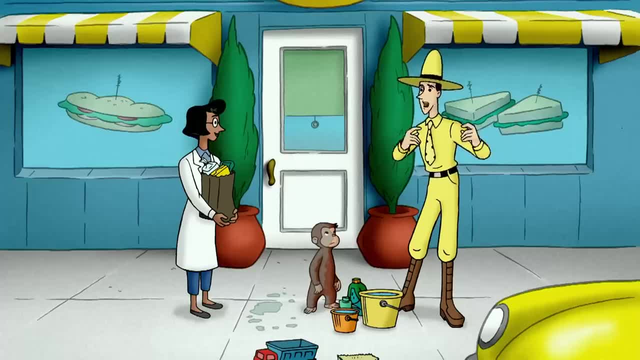 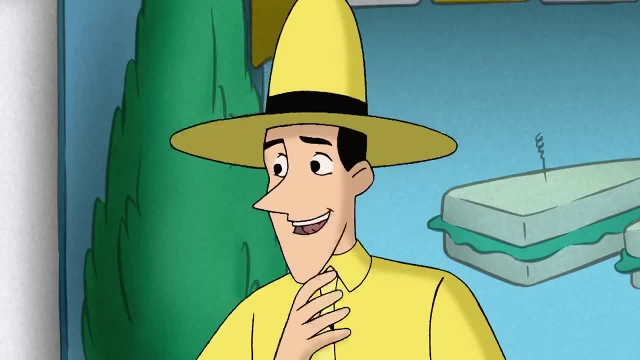 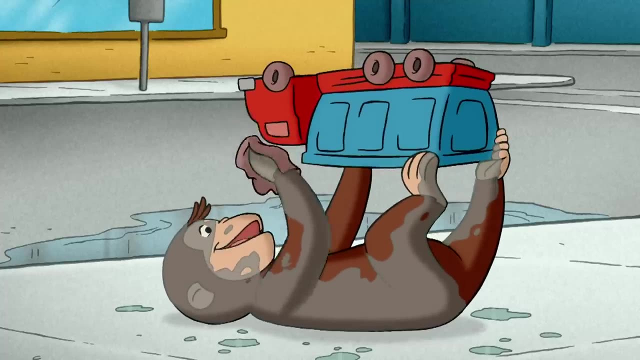 I wish, but George won't take a bath anymore. I don't get it. Maybe George feels he's getting too old for a bath. Of course That's it. My little monkey is growing up Now. I know exactly what to do. 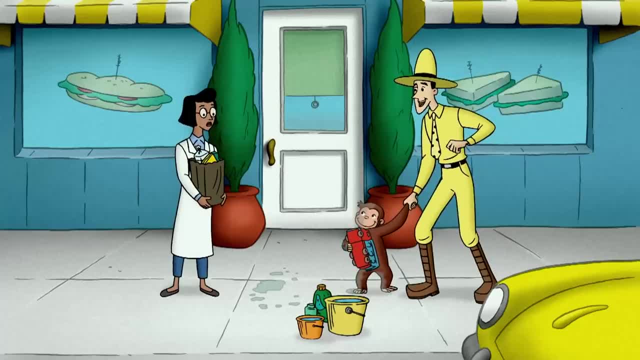 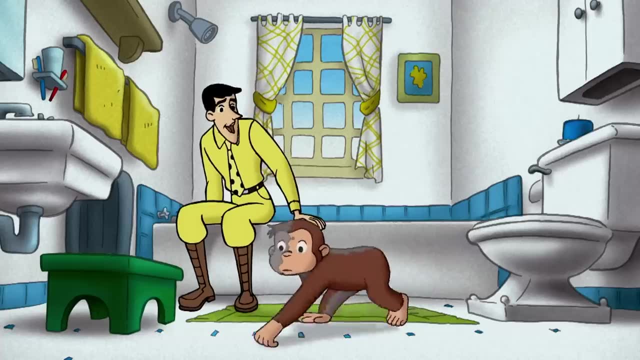 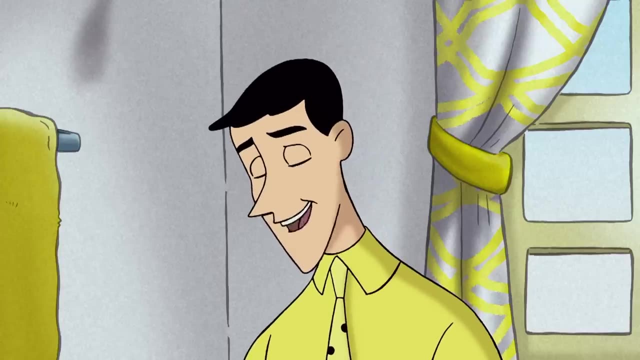 Come on, George, We're going in. Oh thanks, Professor Wiseman, You're a genius. Well, yeah, I understand your problem with baths now, George, And I agree, It's time for you to start taking showers. 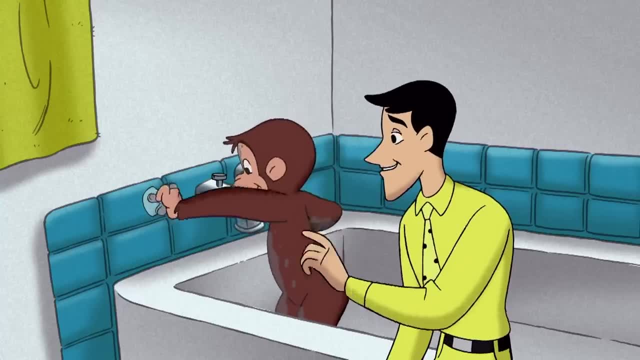 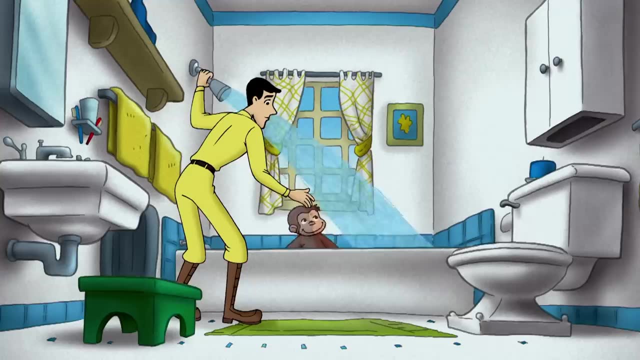 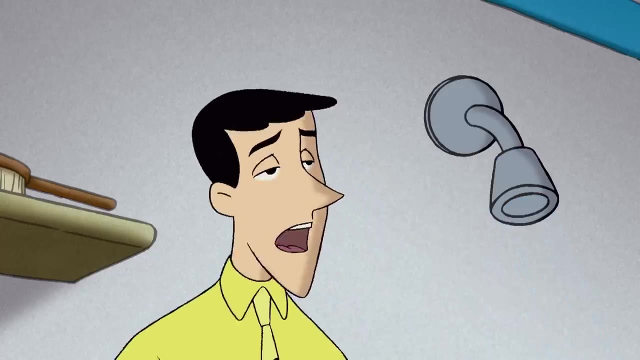 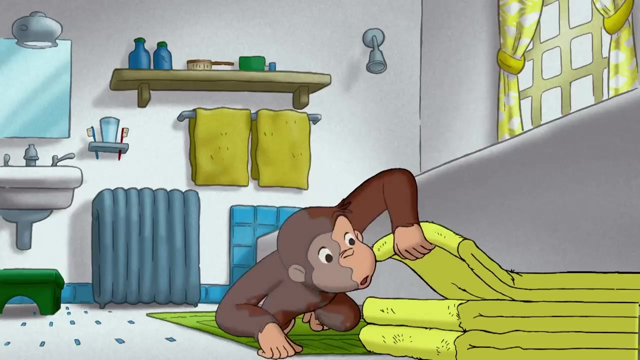 Turn on the water, George, and see what happens. What's this? Oh, George, George, Oh, OK, Won't take baths, Won't take showers. I need to take a walk and not think about any problems for a while. 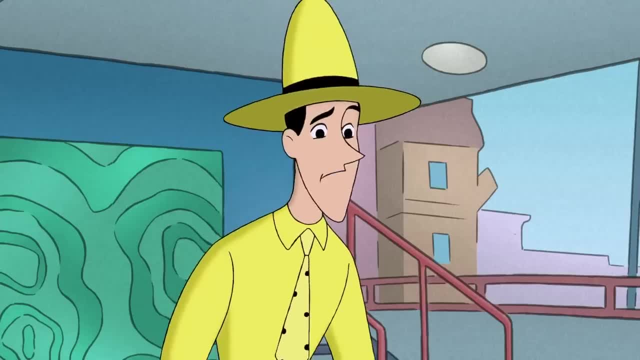 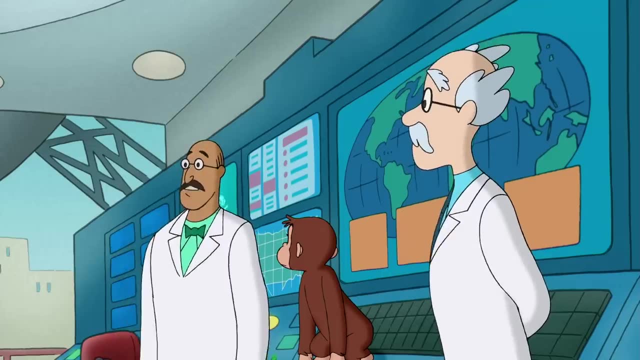 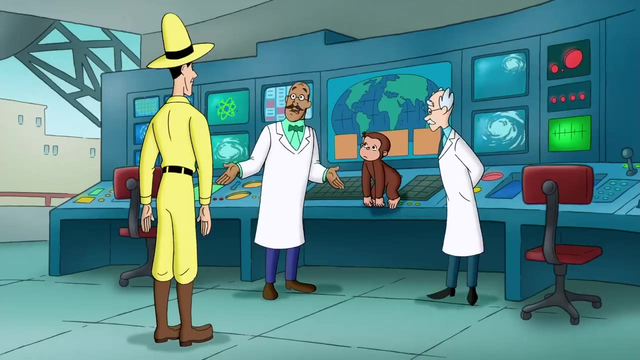 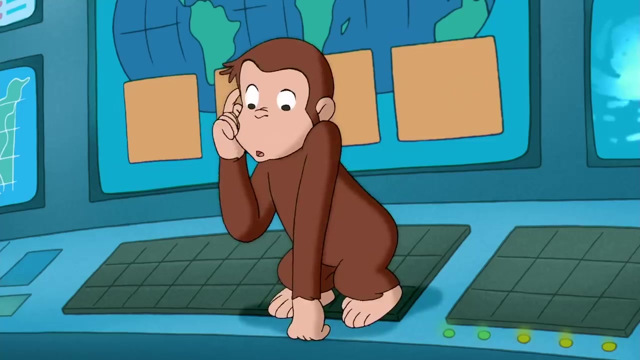 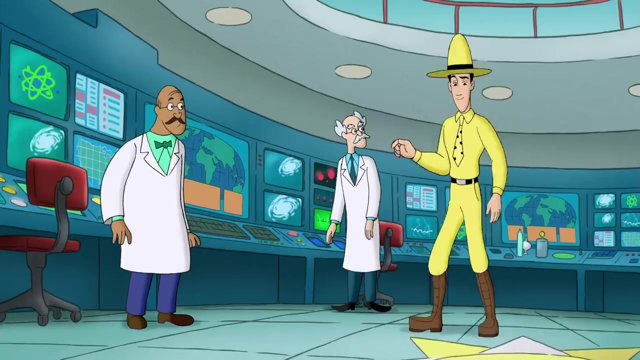 our satellite. you lost your satellite. well, space is very big. and now the mayor's coming by to see if he can play golf today. he hates getting caught in the rain. so did monkeys. without satellite data, our computer can't forecast shist- absolutely hopeless. is he going? so, monkey, fast? i think he wants to predict the weather for you. 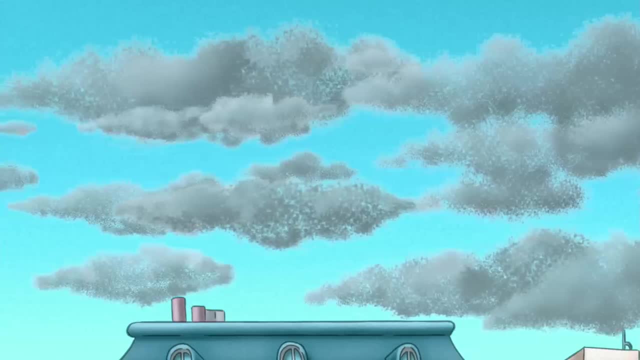 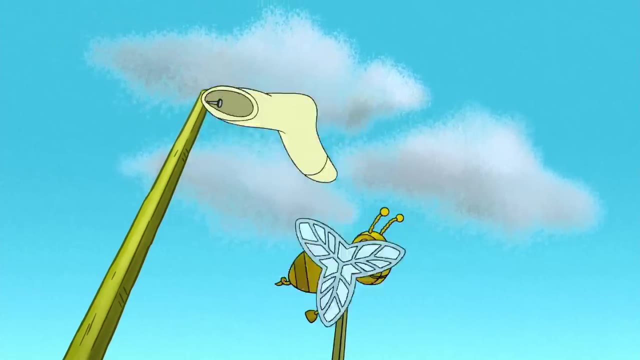 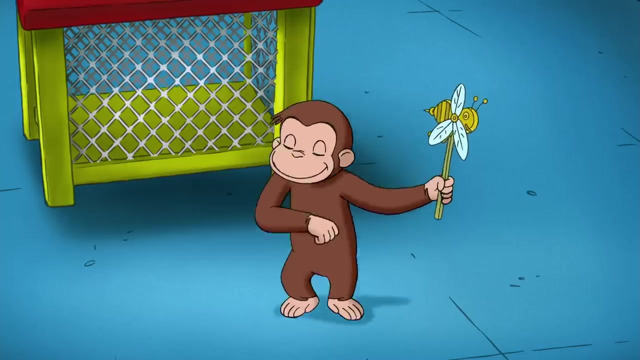 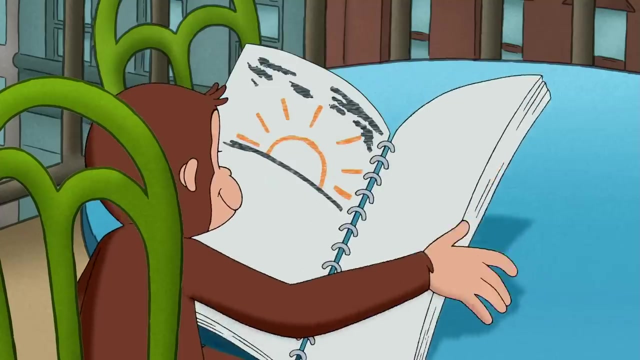 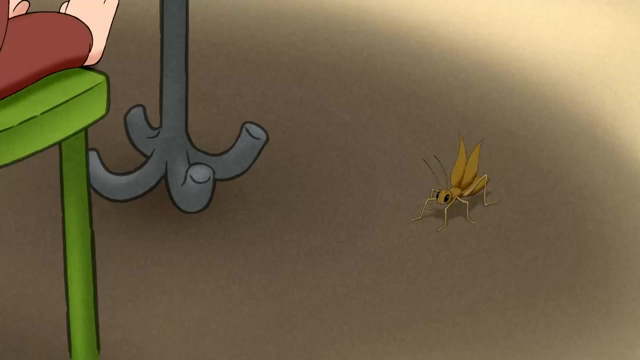 there were storm clouds in the horizon, but the The wind was blowing them away. Oh Ah-ha. George checked his drawings. The sky was red last night And now, with the crickets' fast chirps, George knew it would be a warm day. 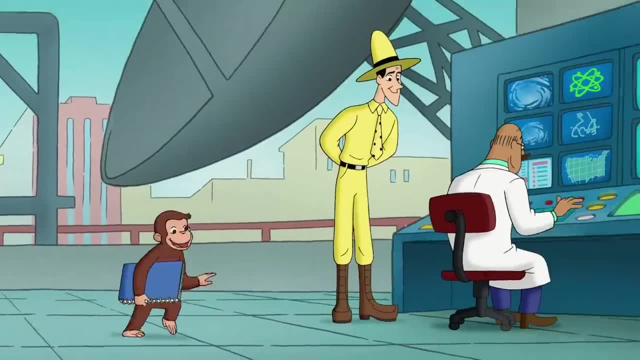 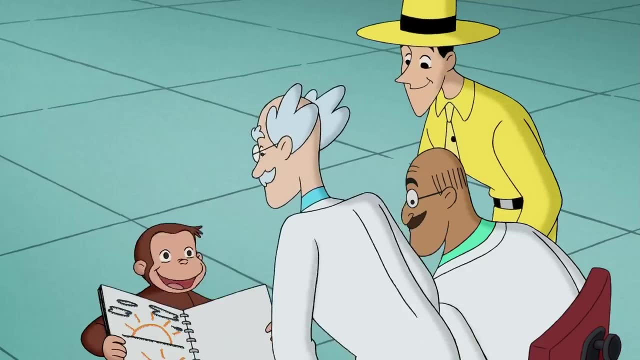 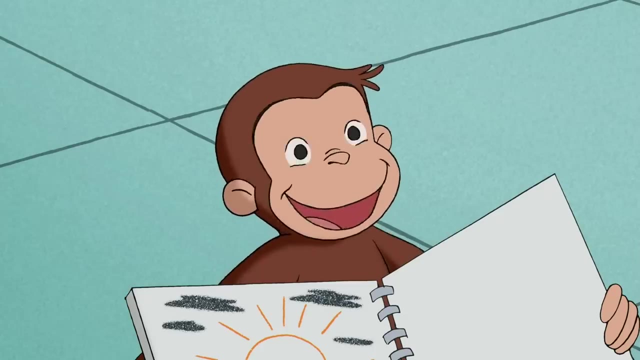 Ah-ha, Woo-hoo. So, uh, will it be okay to golf? Ah-ha, They say that some animals can predict the weather. Maybe George is one of them. Ah-ha Professors, Mr Mayor. 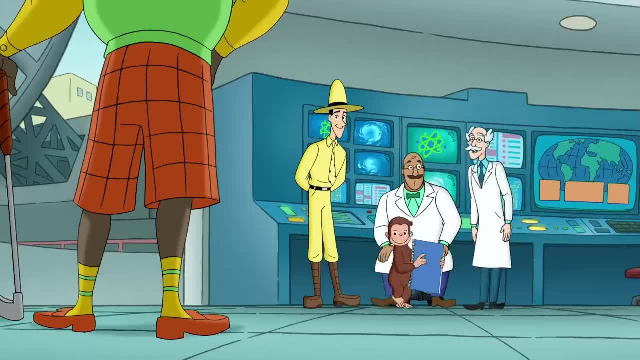 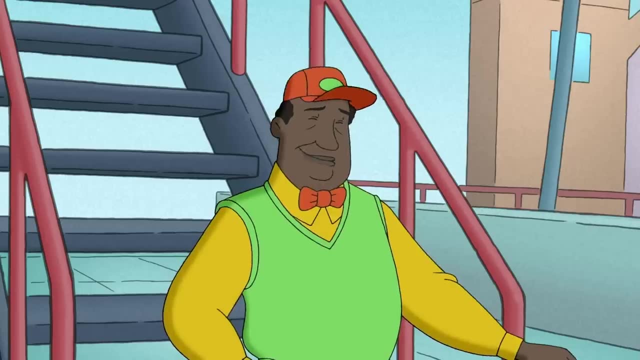 What's the verdict? We have it on the best authority that this afternoon will be perfect for golf. Ah-ha, Splendid, Isn't modern technology? wonderful, Say. why don't you take a look at this? Join me, Woo-hoo. 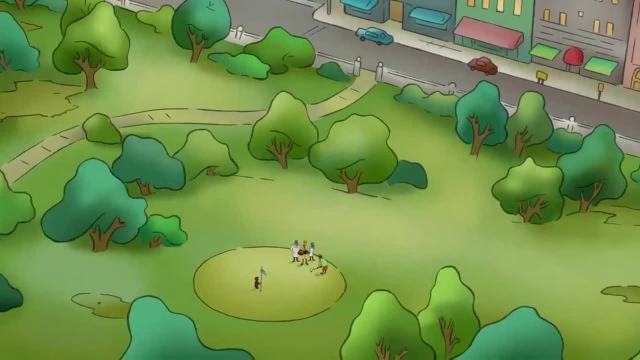 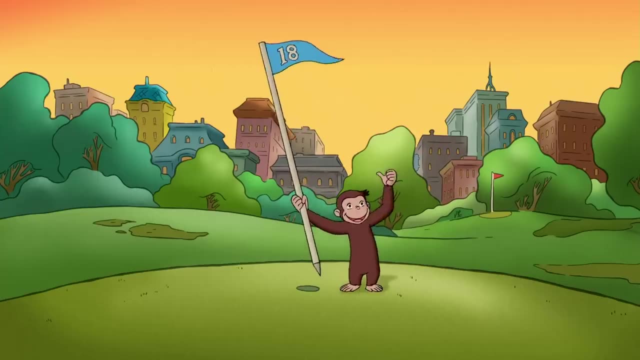 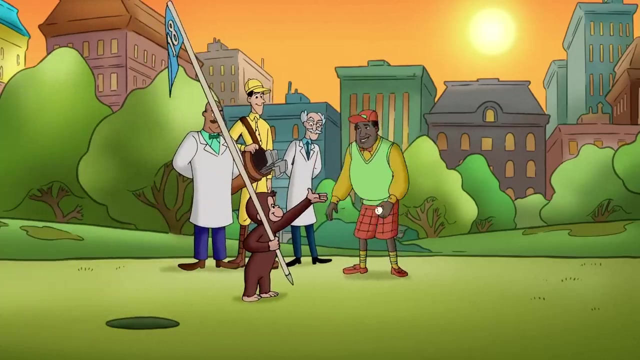 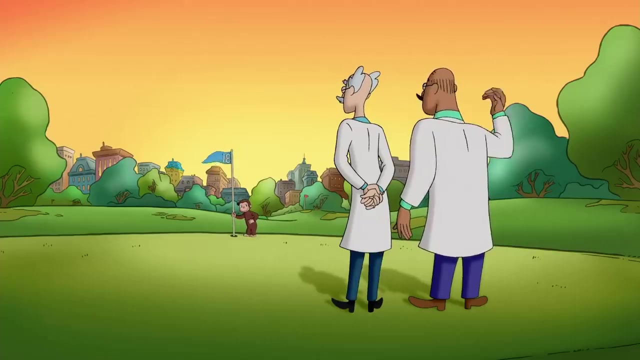 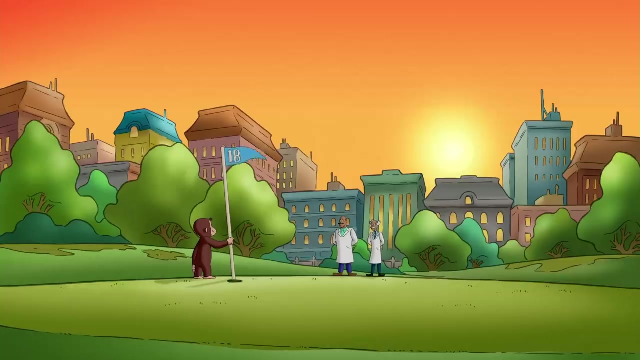 Ah-ha, One of the finest days I've ever seen. You were right. Thank you, George was right, George. perhaps tomorrow you could help us find our satellite. George would have to think about it. Think about that. The sky was telling him. 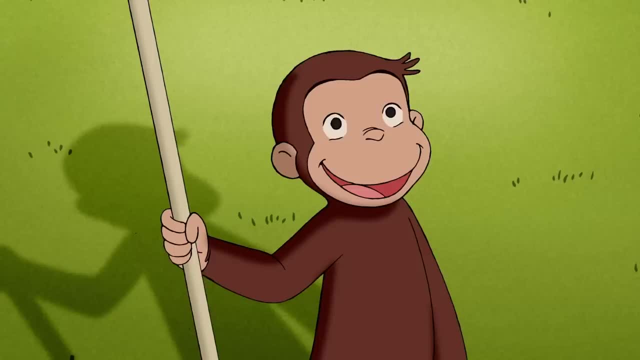 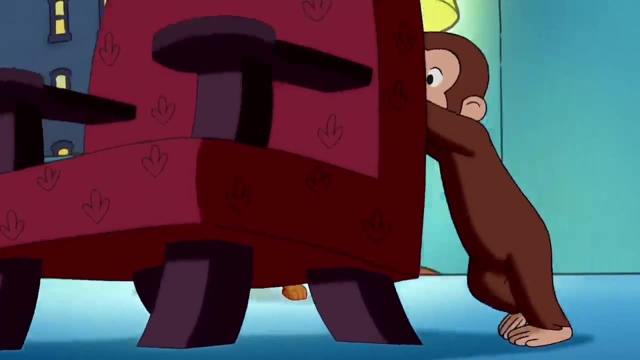 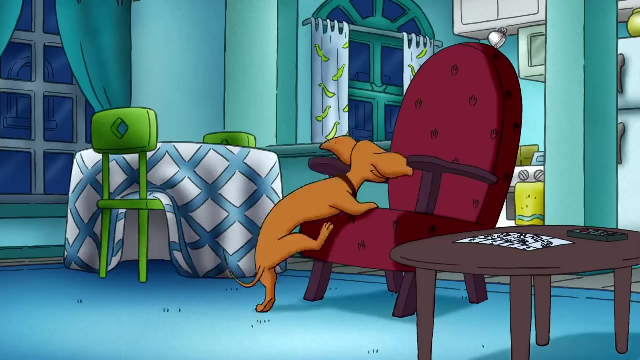 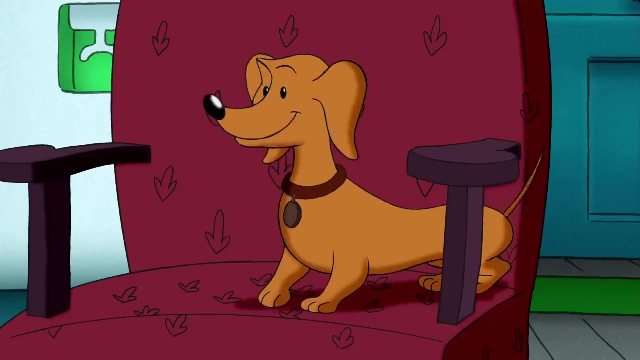 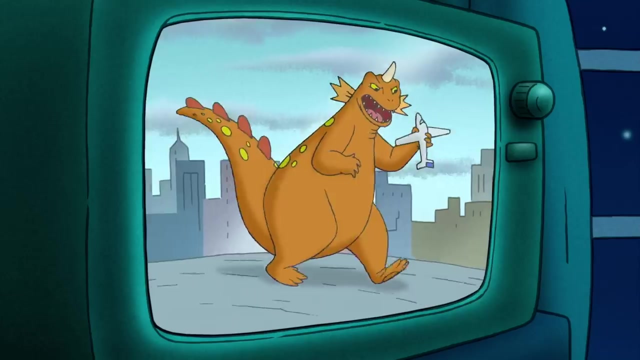 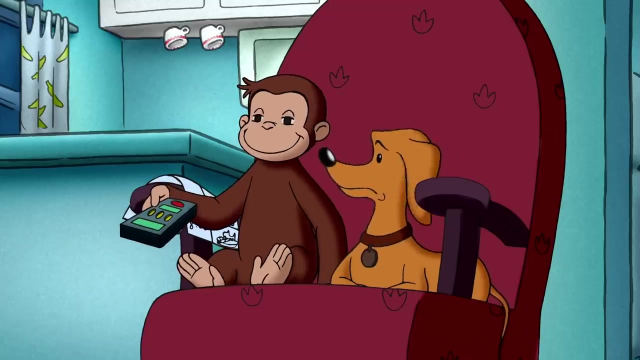 tomorrow might be a perfect day for a picnic. Keeping a house guest happy was a lot of work, but now they could enjoy something together. Woo-hoo Ah-ha Boo, Woo-hoo Ah-ha. Huntly didn't seem to like the monster show. 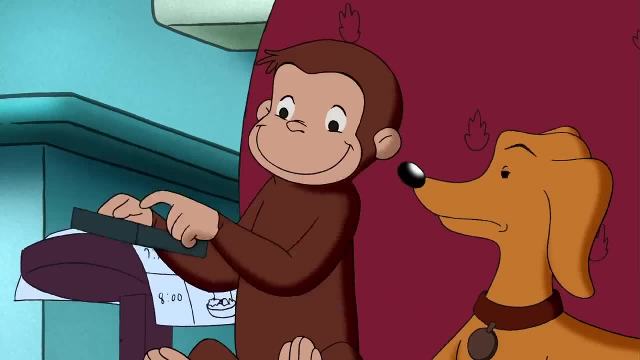 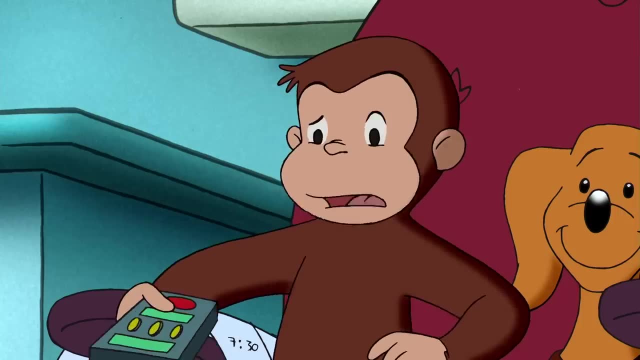 Maybe that number was his favorite channel. Ahh, Ahh, Ooh, ah, ah, A ha, ha, ha, ha, Oh, ooh, ooh, Ah, ahh, Oh. a part Overall, George was sure Hundley would enjoy the monster show more than poodle groomers. 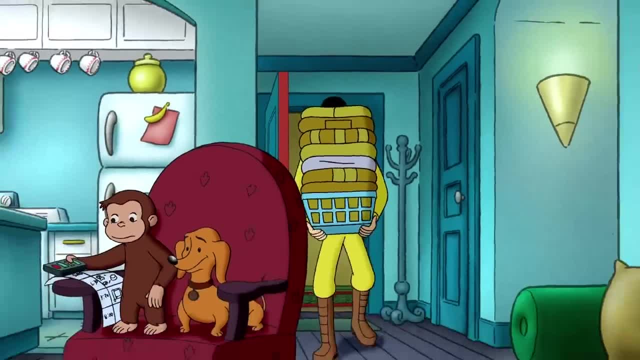 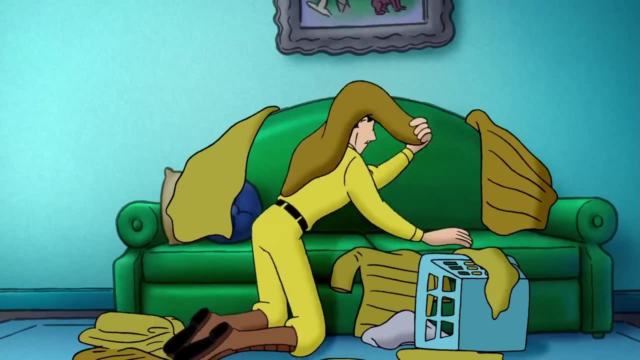 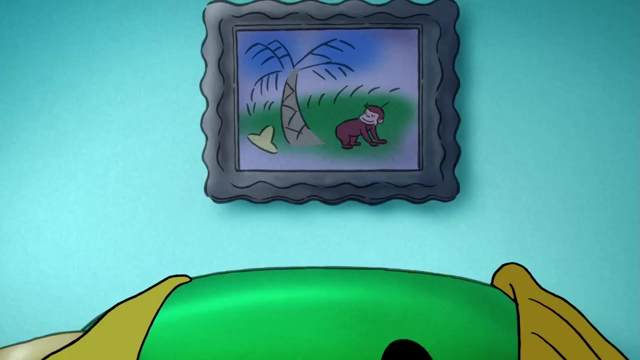 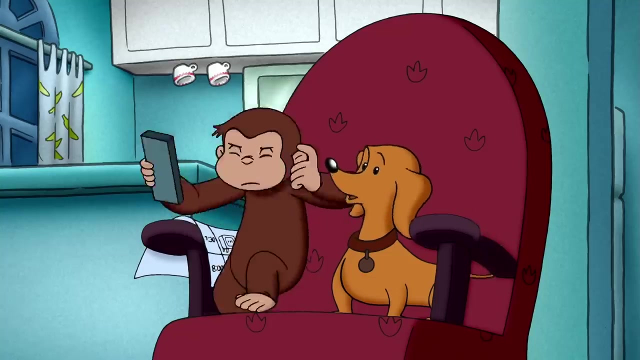 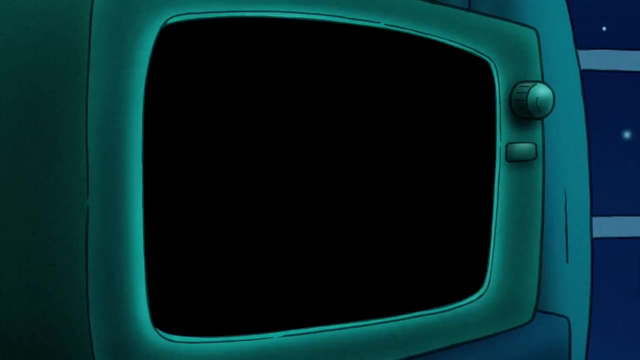 George, you know our rule: No monster show before bedtime. It gives you nightmares in every. Hey, this looks like Hundley's apartment. Oh, I get it Making him feel at home. Very nice, George, It's bedtime for monkeys. 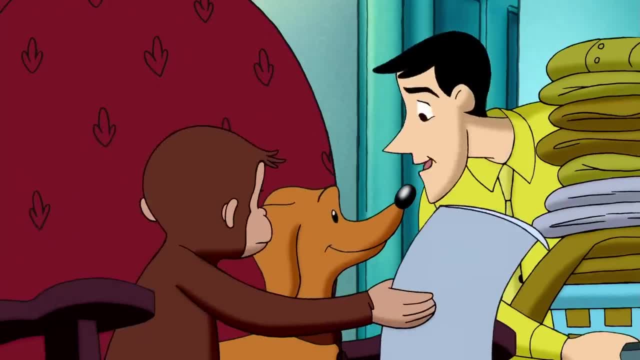 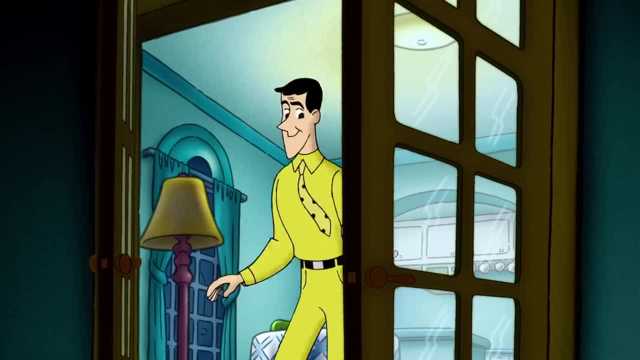 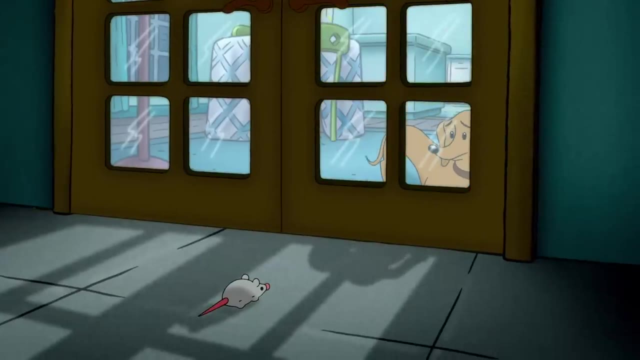 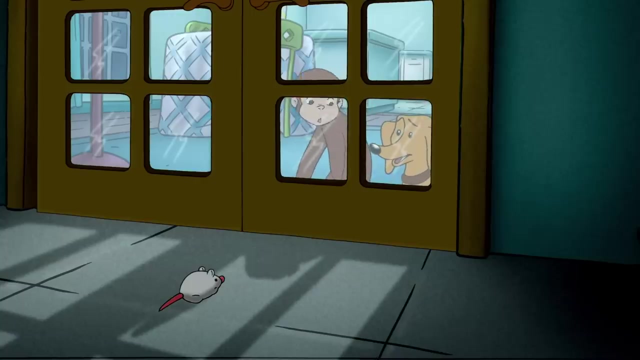 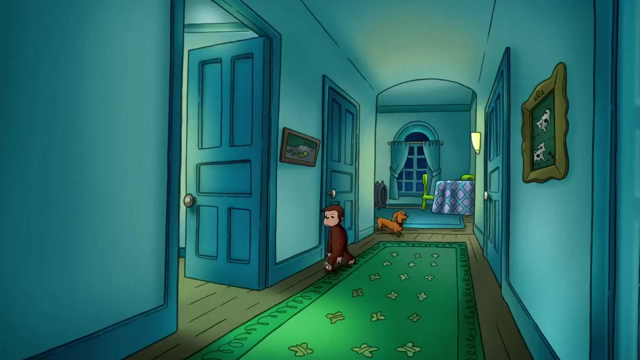 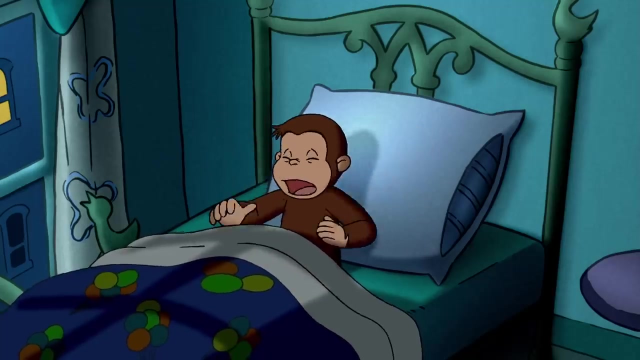 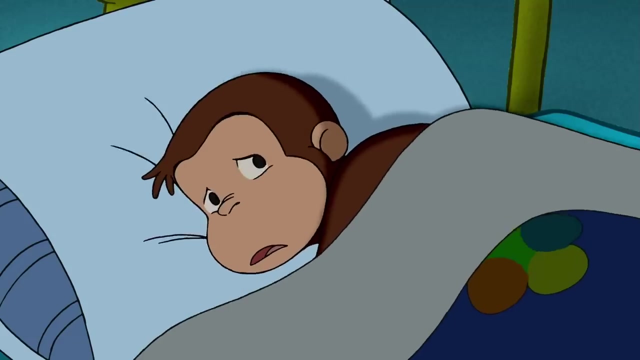 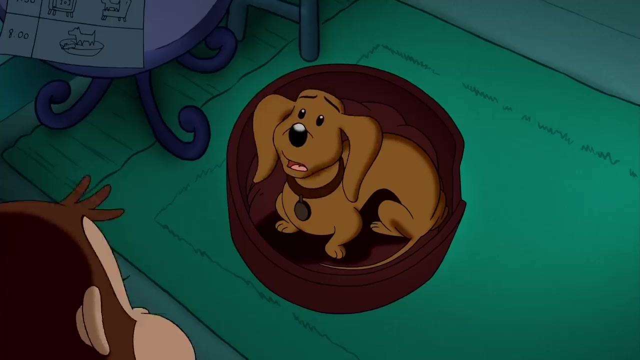 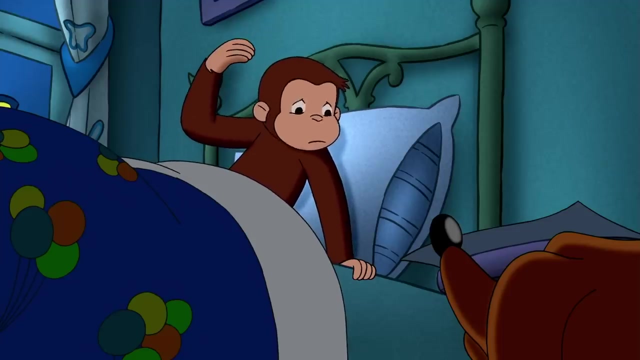 Oh, dachshunds too. Hundley was confused. How did his squeaky mouse get out there? George couldn't believe that Hundley wanted to play with a squeaky toy now, But it was too late. Just to make sure Hundley wasn't trying to tell him something important. 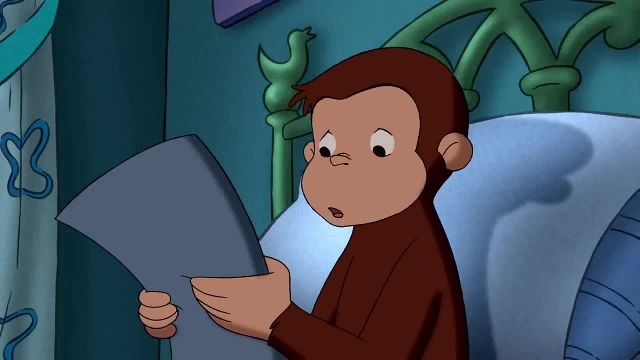 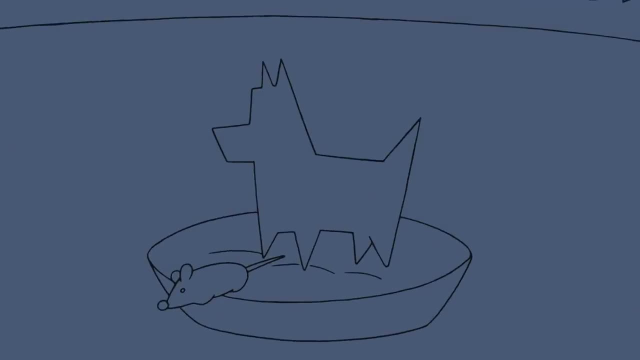 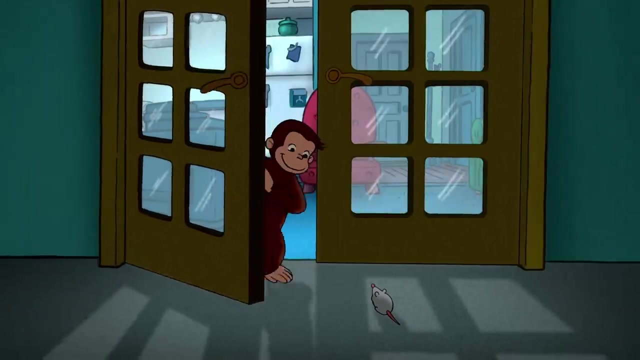 George checked the list. Hundley didn't want to play. He always slept with Squeaky Mouse. Squeaky Mouse helped Hundley sleep and kept nightmares away. Hundley was very happy to have a friend like George who would get out of bed. 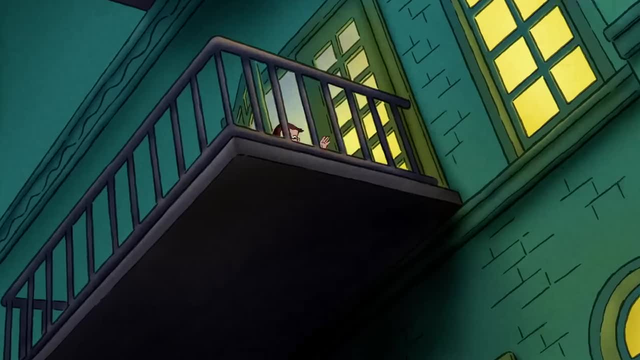 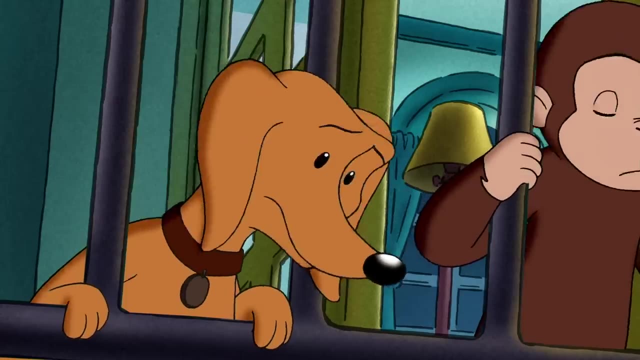 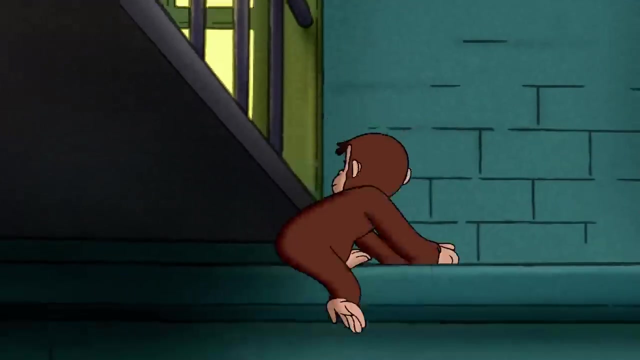 to kick Squeaky Mouse off the balcony. It was about time for him to let everyone know that there was a ghost that was playing with Squeaky Mouse. When he saw this, he took a few steps to the inn. The monster came out and he got rid of the ghost. 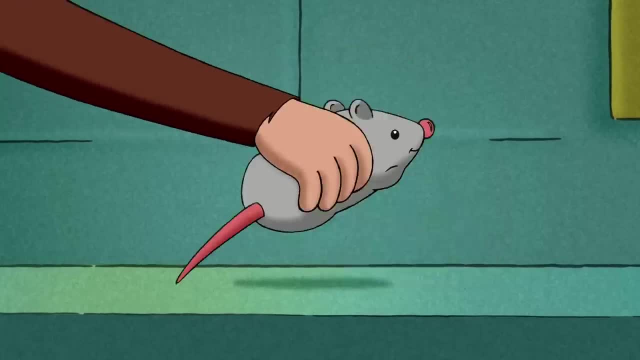 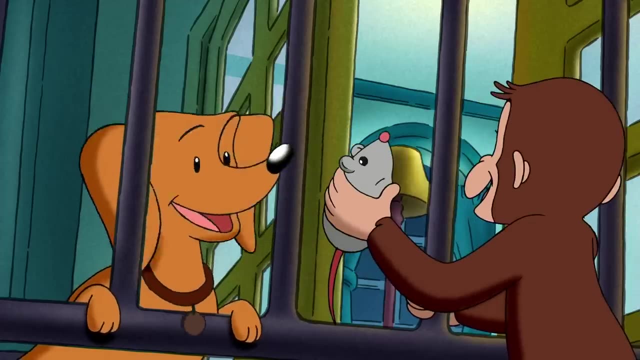 He started his new game called confused. It's a little bit like Nosy, but it has more detailed rules and directions. You can play in the care of people around you and save lives. That's how it goes with me. In the meantime, háér is sleeping. 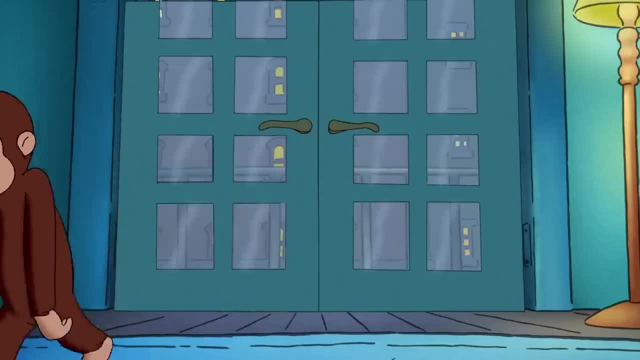 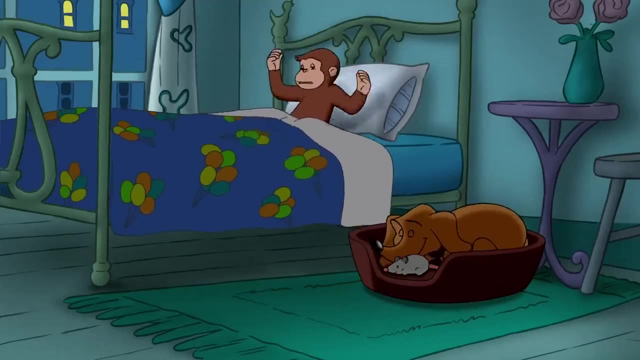 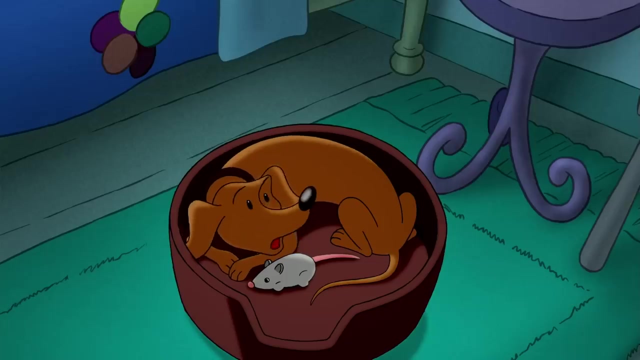 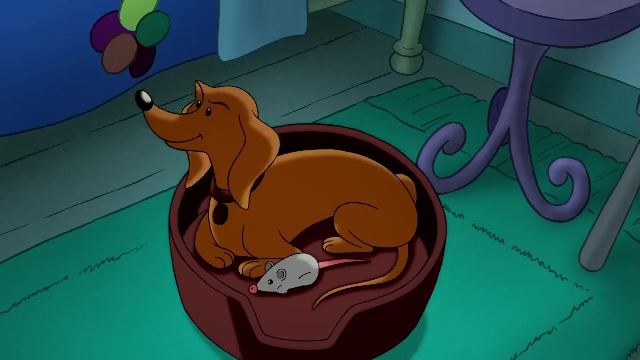 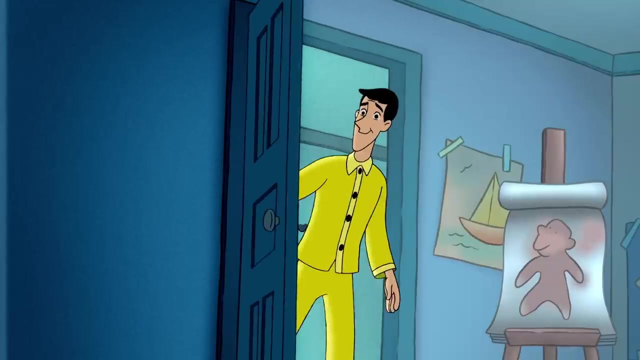 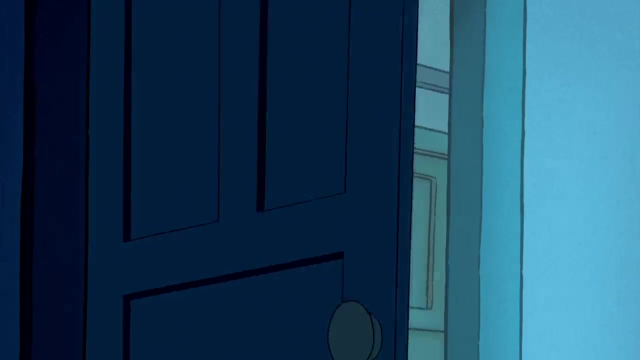 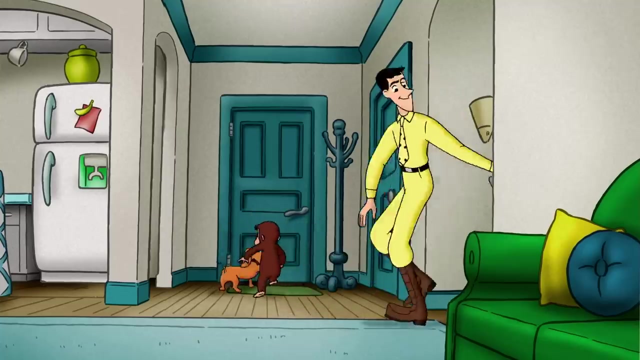 How is he? Good, Good, Good, Come on, come on, come on. Hundley knew George was having a bad dream And he didn't have his own squeaky mouse. Hello, Hundley, How you doing, boy. 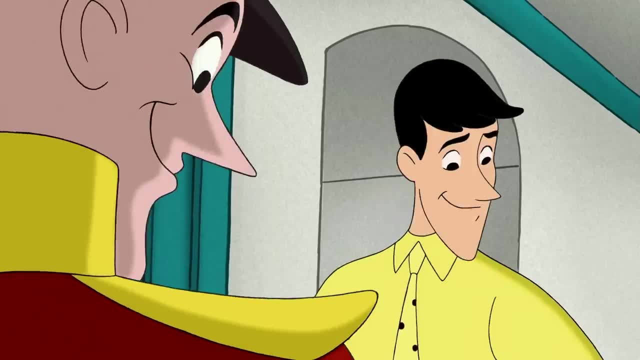 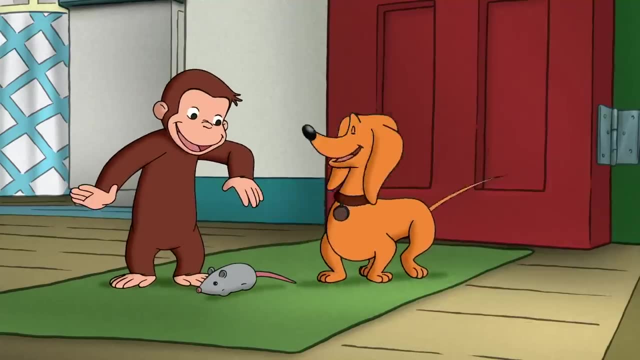 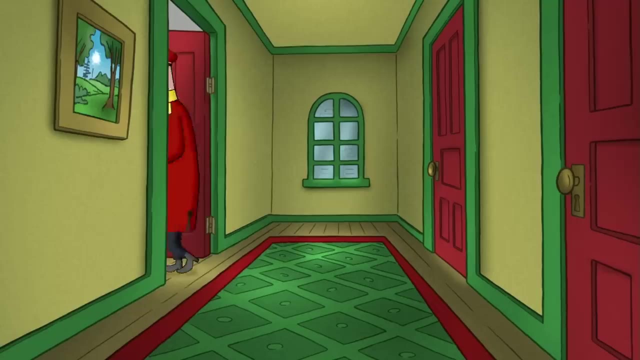 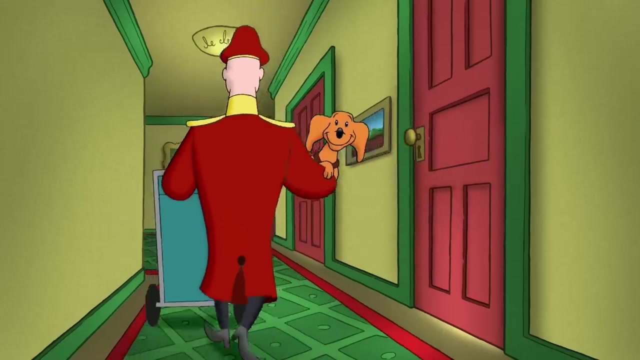 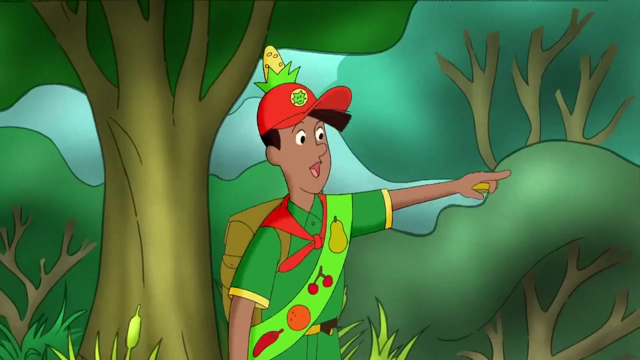 Was he any trouble? Not at all. Right, George Hee-haw Hundley says: thank you. Dogs and monkeys don't always understand each other, But sometimes a squeaky mouse can tell you who your real friends are. According to my compass, this way is north, this way is south, and east and west are here and here. 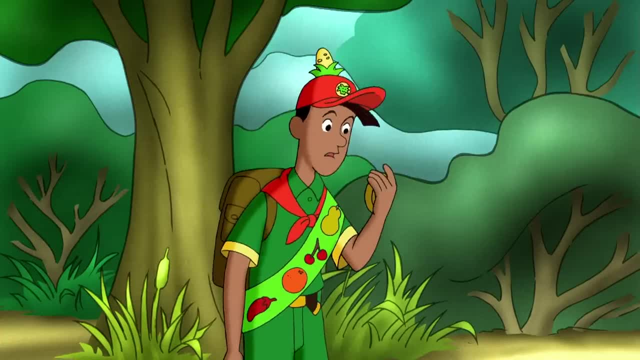 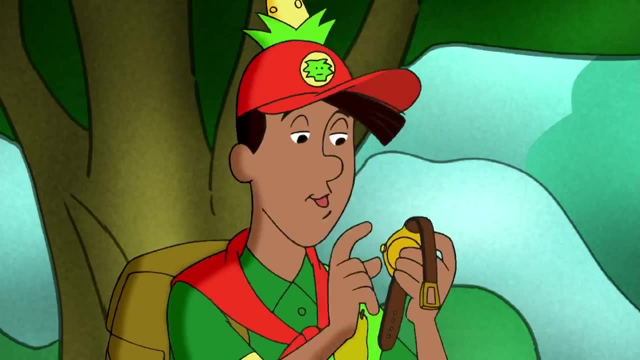 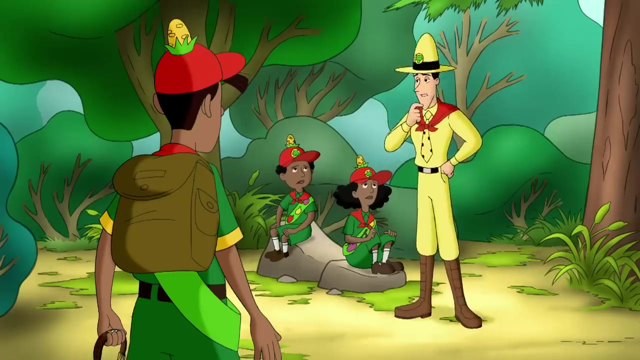 But without a map. that doesn't really help us. But you know what? We can determine our precise location using an analog watch. We just need to know the true local time. Do you know the true local time? I have another idea. 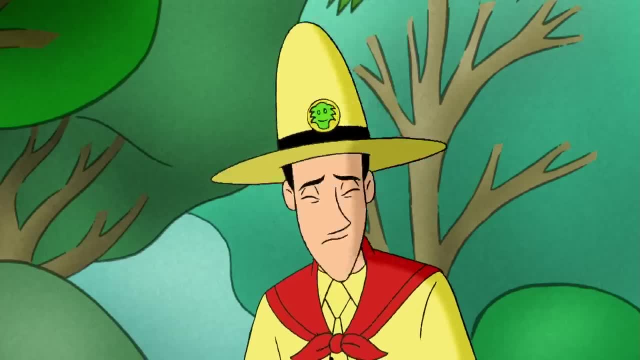 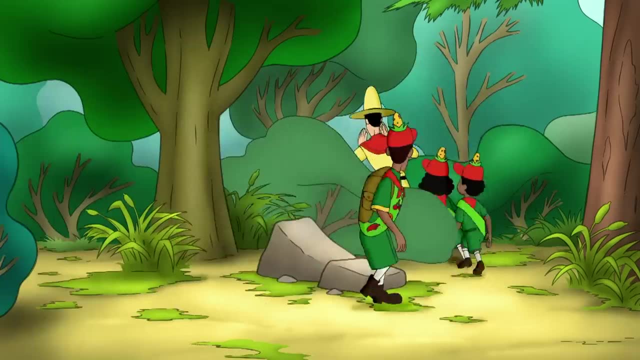 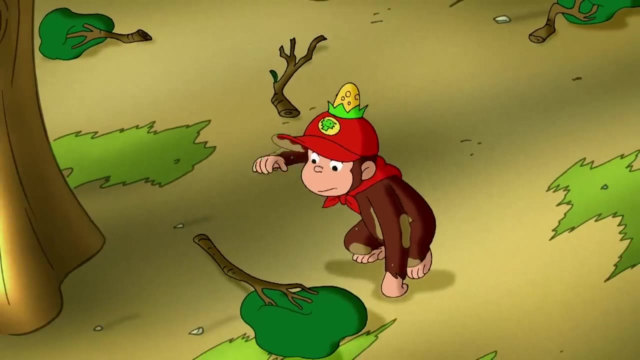 Let's ask George to climb a tree and Oh no, I left George in the tree. George, Where are you, George? George wished he could think of a way to get the branches back on the tree, But he needed something sticky. 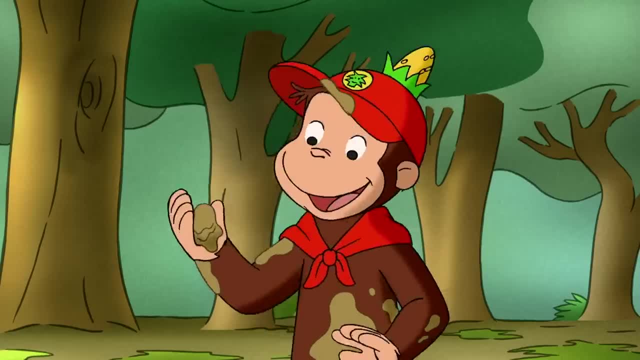 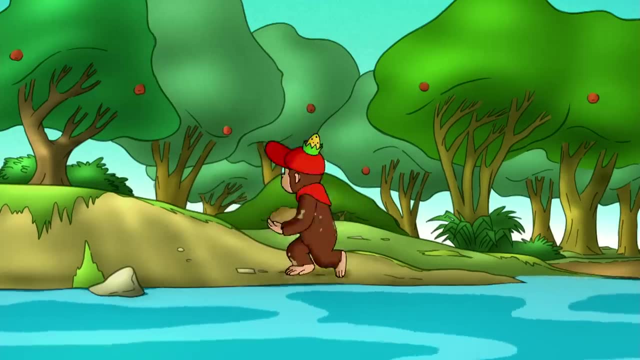 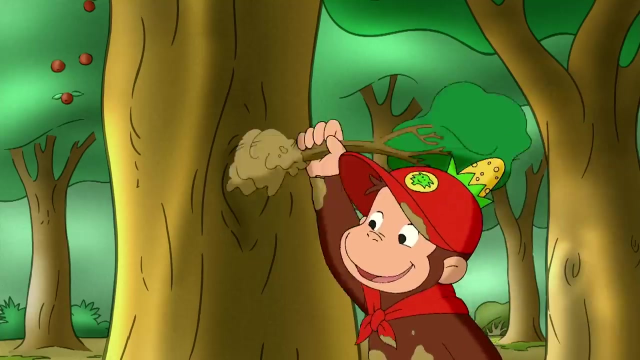 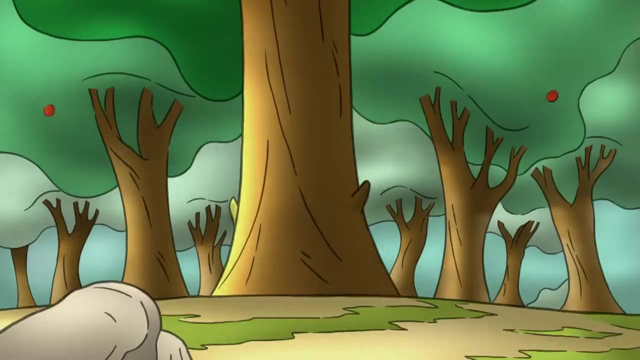 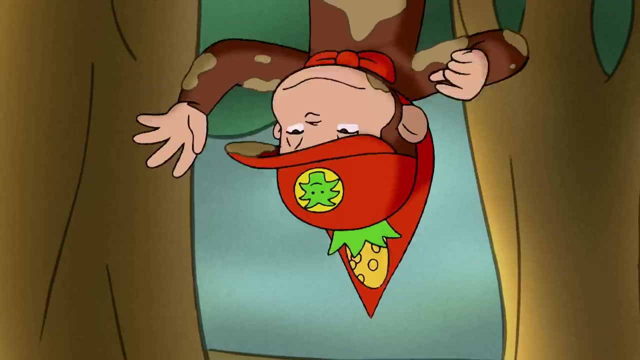 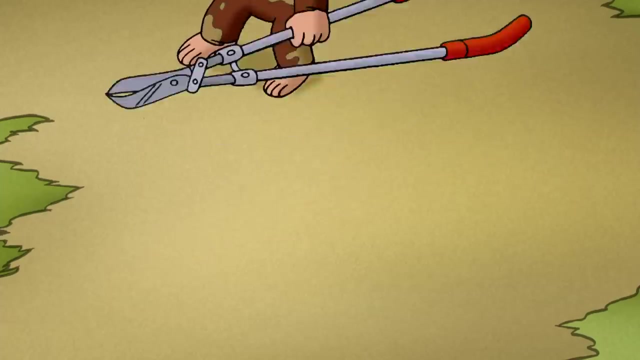 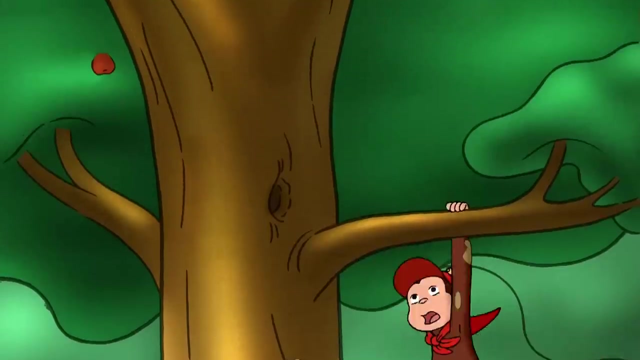 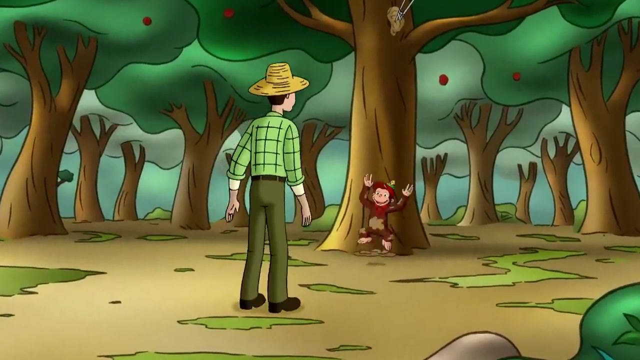 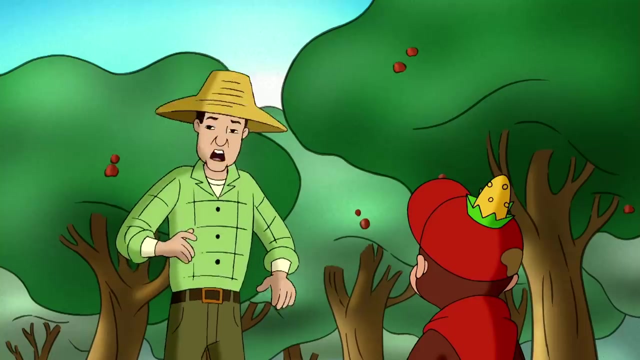 Really sticky Like mud. Another great monkey invention: the tree wrecking man was coming back and he'd probably want to keep on wrecking. you are one crazy monkey. i haven't run like that since. hey, where's my lopper? that thing i was cutting branches with. 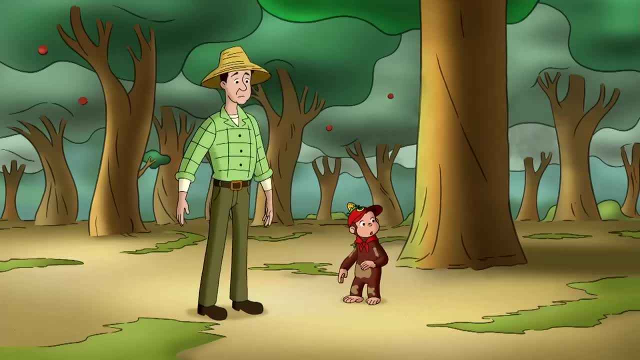 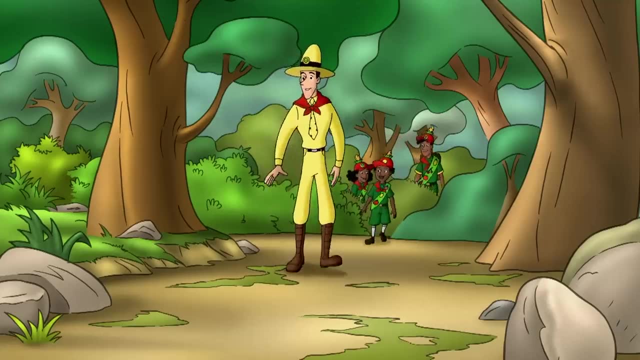 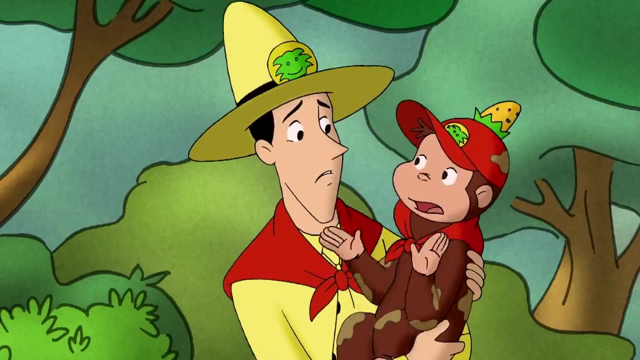 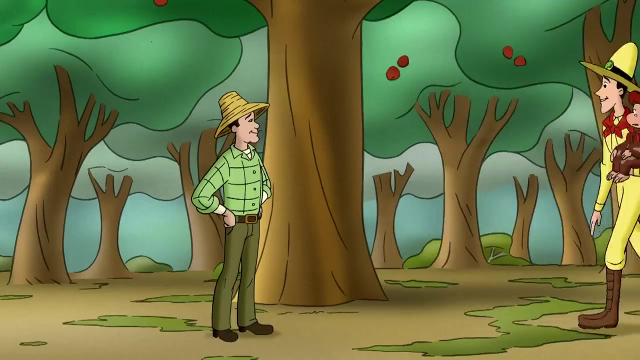 george, can you hear me, george? george, oh, thank goodness i found you. oh, i'm sorry i left you in that tree. oh, dr green bean, nice to see you. sorry we're late. we've had a rough day. tell me about it first. this monkey ran off with my hat. 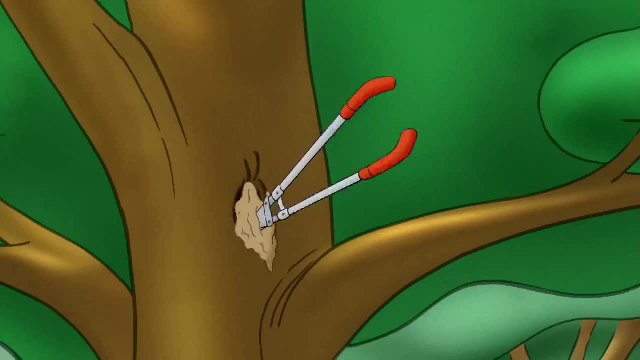 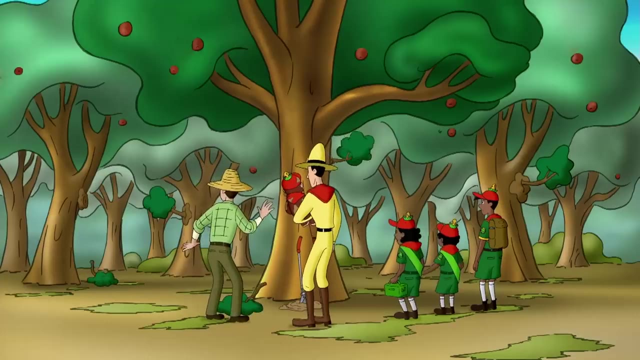 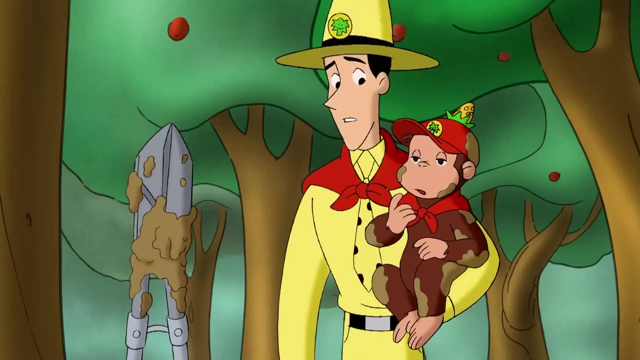 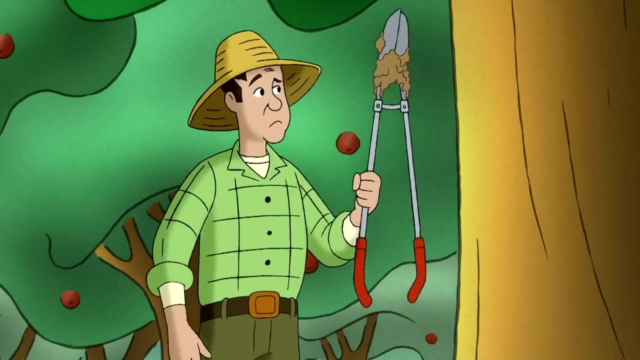 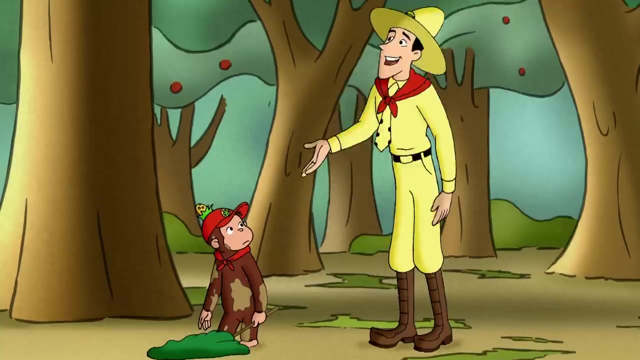 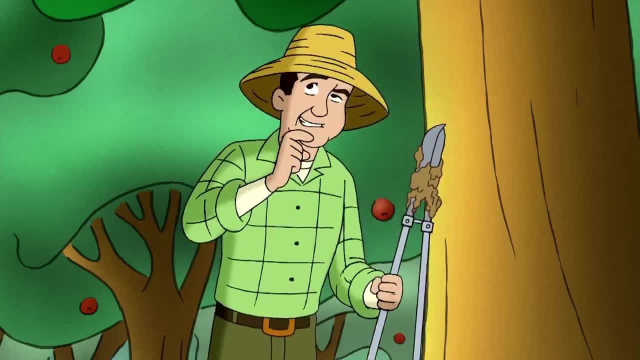 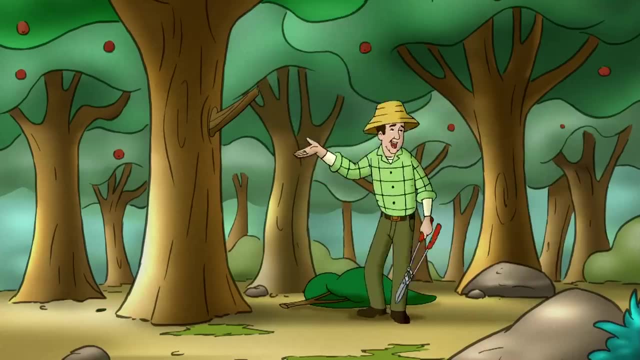 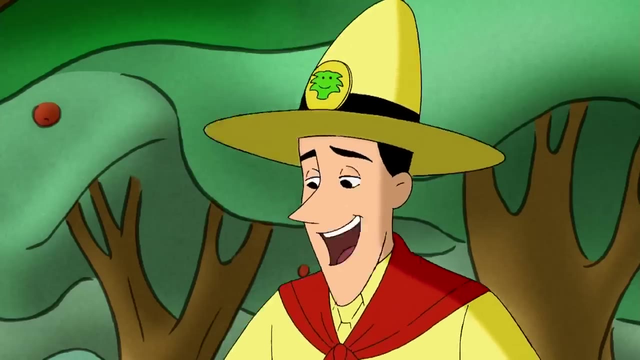 you should have asked: oh wait, you're a monkey. well, anyway, this is called pruning. you make a careful cut and it doesn't hurt the tree at all. he's right, george. i've pruned many a tree in my day. you see, george, too many branches are bad news. they block the sun. 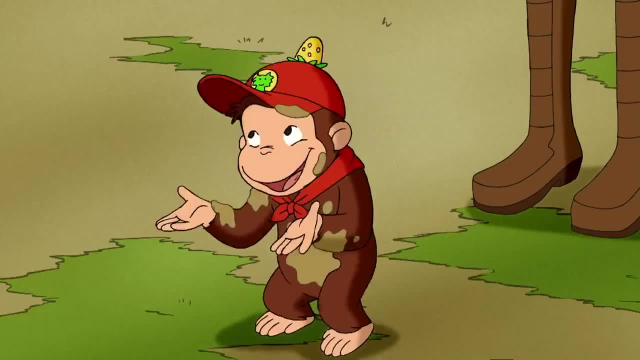 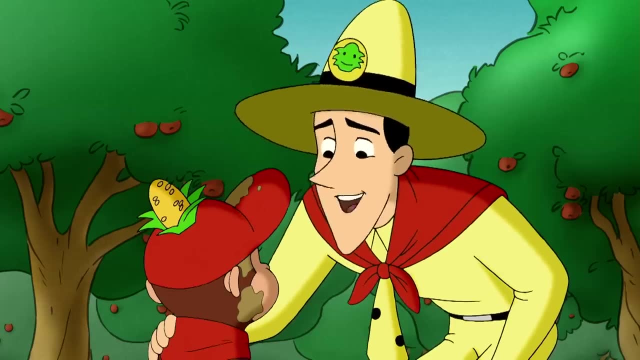 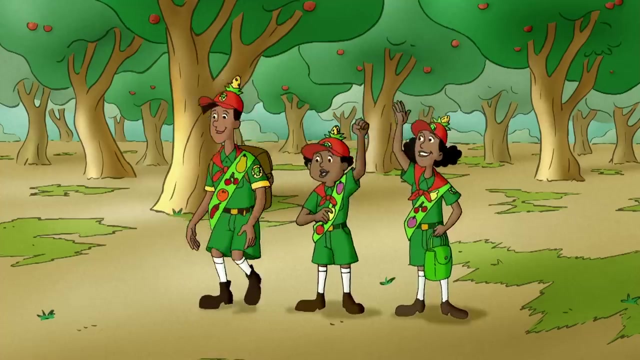 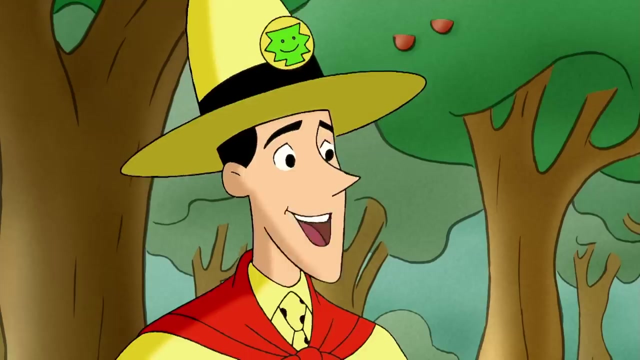 and then the fruit can't grow, hey. but hey, i'm proud of you, george. you behaved just like an honorary sprout. in fact, i would say your effort on behalf of trees qualifies you for full sprout status. nice work for a city kid. okay, sprouts, let's go get some lunch and dr green bean can tell us everything he knows about trees. 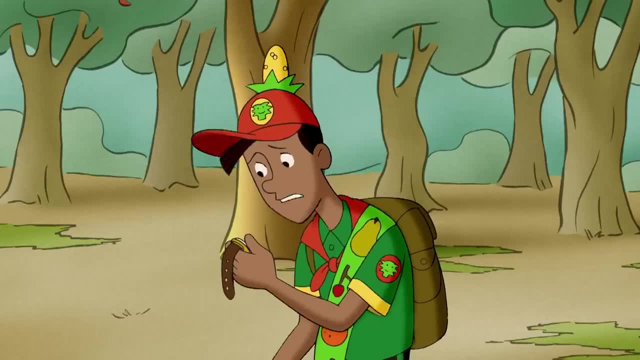 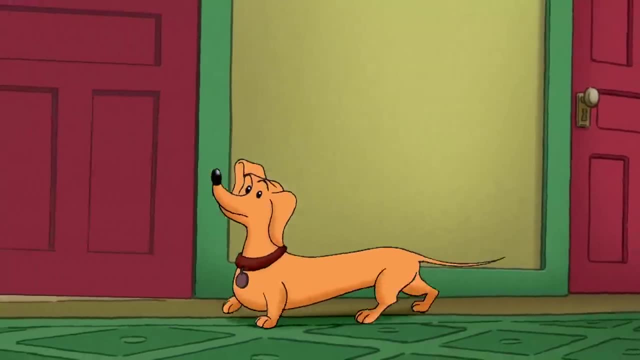 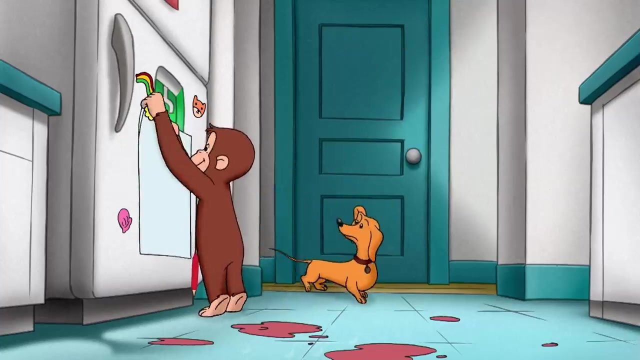 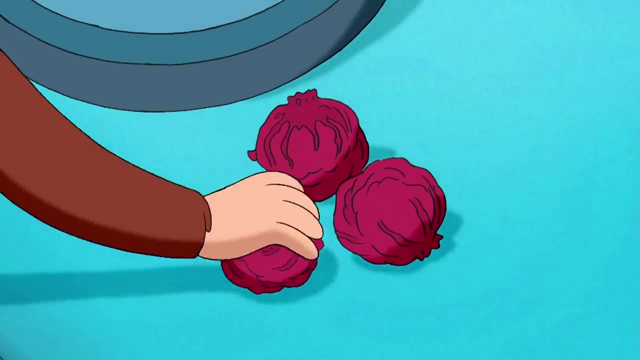 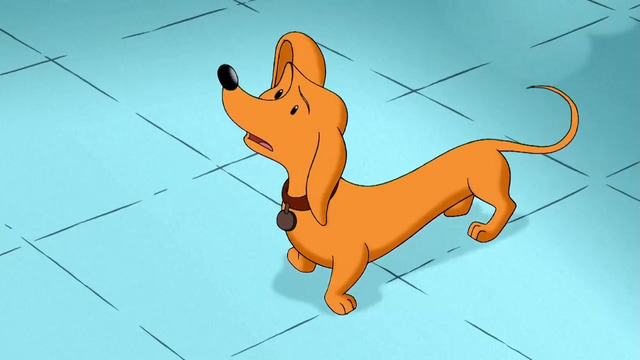 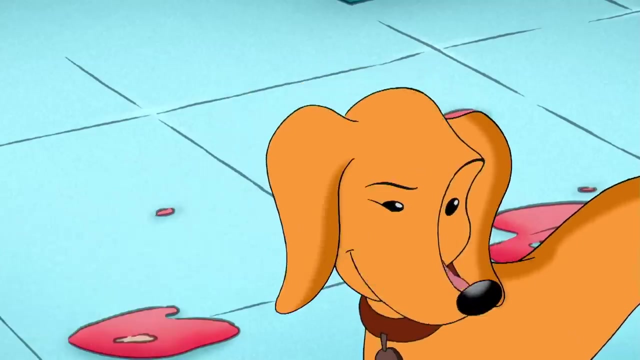 bill, are you coming in a minute? I'm still trying to figure out where we are. Oh, George decided to experiment with different amounts of each ingredient. He used a big piece of paper to keep track. Not berry enough, So George added strawberries. 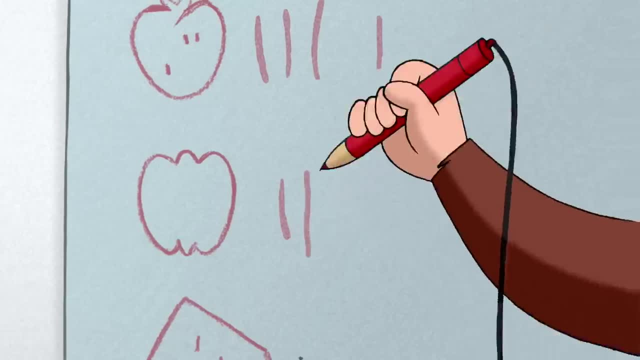 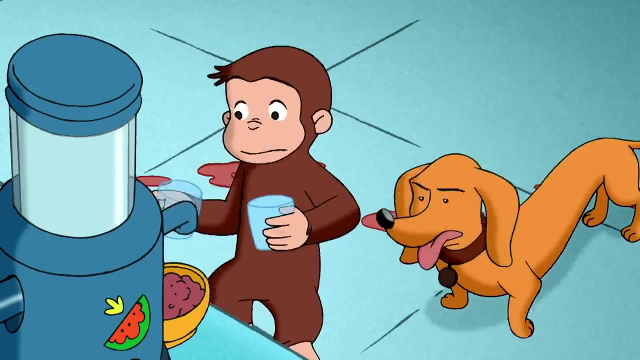 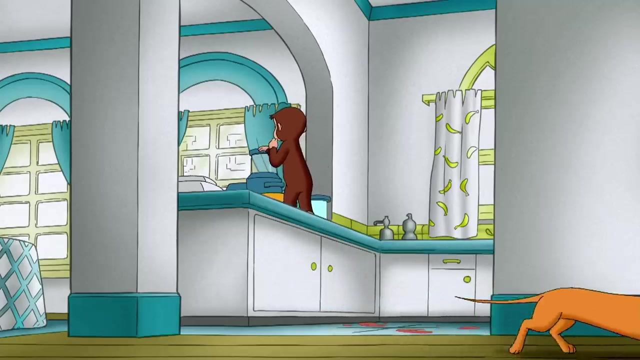 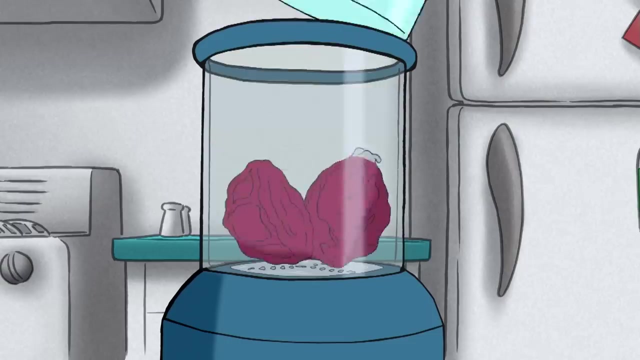 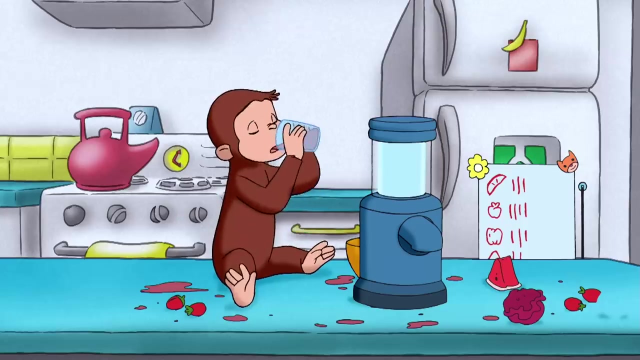 Too sweet. George added more peppers. It still wasn't right And it certainly didn't pass the Hundley test. Maybe George needed more of these things. Close. But George thought more apples might help. George's juice was perfect- Well, almost. 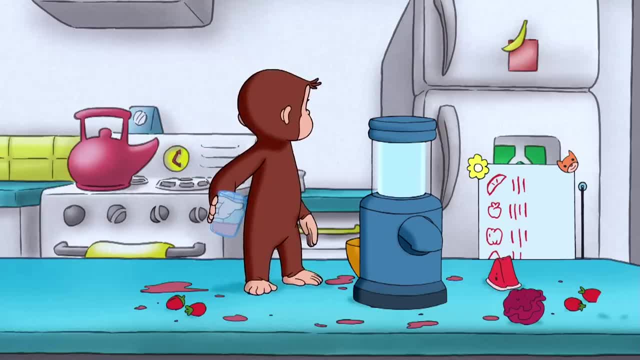 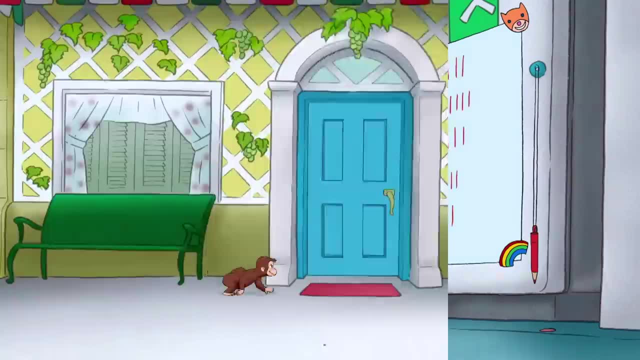 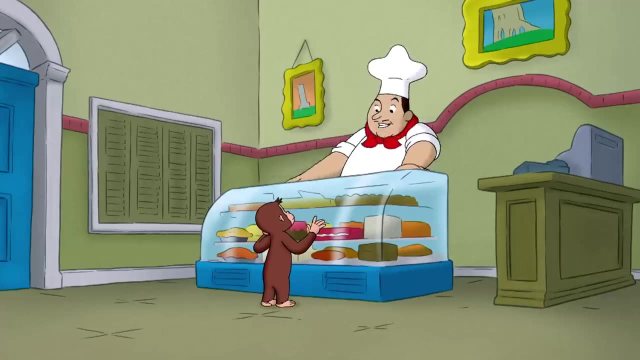 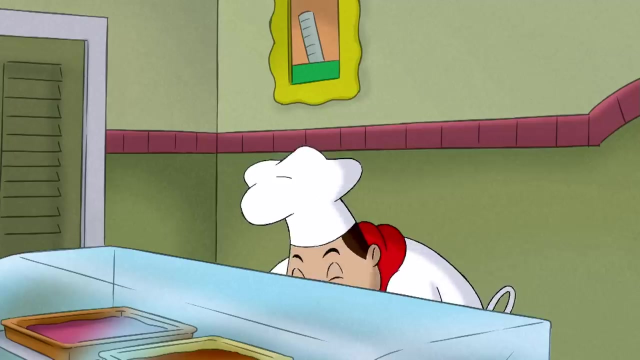 It still needed a special secret ingredient. Where could he find one of those? Hello George Say, can I interest you in today's special Special? That's exactly what he was looking for. It's eggplant piccata With extra amounts of piccata. 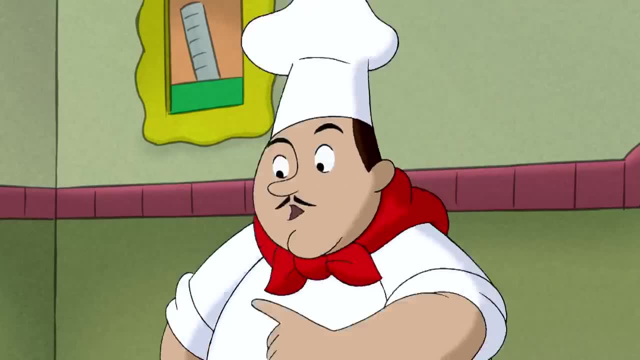 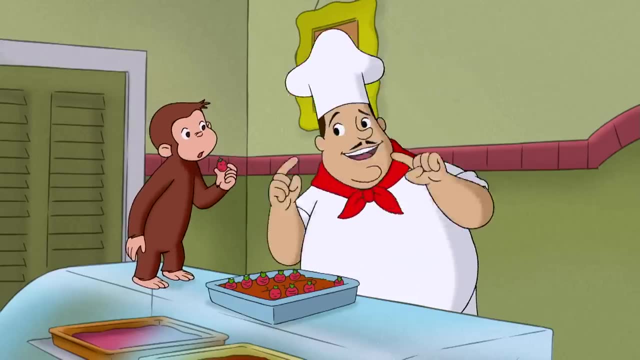 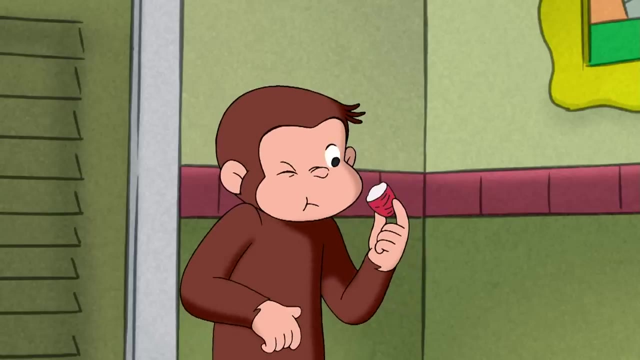 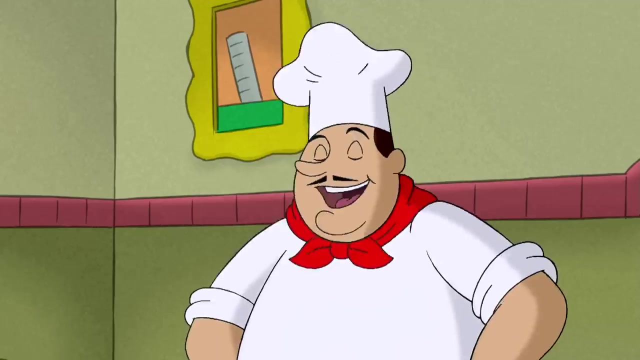 Oh, those are radishes. Try one. Oh, but careful, Radishes are a little speziato, That means spicy. Radishes were spicy, But spicy might be good in a drink. Woo, I know, Help yourself, Georgie. 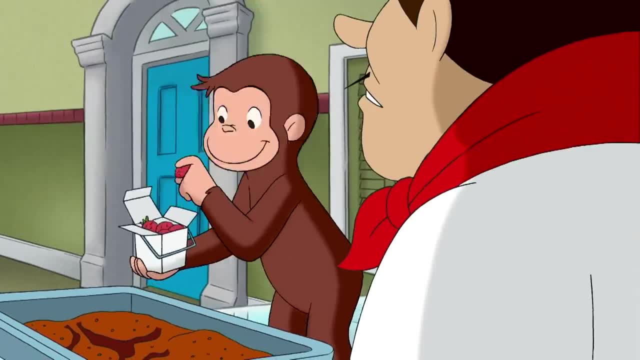 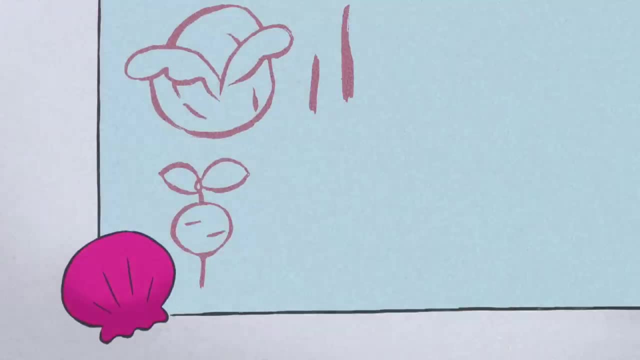 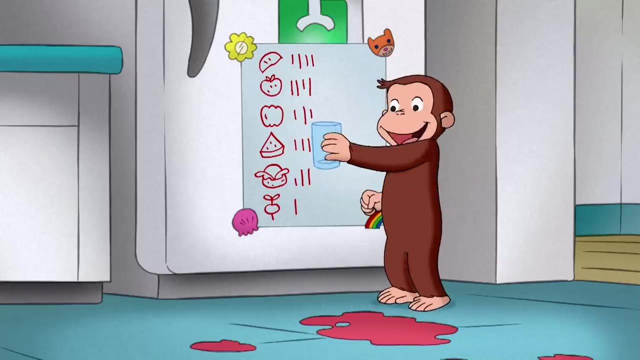 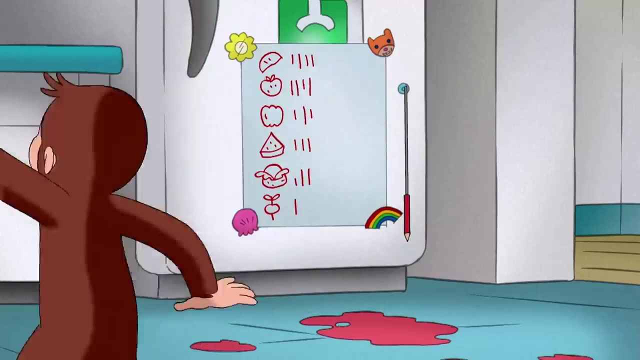 Just the radishes. Ha ha ha. I'm trying Bye bye. George hoped that one radish would do the trick. George had done it. His juice was just as good as Juicy- J's Better, even George. 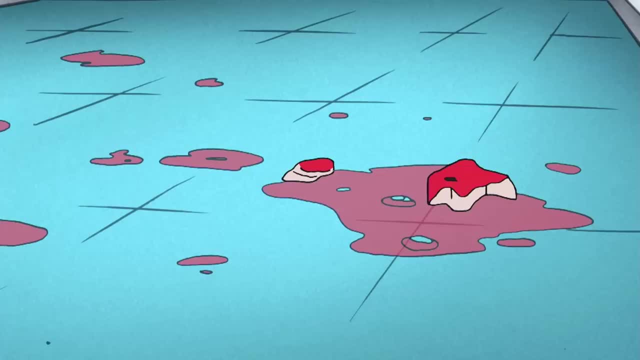 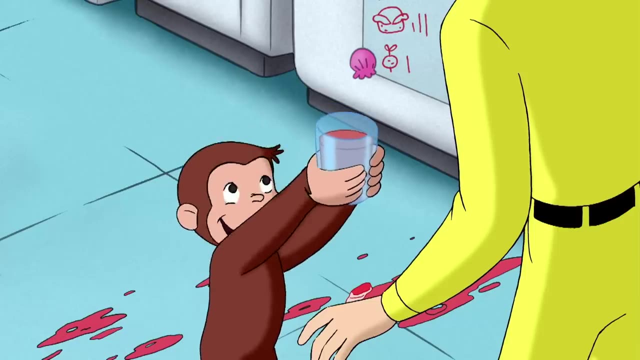 Oh, no, Oh, where are you? Don't go, Don't go, George. I'm sorry, I'm tired, Don't go, Don't go. Oh, have you been making juice, Mmm? Oh, Oh, my goodness, this juice is amazing. 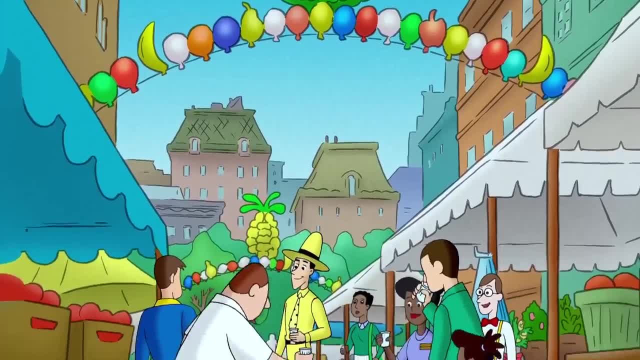 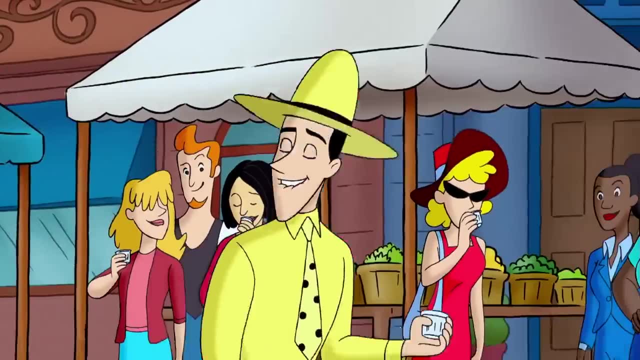 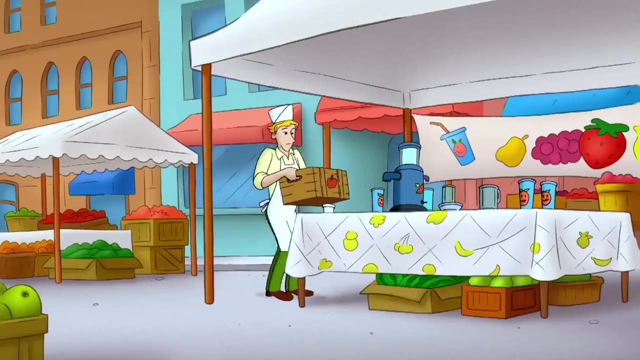 Yeah, George thought his juice was so delicious he decided to give it away at the next farmer's market. Get your George juice. It's made with apples for strong bones, cabbage for vitamin C and a bunch of other healthy stuff. Oh thanks. 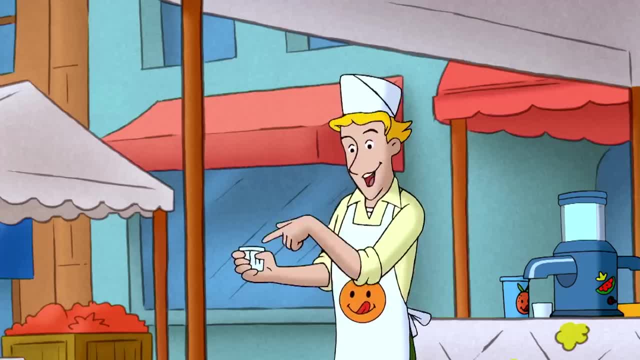 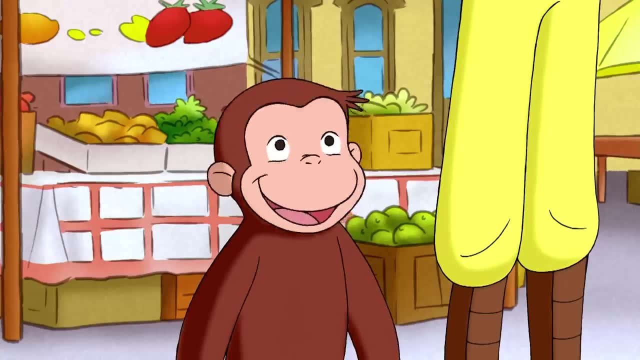 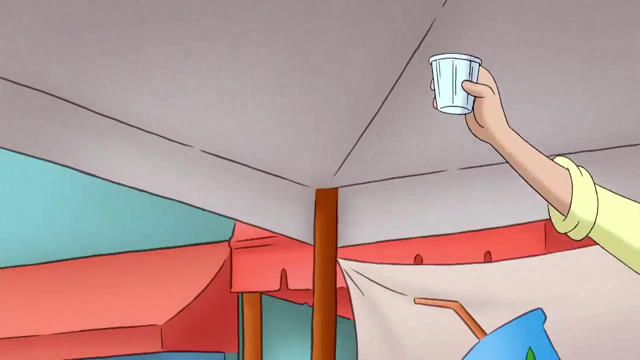 Oh, this is fantastic. Can I get the recipe? Sure, George started with your juice but added a few new ingredients: A radish- Oh, that is brilliant. A revolution in juice making To George and his delicious George juice. 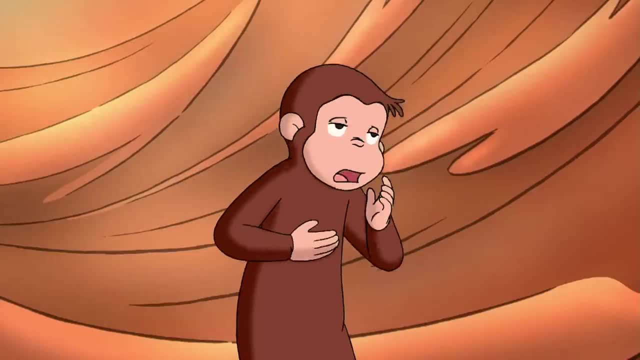 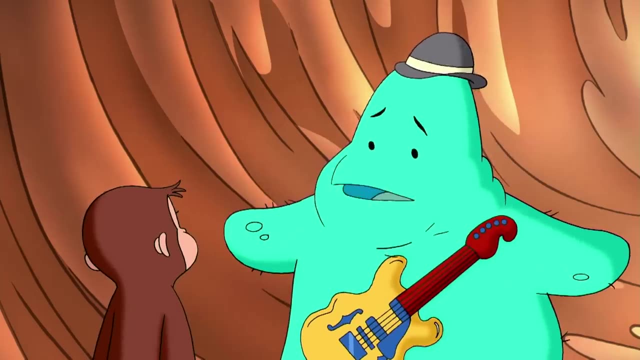 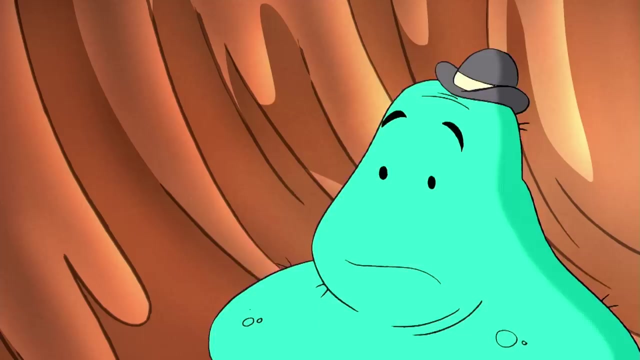 George explained that he was the owner of this body and Toots and the Germettes would have to go. Go. Why should we go? We like it here. I'm making you feel sick. Oh well, in that case I'll be on my way. I'll just get my stuff. 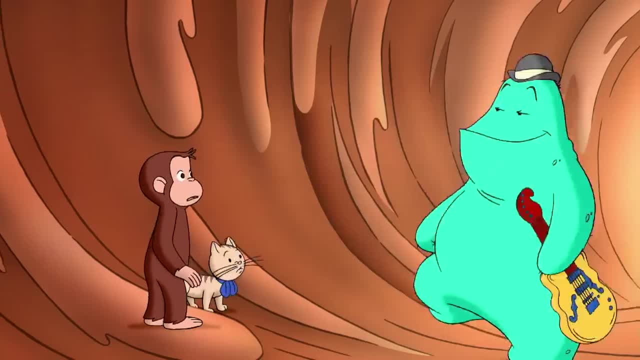 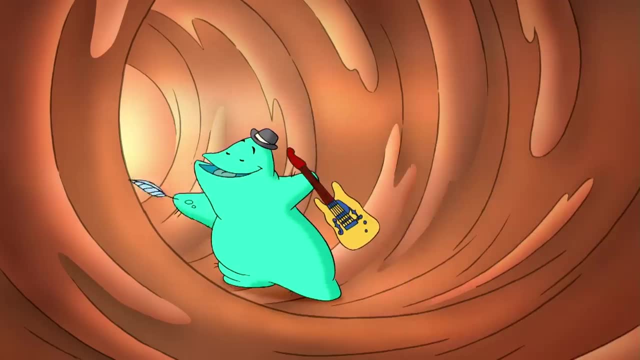 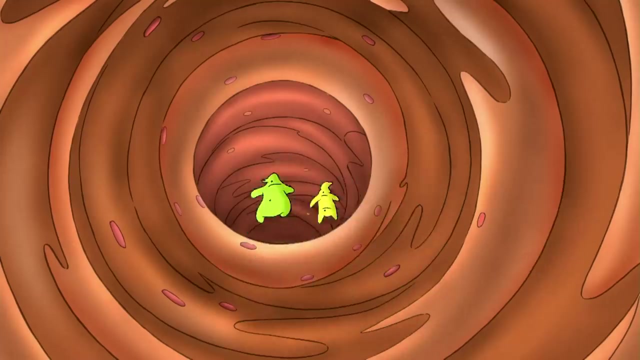 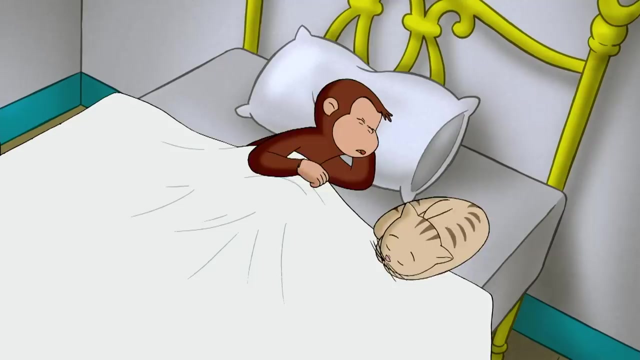 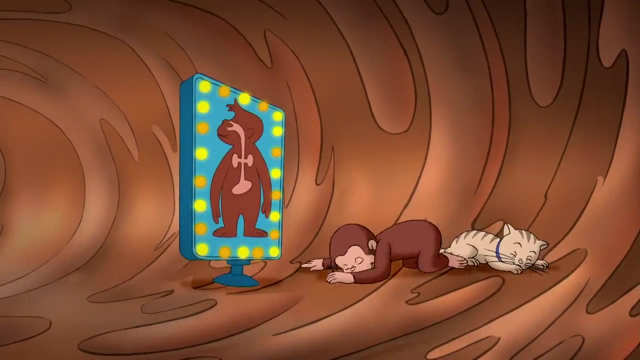 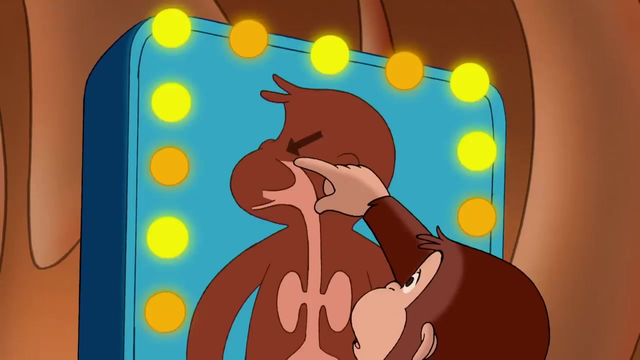 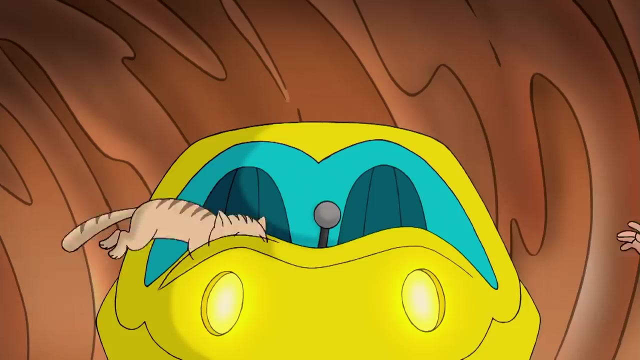 I fooled you. I'm never leaving, Hey, But you are. You got it right? George knew he wouldn't feel better until he got rid of Toots, But where did he go? The lungs: George and Yoki agreed to try his lungs first. 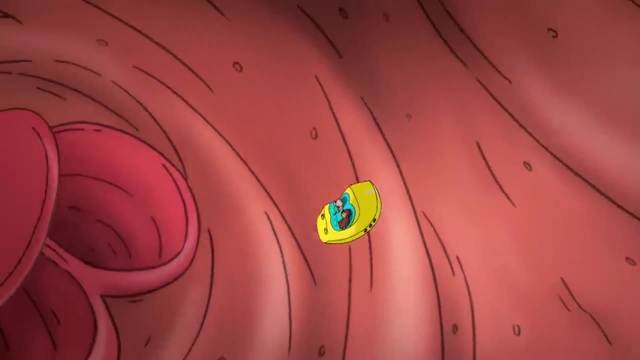 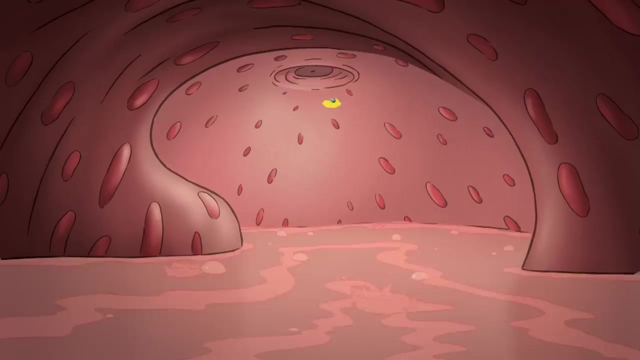 What can that mean? It looks like a good job, Right, George, don't let your new lungs be that bad. But George might have been a bit too high for him. No, not that bad. If you think that he is in a bad mood, do something about it. 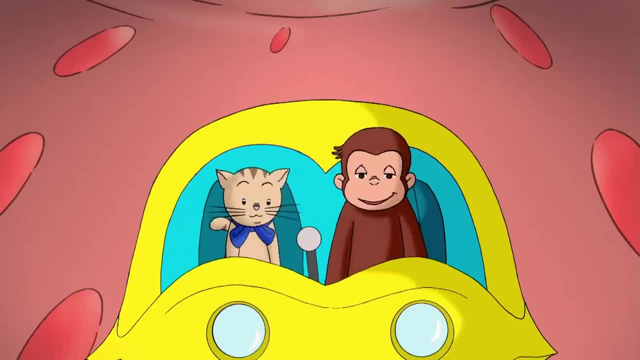 Is he still in a bad mood? Yeah, I'm just telling you, But why are you saying I'm in the wrong place? Why are you saying you're in a bad mood when you are in a bad mood? Oh, that's not what I meant. 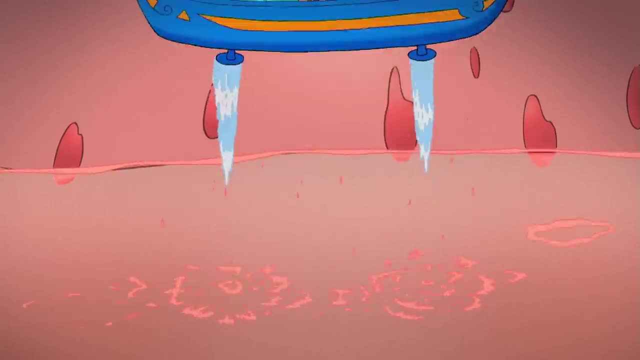 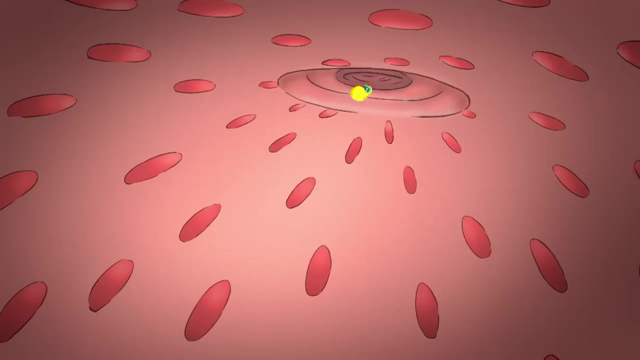 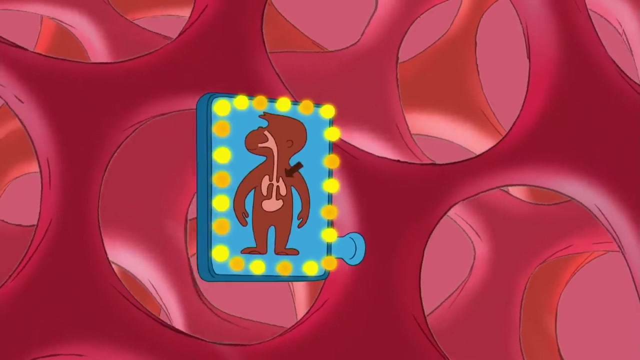 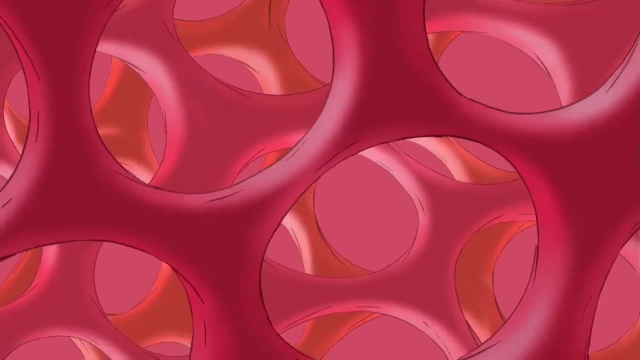 Are you crazy? No, I'm not crazy. You're not crazy. I'm crazy. Of course You got it. Oh no, Now this looked more like a lung. When the walls moved out, air came in. When the walls moved in, air rushed out. 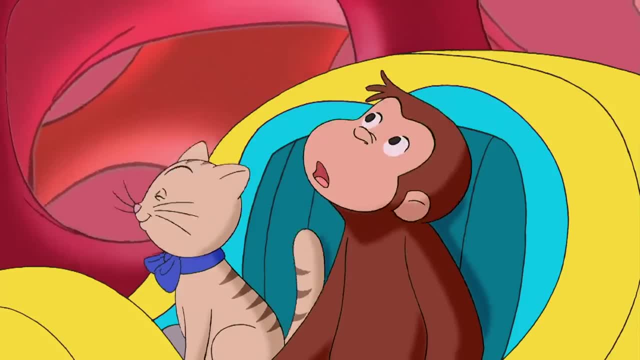 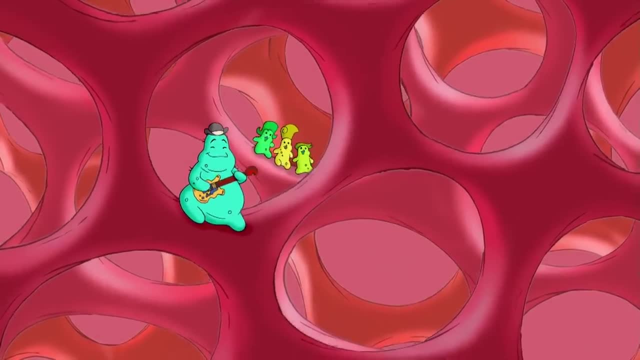 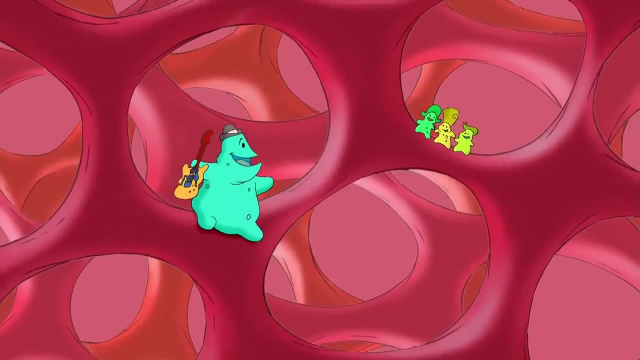 George was watching himself breathe. Well, baby, I'm in your love. Ooh, yeah, it's in your love. Ooh, yeah, in your love. That too, This was George's chance. So where should we go next? 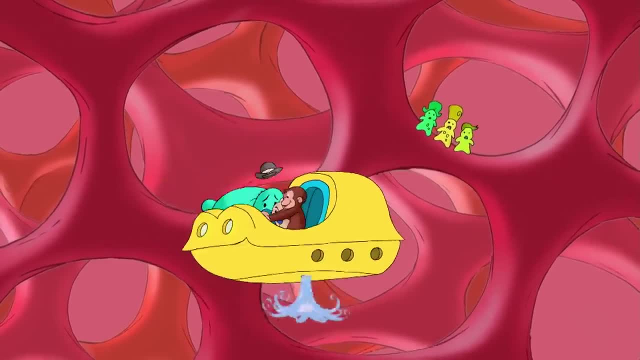 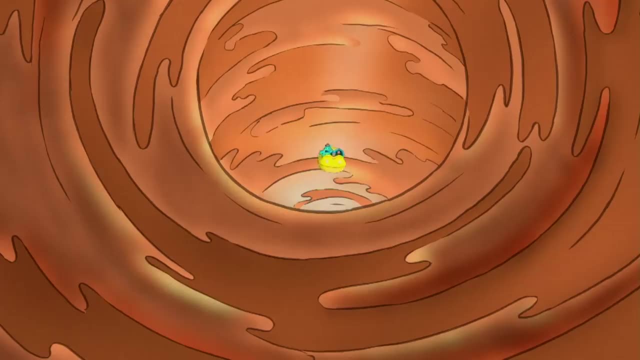